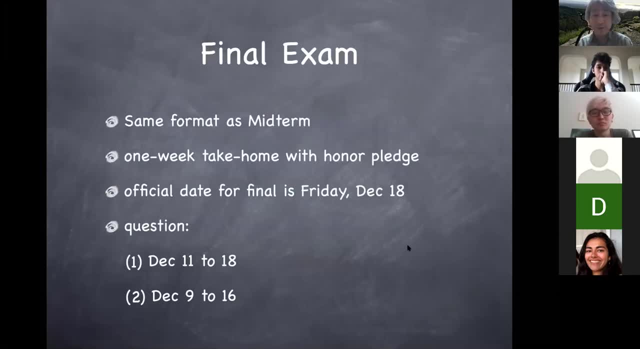 So, but before getting to this, I still have only rather few of you now, but let me post a question anyway. So the final exam will be the same format as a midterm, namely the one week take home, And I asked you to sign a honor pledge. 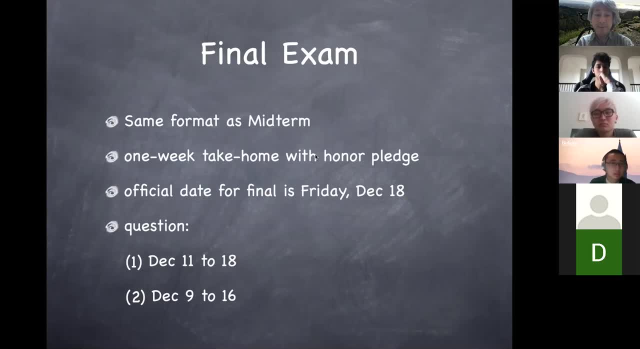 And the official date, as posted by the campus, for the final exam for this class is Friday, December 18,, as you know. So the final default option would be to have this take home exam due on December 18.. So that would actually, you know, walking backwards. I post the exam on December 11 to have a week for that. 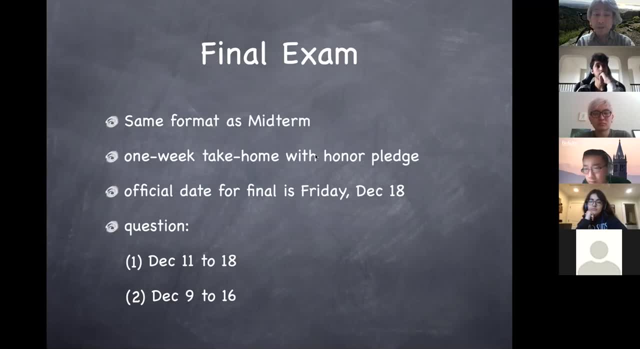 So that's one option. But talking to a few of you, some of you might actually like the idea that you can start working it in the reading week, so that that will sort of spread out the load. You don't have to sort of scramble along to work on this take home exam while you are also preparing for the other final exams. 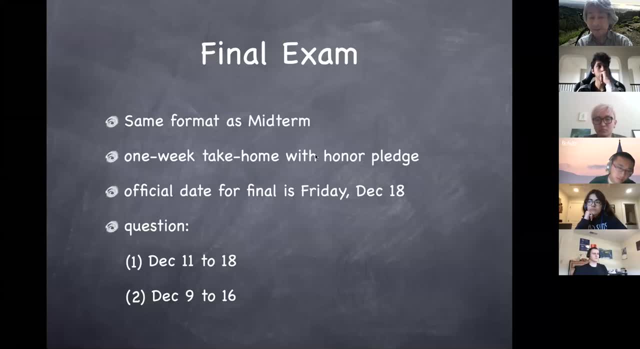 So I would like to ask you for preference, And since there are only rather few of you today, I will actually do an online poll in addition to it, But I'd like to get some preliminary idea on what you prefer. So here's the poll. 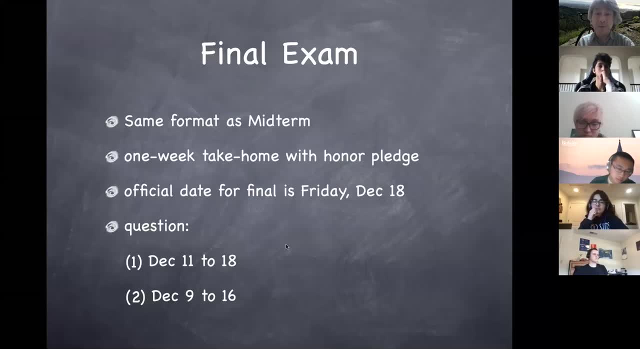 And you can click on both of them. So if you don't have any particular opinions about it, But anyway, I'd like to see your preferences on this. Do you see the poll? Okay, maybe that's about it. So at least more of you seem to prefer the default option. 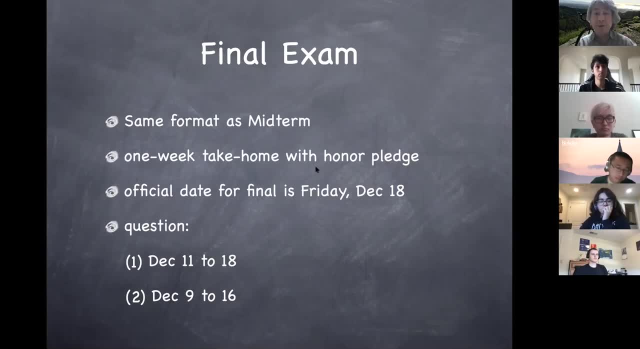 So this is the result, But you know it's close, so maybe we should do a recount. So I'm going to actually post this poll also online And I ask every one of you to actually fill that out, Okay, And hopefully there's not dead people voting at this stage, right? 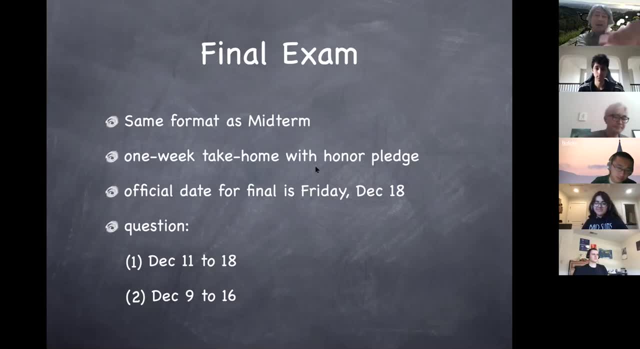 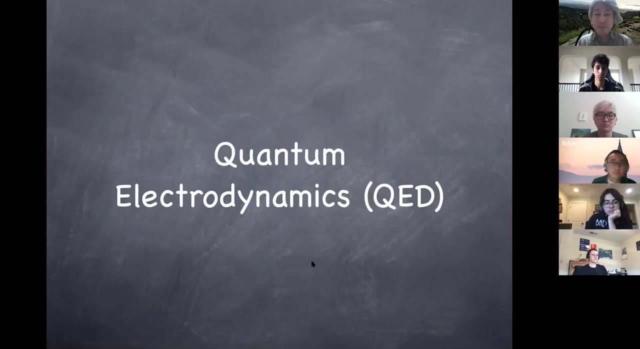 We will find out. So I actually put the deciding on schedule depending on the preference of the class, So we'll do that later on. Okay, let me get to physics. So we started talking about quantum electrodynamics, QED, Which is arguably the most successful physical theory ever in the history of physics. actually, 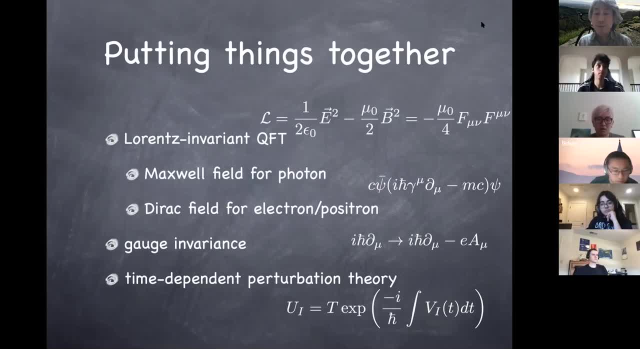 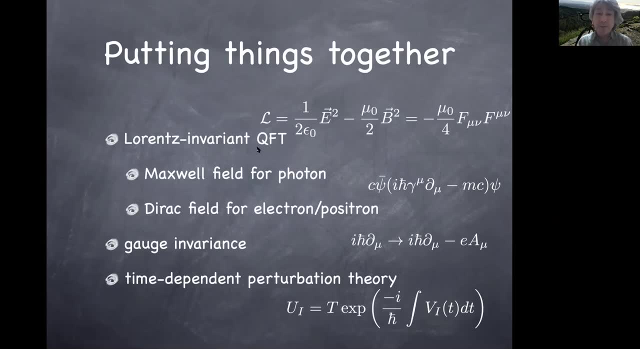 And I come back and talk about that too. So what we had to do is really just put together all the ideas we talked about in the class from the very beginning. So we are now talking about Lorentz invariant quantum field theory. So for the electromagnetic field we have this Maxwell's Lagrangian. 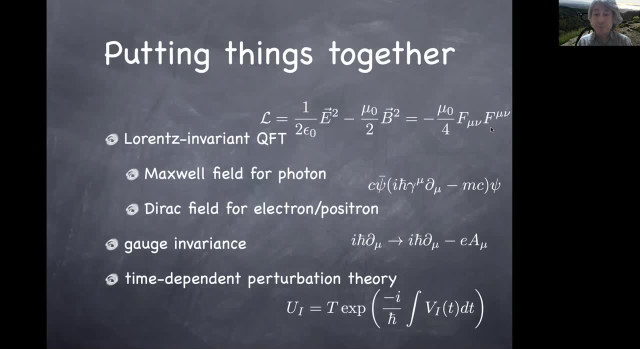 And in Lorentz invariant notation this F mu nu, F mu nu. So we have actually quantized this to get the photon out of that. We also know how to describe spin one-half particle like electron and positron, using the Dirac field. 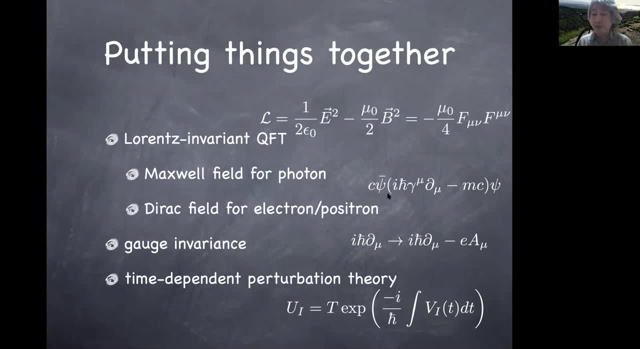 We quantized it and got four degrees of freedom. The particle will spin up and down And the antiparticle will spin up and down. So we know these fields- And both of them so far are free fields. But we also learned when we talked about the superconductivity that we need to respect: gauge invariance. 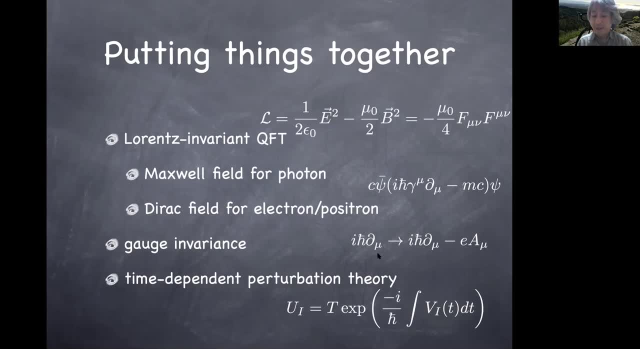 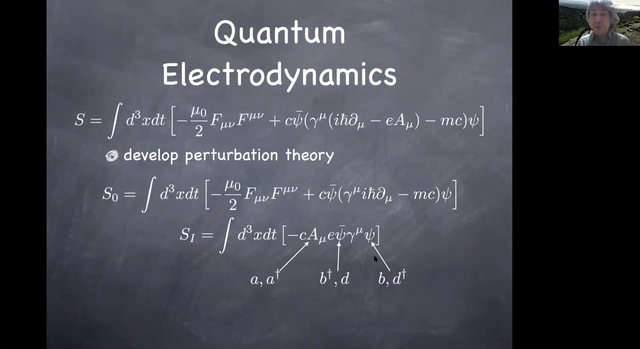 And that forces us to change all the derivatives on the charged fields, replaced by this covariant derivative which now includes this electromagnetic potential, A mu. So, at the end of the day, this is all you have to do. So, by putting together this Lagrangian for the electromagnetic field, Lagrangian for the Dirac field, 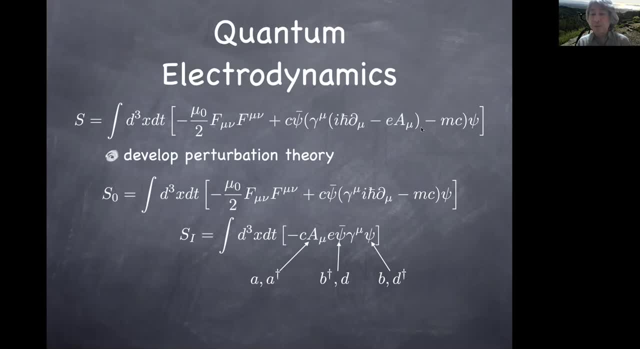 but now that this derivative is replaced by Dirac field, it's replaced by this covariant derivative, And that's it, And that's the Lagrangian of QED. So it fits on one line. And I have not seen any T-shirt actually with this action printed on it. 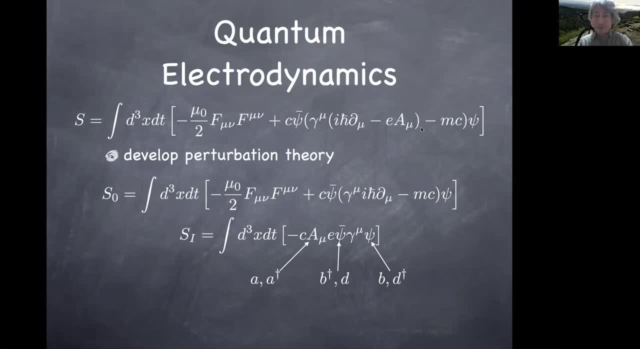 I encourage some of you to actually make those, because it's just one line equation And that is supposed to be one of the best physical theories ever, So this is actually definitely worth a T-shirt. So the idea here is that now that we have this Lagrangian 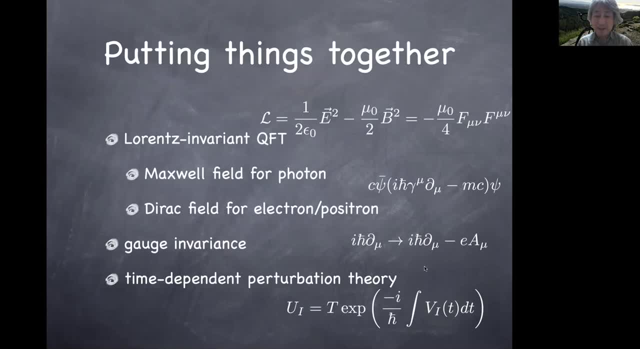 let's talk about perturbation theory, And I forgot to mention on the last slide that we use this time-dependent perturbation theory we already developed in the class And we use this to, for example, compute the weighty scattering of the photon getting scattered by an atom. 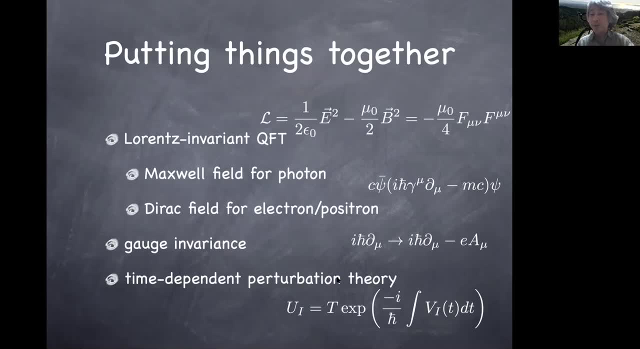 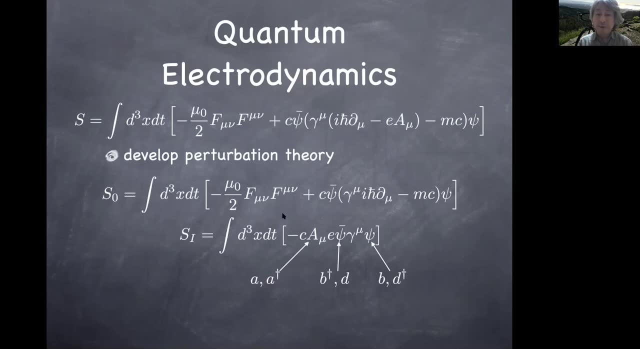 And we understood why the sky is blue, And so we just extend that idea to QED as well. So what do you do? is very simple. So we already know the free theory of the photon free theory of the electron, And the only additional term we got is when we replaced this derivative by covariant derivative. 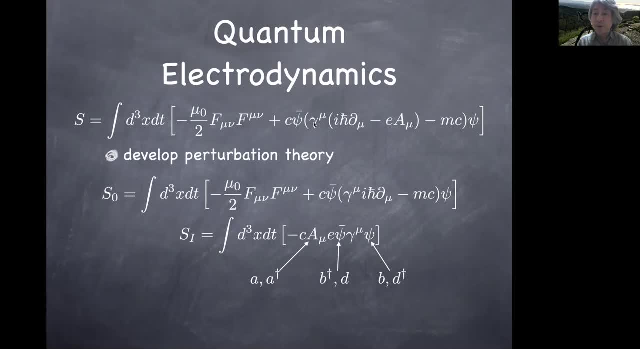 So this piece with Ea, mu coupled to psi, bar gamma, mu. psi is the only new term you have And we treat this as a small perturbation to the system And, at the end of the day, we justify this treatment of the perturbation theory a posteriori. 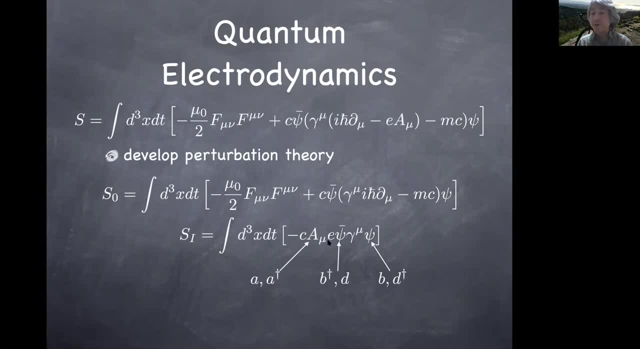 because E here turns into the fine structure constant. E squared over 4, pi, epsilon of H, bar, C, is the fine structure constant, which is known to be a small number: 1 over 137.. So the perturbation theory is the power series. expansion in alpha. 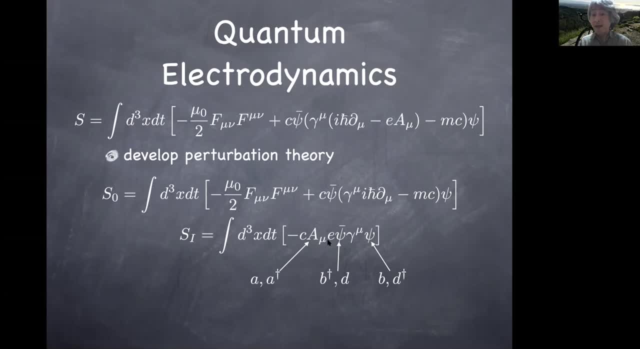 It actually more turns out to be power series, expansion in alpha over pi. it turns out So that's something like three per mil. And if you have a power series in a number in highest powers in three per mil, you know every term becomes smaller and smaller. 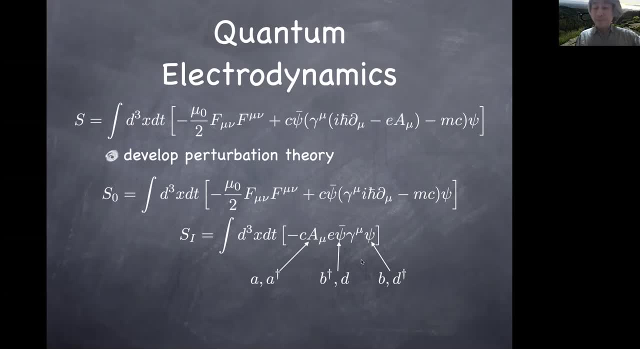 So the perturbation theory is supposed to work very well. So that's why the perturbation theory is actually justified at the end of the day, And so the quantum electrodynamics works beautifully as a result. So you are not seeing any new ideas here. 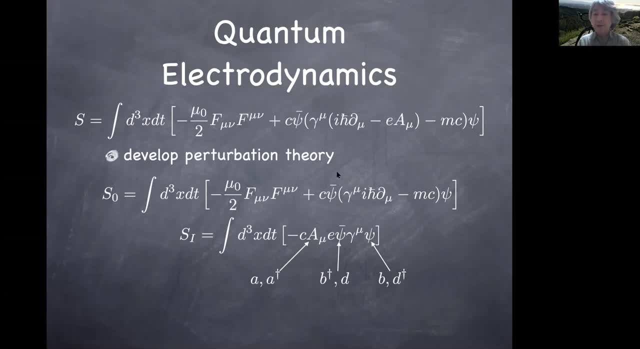 You already have understood the free theory of photon, free theory of electron. Now you have, this time, dependent perturbation theory, using this additional term in the Lagrangian, And all we need to do is to understand what this operator does. And that turns into the Feynman diagrams. 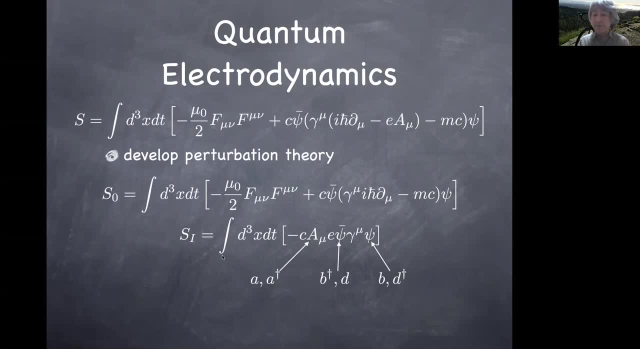 as we started to talk about very briefly before the Thanksgiving break. So, anyway, that's where we're heading today, And we try to develop all the machineries of the computing Feynman diagrams using this idea of time dependent perturbation theory, using this operator as a perturbation to the system. 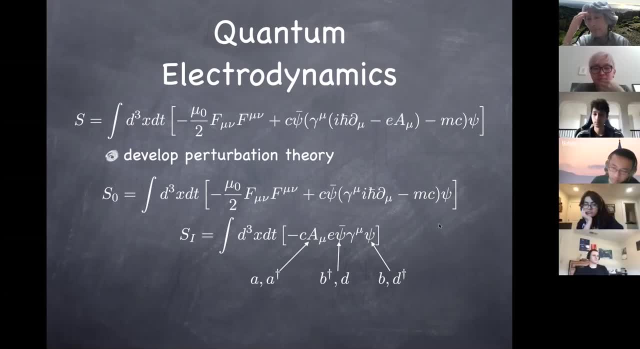 So any questions so far. Where are we heading to? OK, All right. So one thing we need to do is, by staring at this operator we are perturbating the theory with. we know that a new field, the vector potential, is written in terms of the creation and annihilation operator of the photon. 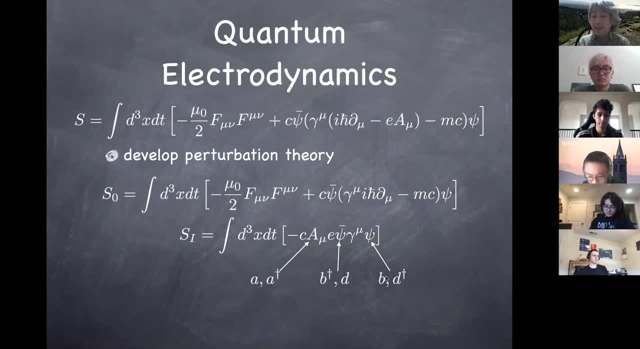 And psi field, a Dirac field. it contains annihilation operator for the particle, like electron in this case, and creation operator for the antiparticle, namely positron. So psi contains B and D dagger. So here I avoided the clash of notation. 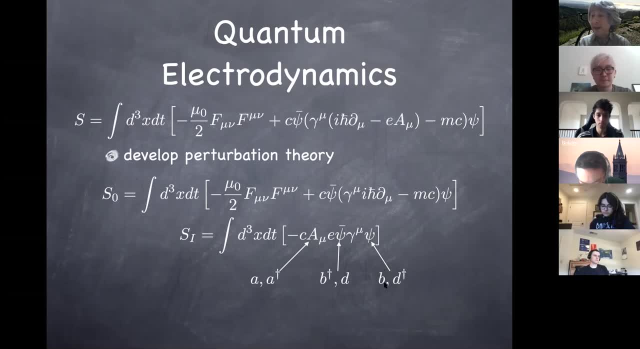 So annihilation operator is now labeled B instead of A to avoid clash of notation with the annihilation operator of the photon, which I still call A. So B is the annihilation operator for the electron. D is the annihilation operator for the positron. 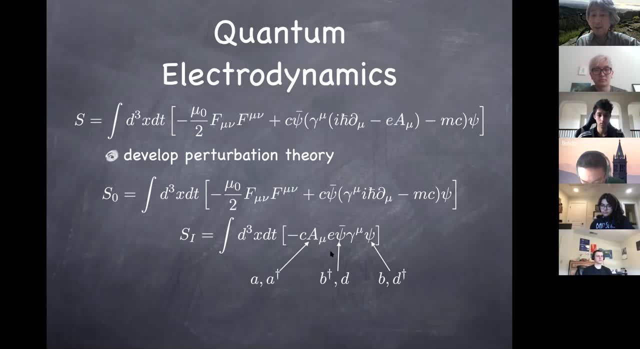 Psi contains B and D dagger And psi bar is a psi dagger gamma naught. So that contains B dagger, creation operator of the electron, and D annihilation operator of the positron. So knowing the operator content of this perturbation. 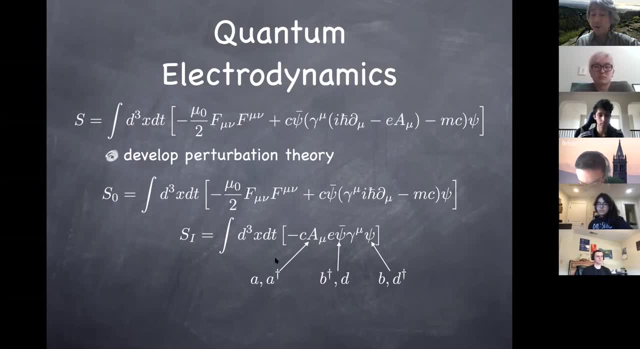 we can figure out what this operator actually does when we develop perturbation theory. So that's the idea how we'd like to proceed. So that's where we define this perturbation: Hamiltonian VI in the interaction picture And as you have seen before, 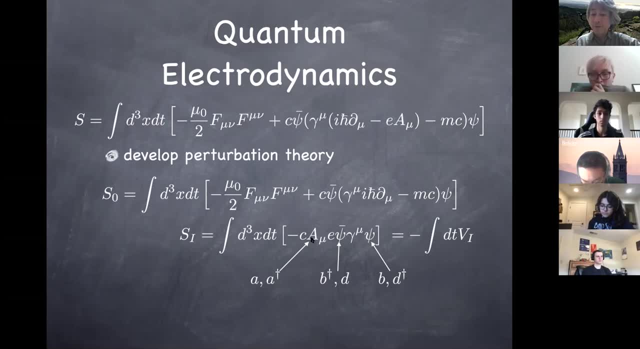 going to the interaction picture is simply letting all of these operators evolve according to the free Hamiltonian, So namely that psi, B, D, dagger, all follow the evolution equation of the free theory. So we understand them cool by now. right, And so we know everything about A: A dagger, B dagger, D, B, D, dagger. 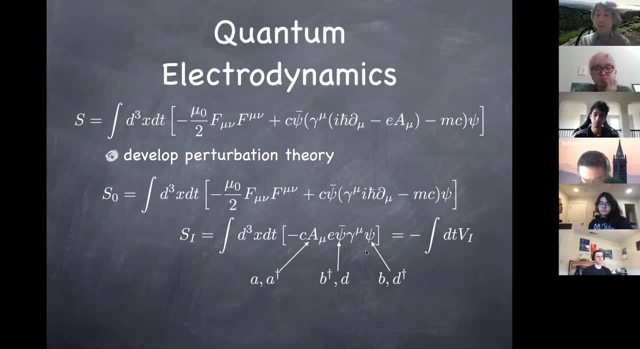 coming into this perturbation Hamiltonian in interaction picture. So all we have to do then is to put them into the matrix elements to compute some process. So we started actually doing this, And the time evolution operator is a time-ordered product of the exponential of this perturbation Hamiltonian VI. 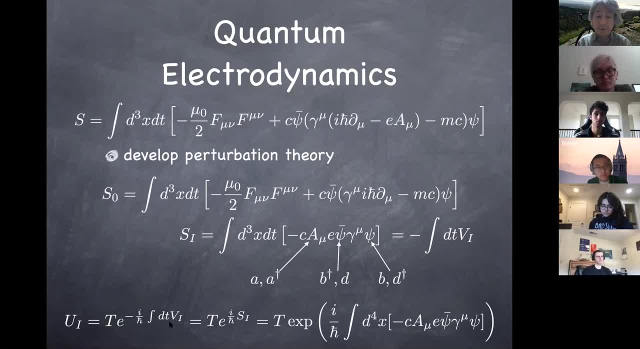 We also talked about this in the time-dependent perturbation theory before, And what you notice here is that when you do this time integral of the perturbation Hamiltonian, perturbation Hamiltonian is this action without time integral with a negative sign. So what this amounts to is basically just to gain this new term. 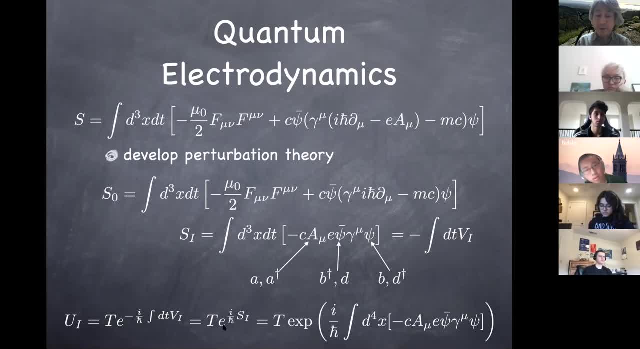 in the action SI into this time-ordered exponential. So hence this is the expression. we are looking at: Time-ordered product of exponential, of four-dimensional integral of this operator. And now everything looks manifestly Lorentz invariant. So in this term, in the Lagrangian density, 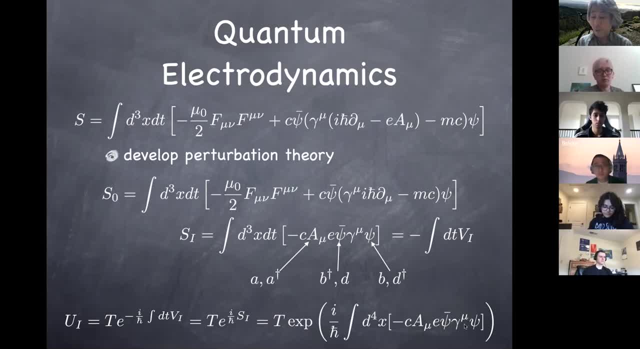 I have psi bar gamma, mu, psi. I have Lorentz index, mu, which is contracted with the Lorentz index downstairs for the vector potential, a mu. So upon contraction this is now a Lorentz scalar. It's invariant under Lorentz transformation. 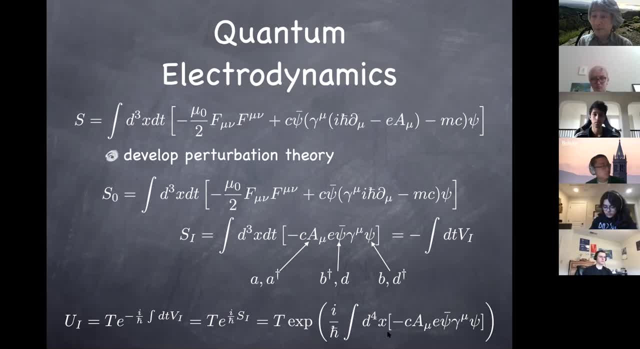 It's integrated over the full space-time- three-dimensional space in one-dimensional time. So this integration volume is Lorentz invariant. So now every quantity we are looking at here is Lorentz invariant. So this perturbation theory is now defined in a manifestly 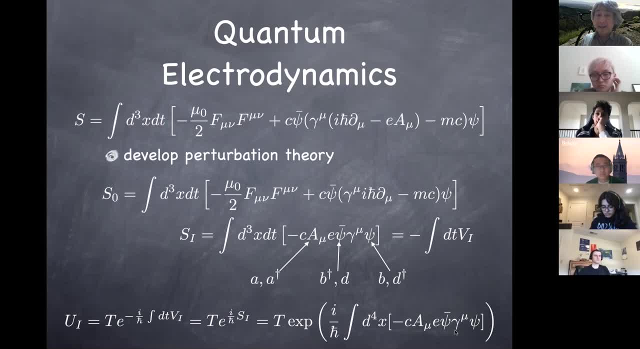 Lorentz invariant function, And that's exactly what we wanted. So we can now start doing some computations in quantum electrodynamics, QED, where every stage of the calculation is now manifestly Lorentz invariant. And so that you wouldn't lose track. 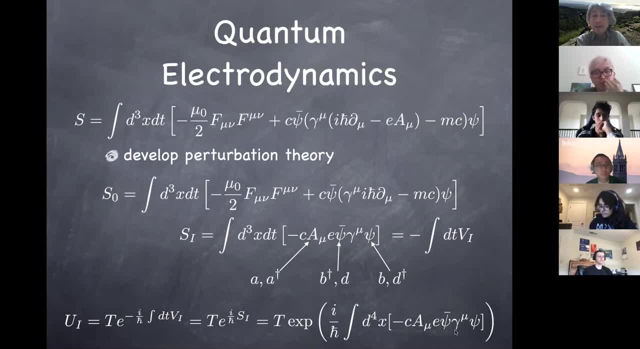 of the full Lorentz invariance of the theory. So that's how we can actually develop perturbation theory. That's a great advantage of using this time-dependent perturbation theory, which was started by the Richard Feynman. that's why we talk about Feynman diagrams. 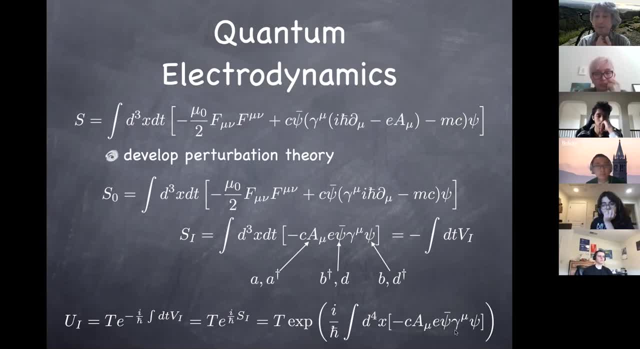 and Feynman rules, But of course there have been other formulations. We'll come back and talk about that, hopefully on Friday, But anyway, any questions about this slide? Well, I think you get a better idea after seeing it. So now that we know the operator, 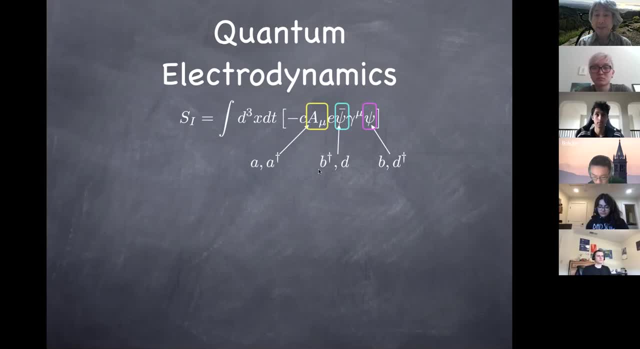 and what is made of creation and addition operators. and because each field contains basically two kinds of operators, either annihilation operator or creation operator, each one has two pieces in it. Two times two times two, there are eight pieces in this operator. 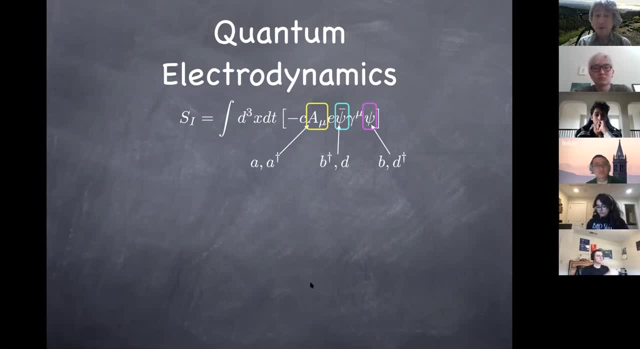 And we can see what it does- And we already talked briefly about this last time- And because of this drag notation, that initial state tends to be on the right, final state tends to be on the left, as a bra initial state as a ket. 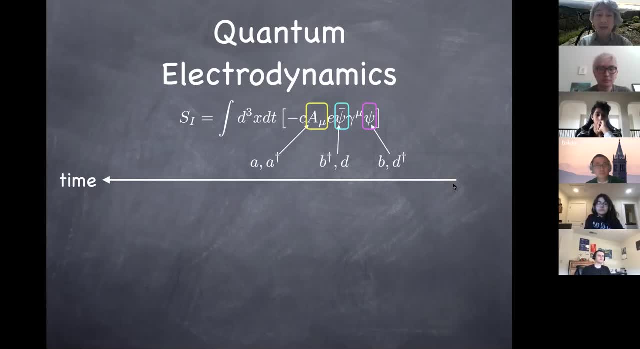 final state: as a bra, we better write time flowing to the left, like in Arabic and Hebrew, which is not I'm familiar with. but this is the ordering which probably makes the best sense when you compare the equation to the diagrams. So when you actually have this operator psi. 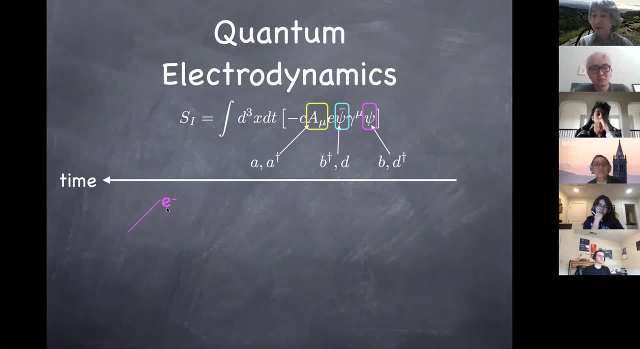 you can start with a ket that has an electron in it, and then psi would annihilate that. So now the electron is gone, But using this psi bar, which has the creation operator B dagger in it, you can create electron, but presumably in a different momentum state. 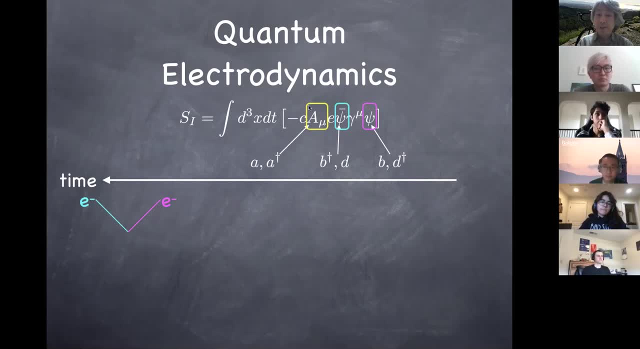 And at the same time you also have this operator in yellow which can create a photon. So one thing this operator can do is to take an electron and turn that into one electron and one photon. So that's what this operator can do. 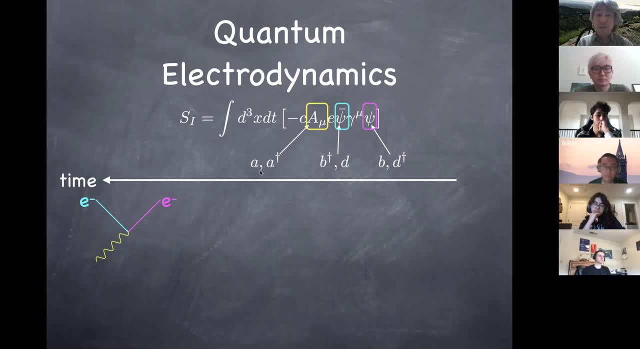 But because a mu also contains an annihilation operator for the photon instead of creation operator we used over here, it can also give you this process that you start with the initial state with one electron and one photon. an electron absorbs a photon and turn into a single electron. 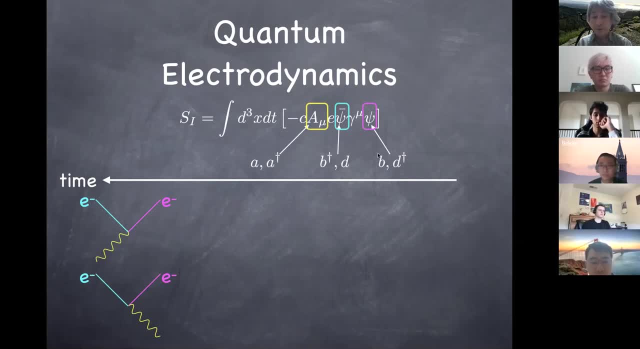 That's yet another thing this operator can do. So this is two things, But, as I said, there are eight possible things this operator can do, So let me go one by one. Another thing this operator can do is to first use this psi. 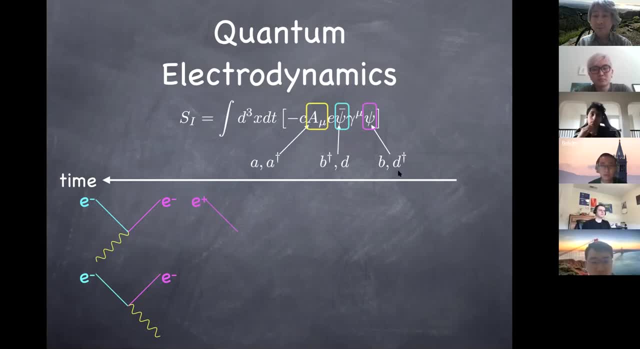 to create a positron. So positron didn't exist as a part of the initial ket, but positron can exist as part of the final state bra. But of course we also have psi bar that has D in it, which is the annihilation operator of positron. 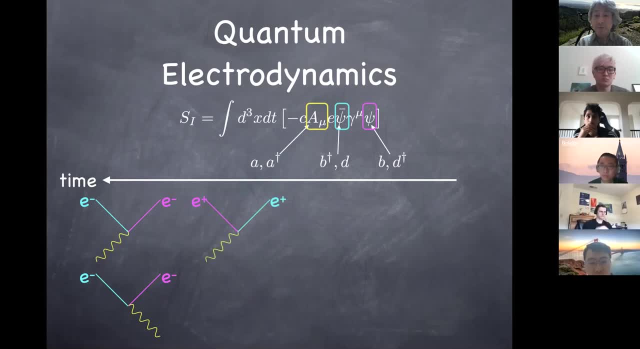 And then a mu can create a photon. So that's a very similar process as we described for the case of electron, except that the role of psi and psi bar interchanged. So psi field creates positron, Psi bar field annihilates a positron. 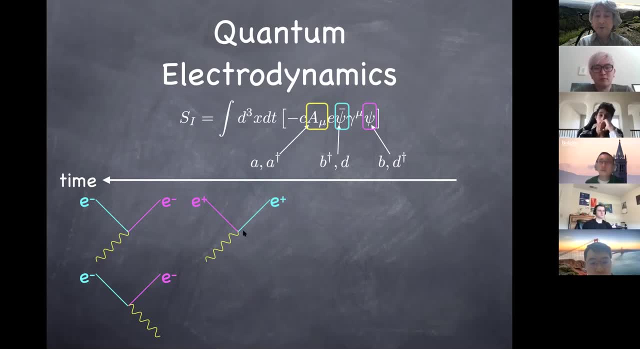 But nonetheless the process looks similar. Positron ends up emitting a photon, So that's the same thing as what we stare at here for the electron, And obviously I can also go to the lower row, namely that the positron is created by this magenta psi. 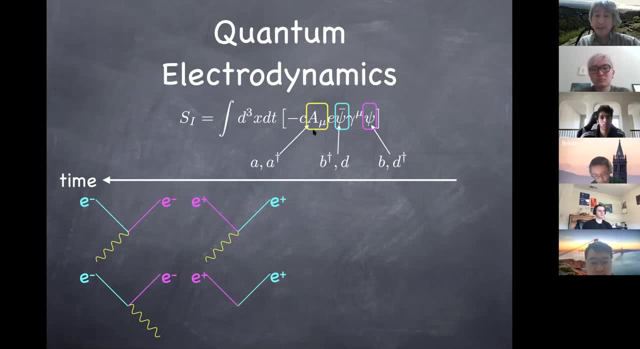 Positron is annihilated by the psi on psi And a mu creates- sorry, absorbs- a photon. So positron now absorbs a photon and becomes a single positron. So that's yet another thing this operator can do. So now we have four. 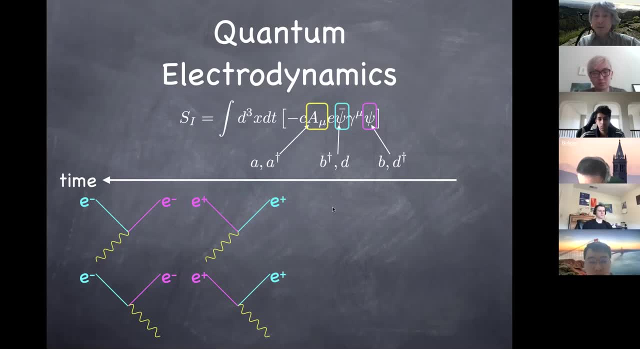 and there are four more to go right. So another thing this operator can do is to use this magenta psi to annihilate an electron using this B operator. But using this psi on psi bar I can also annihilate a positron using the operator D. 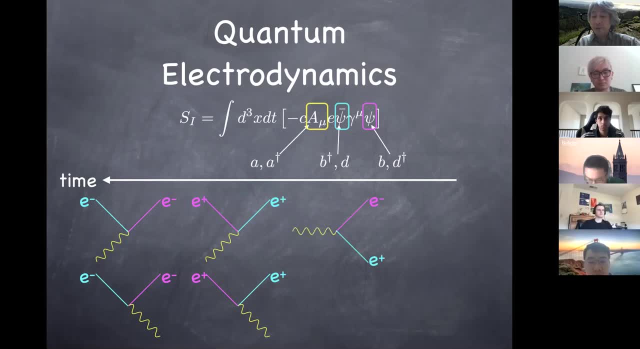 and then create a photon with a mu. So this is a new process which we haven't seen before, Namely an electron and positron can literally annihilate into a photon. So in the first four processes we talked about, total number of electron doesn't change. 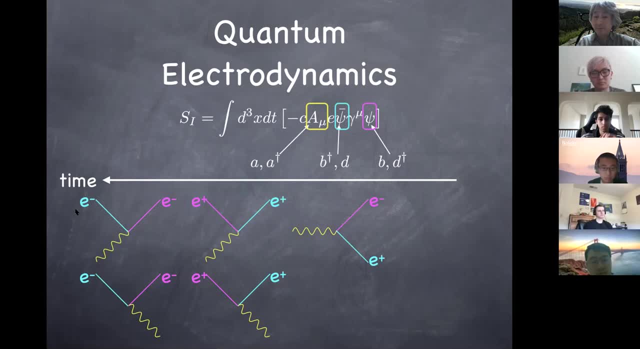 We start with one electron, you end up with one electron. Or you start with one positron, you end up with one positron. So number of matter particles doesn't change. But here you have a new possibility: Number of matter particles can change. 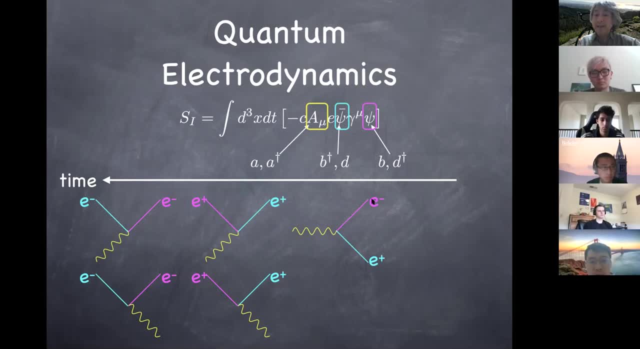 because a particle and antiparticle can annihilate with each other. A number operator that is conserved, which we talked about before, is the number of electrons minus number of positrons. that is still conserved because the number of electrons is one. 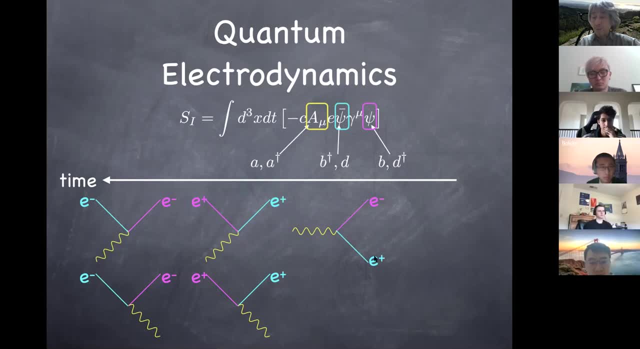 number of positron is one. one minus one is zero in the initial state, and so it is in the final state. zero minus zero is zero. So that's the conservation law we talked about. What is conserved is only the difference between the number of electrons. 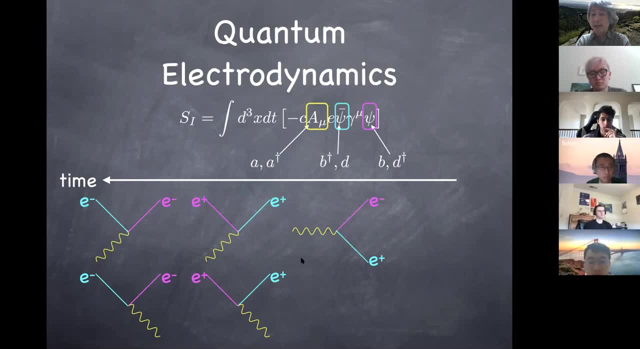 and number of positrons, which is called the electron number. An electron number times charge. E, of course, is the electric charge of the system, So that is obviously conserved. But what we are seeing here is that electron number and positron number. 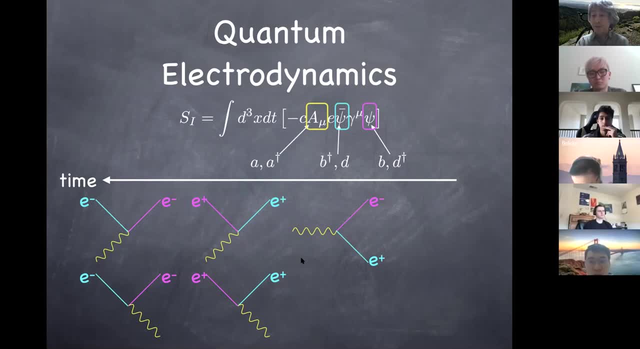 individually is not conserved because they can annihilate. So that's the first time we observe something like this And we talk about a concrete process where this does happen later on. So this is five now, And the next thing we have to do 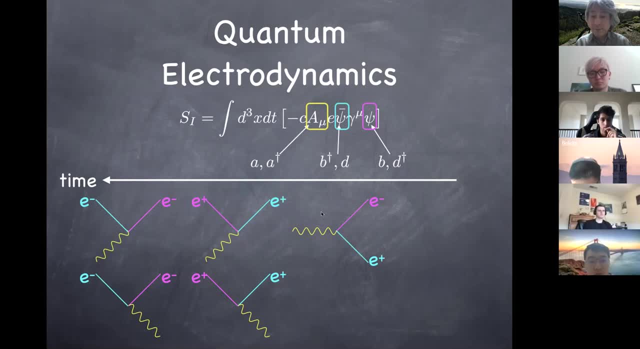 by going to the lower row, is that instead of using creation operator for the photon, we can also use the annihilation operator for the photon, which looks kind of bizarre. Electron, positron and photon come together and they all disappear And you may complain that. 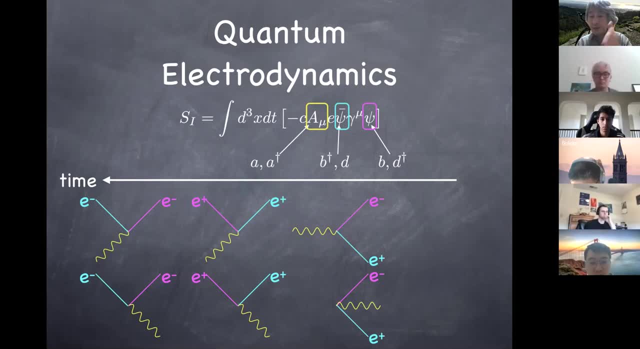 well, this doesn't seem to conserve energy, because you started out with the finite energy. two mc squared of electron and positron, together with the energy of the photon, doesn't seem to be conserved. But, as we have learned in time-dependent perturbation theory, 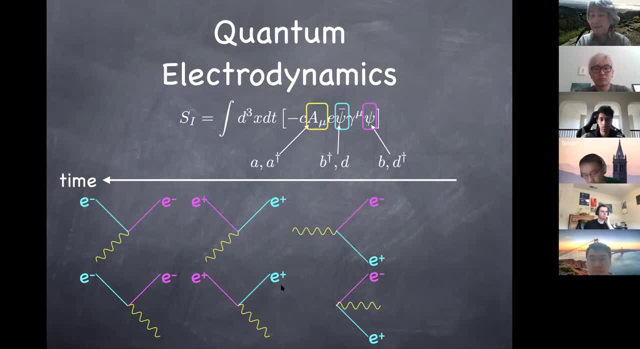 you can violate energy conservation temporarily as an intermediate state in perturbation theory, as long as the real initial state and real final state have same energy. So we make sure of that. later on You will see how that would come about, But temporarily you can have a process like this: 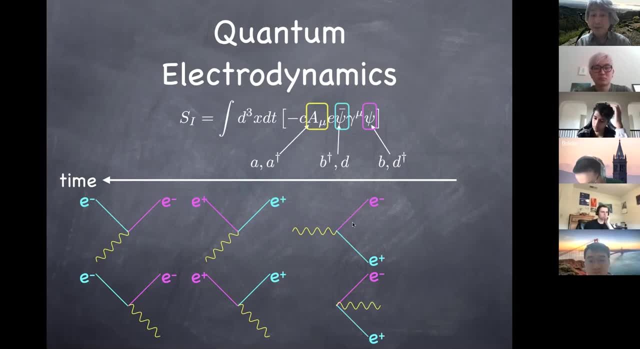 And in fact none of the processes here actually conserve energy momentum. Single electron can never emit a photon, Because if you are in the west frame of this, electron emitting a photon would produce a kick. namely, there is a momentum To conserve momentum. 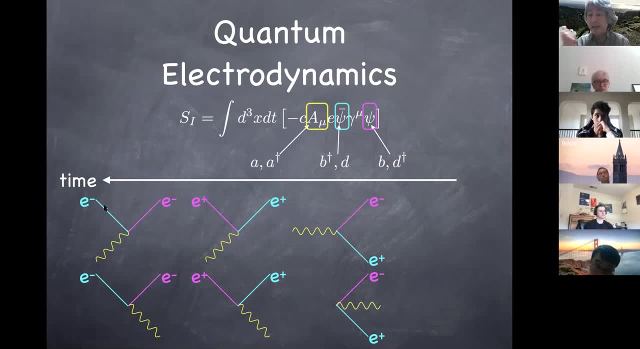 this electron would be kicked backwards with a finite momentum action-reaction going back to Newton. Then this electron has a higher energy than the original electron up west. So the final state would have higher energy than the initial state. So even this process. 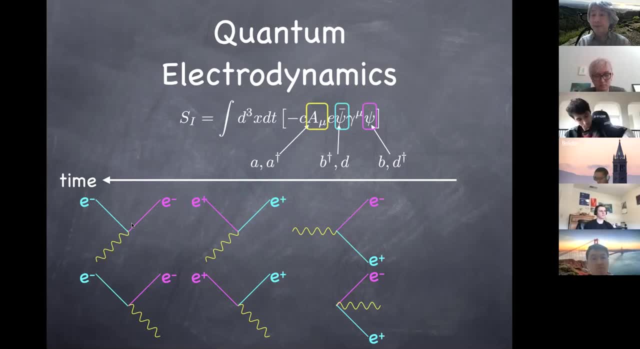 which looks kind of familiar to us but doesn't happen standalone anyway. So none of these diagrams are standalone. You have to use multiple of these processes to come up with a process that conserves energy and momentum anyway. So this sixth diagram: what this operator does. 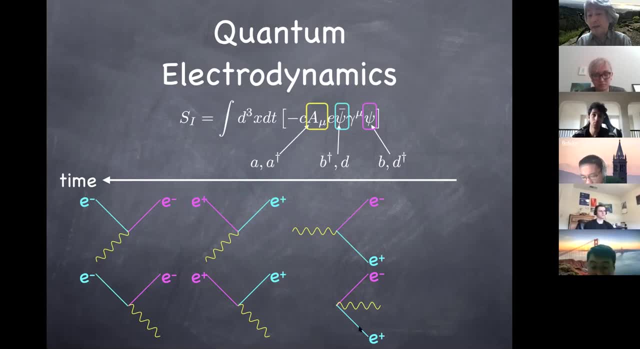 looks the most weird one so far, but at least it is on equal footing than the rest. None of them conserves energy and momentum by its own, But if you combine several of these, you can come up with a process where energy and momentum is conserved. 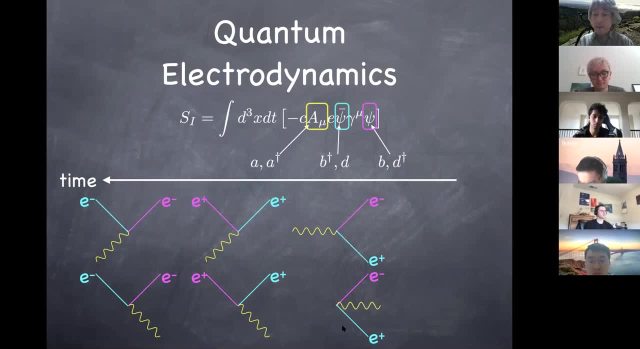 and a process can happen at the end of the day, But anyway. so right now I'm just exhausting all logical possibilities coming from this operator And I just finished six. so there's two more to go And the last two. I think it's already obvious to you. 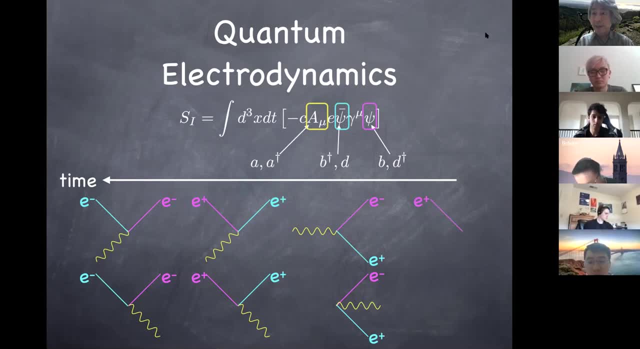 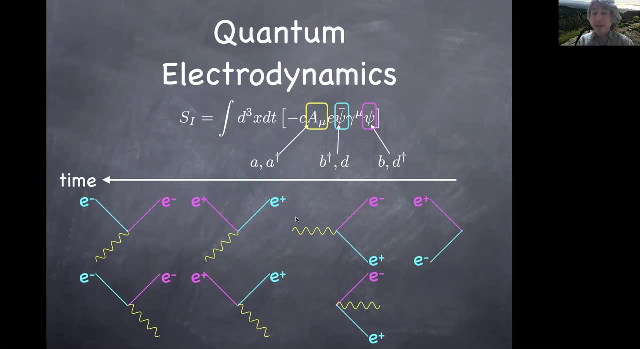 So using this magento operator, I create a positron. Using the cyan operator, I can create an electron, Together with creating a photon. that's sort of the reverse of the last process we just talked about And this last amu operator. 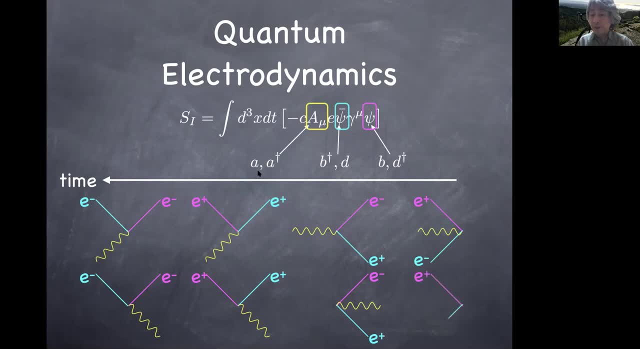 can also annihilate a photon, So what it does is already obvious to you. that will be this process. So this exhaust, this energy and this momentum are all eight possibilities of what this operator can do And, as I emphasized already, none of them actually conserves. 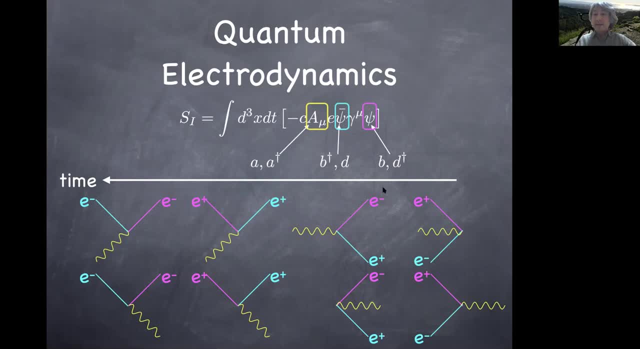 energy and momentum by its own. So I have to use these processes at least multiple times to come up with a physical process that can happen, which fully conserves energy and momentum, And we'll get to that in a moment. So this is the beginning of this idea. 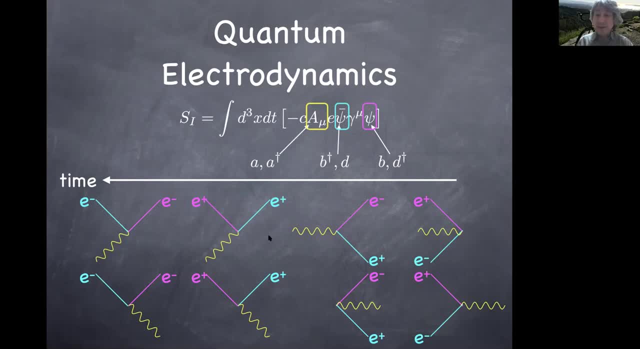 called the Feynman rules, And any of these things are called vertices because three lines come together to a point, like a vertex of a polygon. So these things are called vertices And we now have these eight possible things these vertices can do. 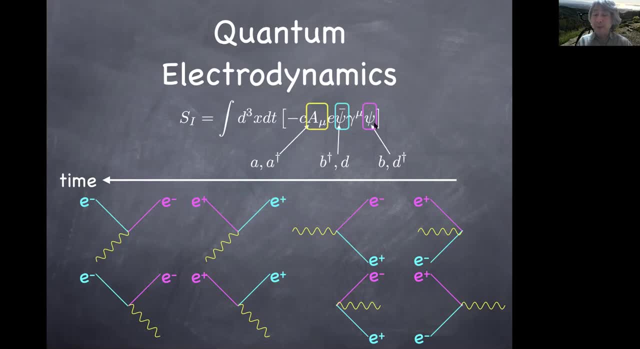 And to keep track of which one corresponds to psi operator and which one corresponds to psi bar operator. there's a convention to do all arrows for it. So when you have electron that gets annihilated by this magento operator, electron was in the initial ket. 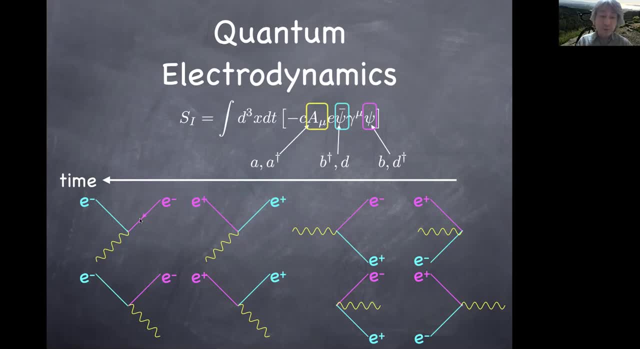 which is now gone. So that's why I draw this direction of the arrow to represent that. And this psi bar would create an electron that didn't exist, So that would go into the final state electron. So I draw this arrow over here to indicate that. 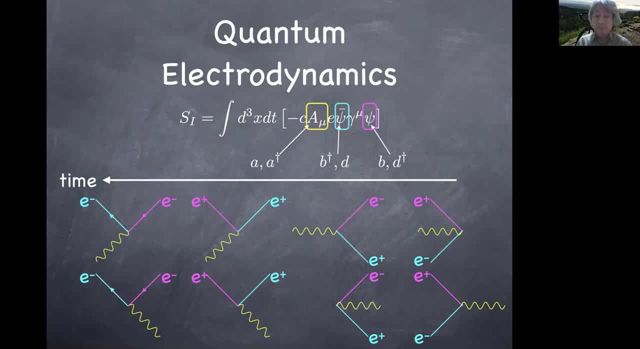 So I would do the same thing for the bottom row. But when you go to the positron it's a little weird, because what this magento operator of psi does is to create a positron. So I draw the arrow the opposite direction to indicate that creation. 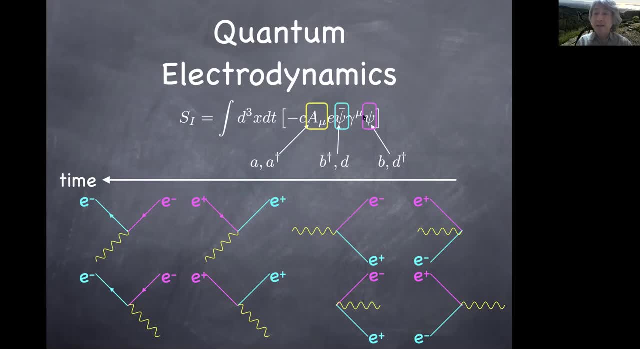 of the positron happened by this psi operator, not psi bar operator. So, instead of the initial state positron, which is electron, was annihilated by the magento psi, but this positron is annihilated by this psi and psi bar, again to indicate that this is done. 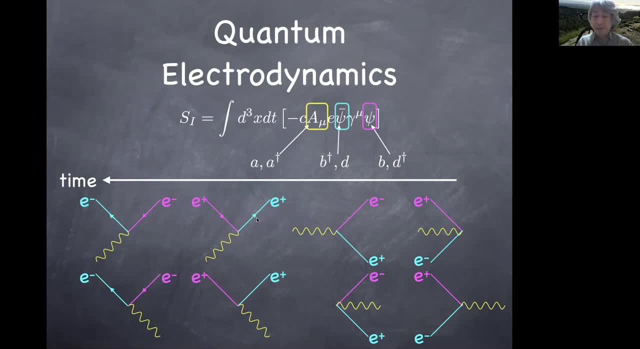 by psi bar instead of psi. I draw the arrow backwards. I do the same thing for the bottom row, And this is where some of you have heard this idea- I think it was Wendy- that antiparticle goes backward in time. Time is flowing to the left. 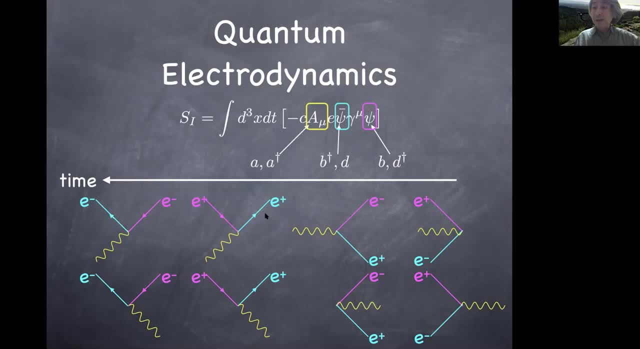 but I have drawn the arrows going to the right. So it seems as if the antiparticle positron is moving backwards in time, And obviously nothing can go backwards in time. We can never go back to kill your grandma before you were born. 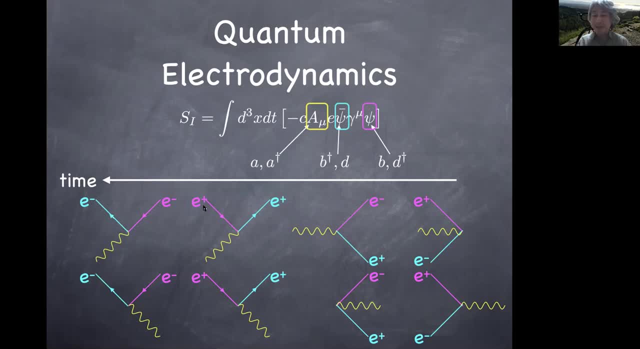 and that would really screw up laws of physics. That's the idea of causality, And back to the future shouldn't happen. So that's not something we are talking about here, But this arrow is meant to be a good way of keeping track of. 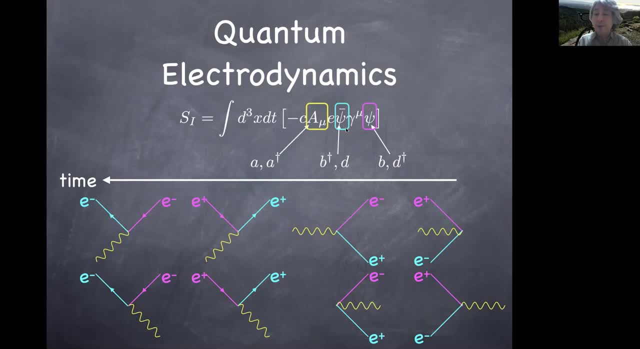 what these individual operators do. It's not meant to be that antiparticle is going backwards in time, But keeping track of these arrows I can keep track of the flow of the electron number I mentioned earlier. So electron has electron number one. 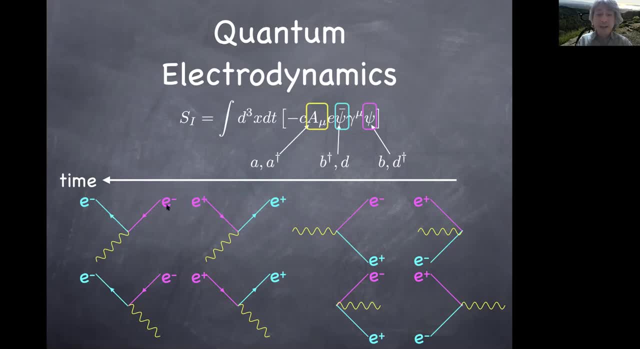 And that is the flow of the electron number. So electron number one is flowing forward in time. Positron has electron number negative one. So this number flowing backwards in time, as depicted in this picture, is meant to tell you that this is actually an antiparticle. 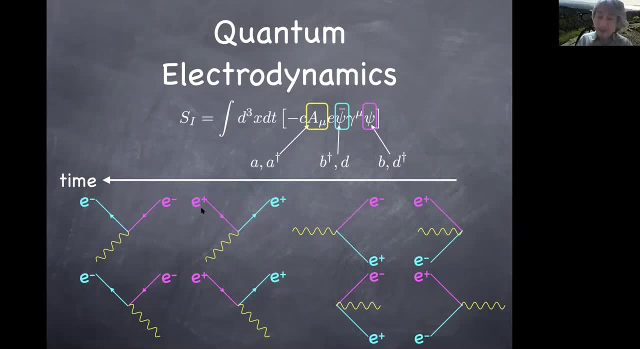 with electron number negative one moving forward in time. So instead of antiparticle going backwards in time, this is meant to be going forward in time. It's just that this backward arrow tells you that we are talking about the antiparticle, So this arrow can confuse people. 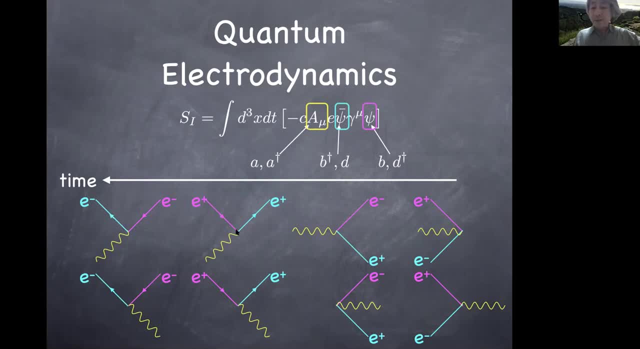 But all it is meant to convey is that backward arrow means it's antiparticle, while the forward arrow means a particle. So that's the only meaning of these arrows. So don't read too much into it. And some books, even some textbooks, 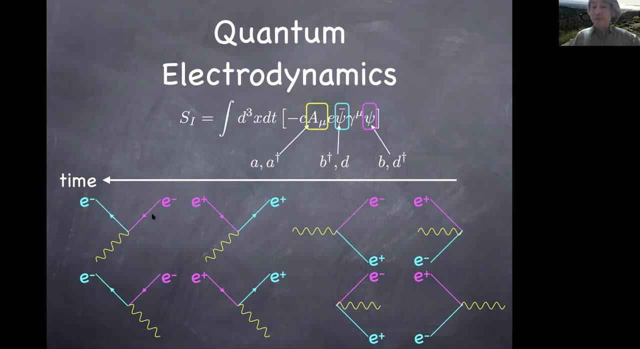 they don't say that backward arrow talks about antiparticle and backward arrow talks about particles. So we keep following this convention. And now you see why this convention is useful, Because backward arrow talks about antiparticle and forward arrow talks about particles. 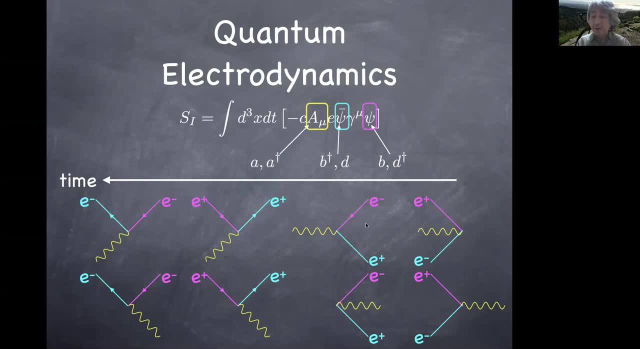 So we keep following this convention. And now you see why this convention is useful, Because when you talk about this process, you have an electron by psi-magento field- that's forward in time- And the cyan positron that is now the antiparticle. 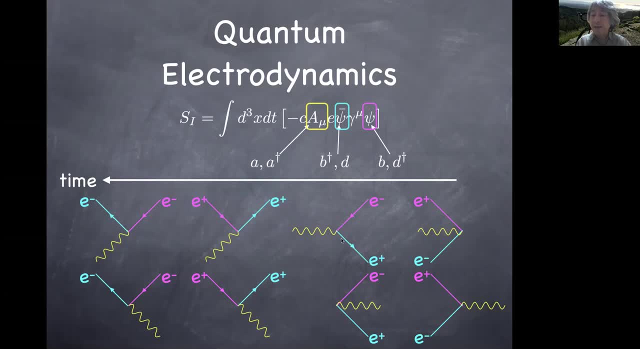 so the arrow goes backwards. So that means you can always consistently look at the flow of the arrows to understand this process. And same here, And same there And same there For every vertex. the arrows keep flowing If something comes in. 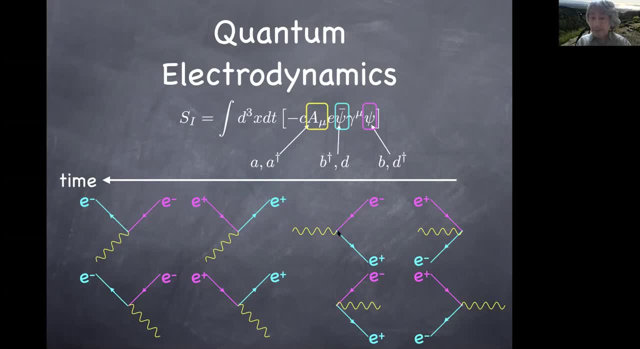 something goes out. If something comes in, something goes out. And again, the convention is that the arrow goes backwards in time. That refers to antiparticle. So once you actually look at this picture you can tell even without the labels. 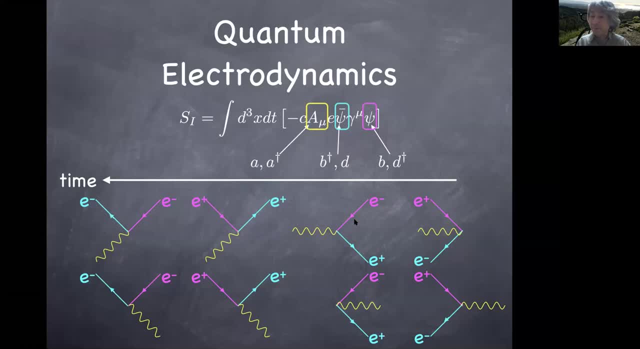 of E minus E plus in it. this magenta line is forward in time, So you can tell this is supposed to be electron. This cyan line has arrow backwards in time, So you can tell this is a positron, This is an electron. 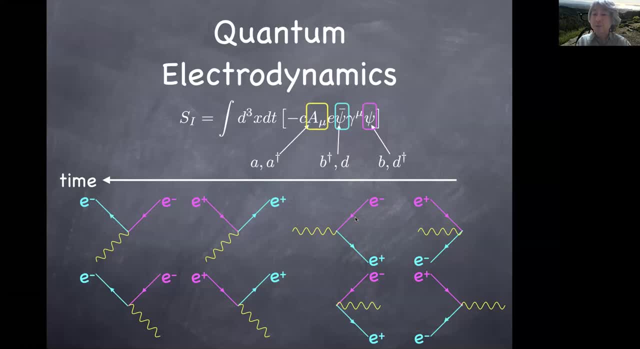 Positron annihilating into a photon. So that's the reason why we use these arrows. So they are just meant to be a way of keeping track of which line is particle, which line is the antiparticle, And you make sure that. 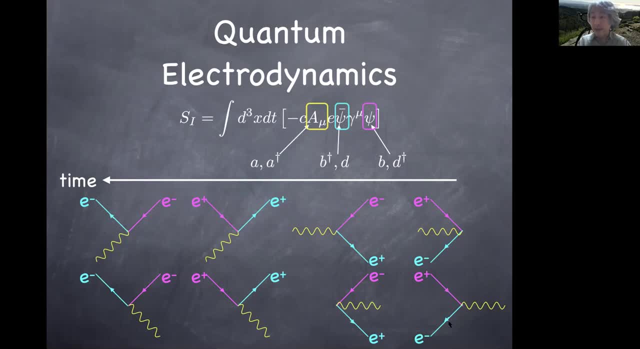 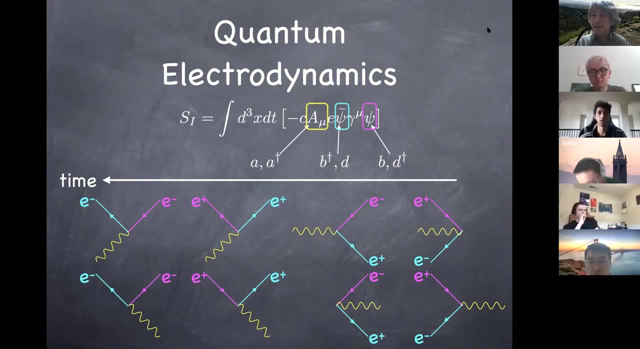 the arrows keep flowing consistently throughout the diagram And that's the purpose of these arrows. Okay, let me stop here to see if there are any questions. Is there any need for the arrows if we explicitly label the particles, as we've done here? 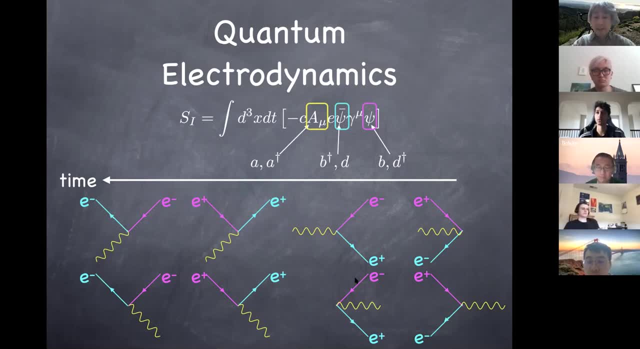 Or is it the case in general that we don't actually label the particles? Yeah, that's an excellent question, And you actually see later that trying to label each line turns out to be rather inconvenient thing to do, And you'll see why that has to do. 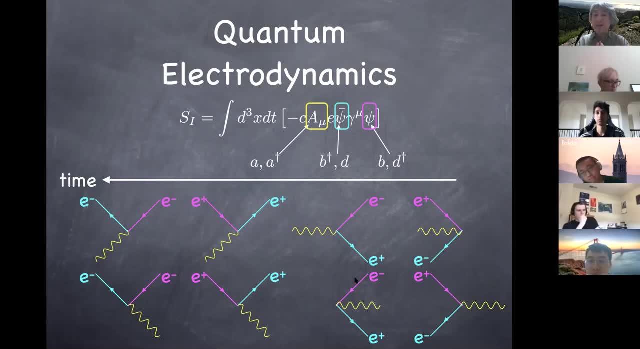 with the time ordering, So right now I can't say more than that. But you'll see why it is actually useful not to try to label each line. It's just to keep track of arrows. So I can't say more at this stage. 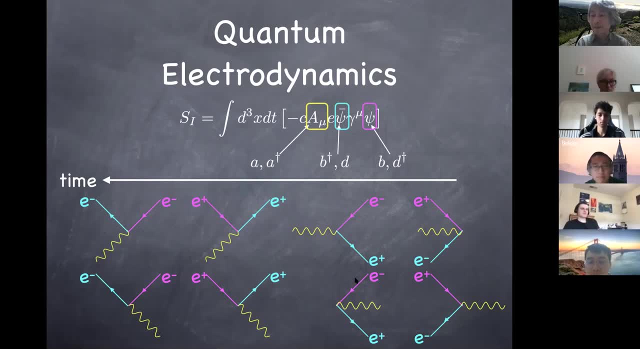 but you will see the answer to that in a moment. That's an excellent question. Any other questions, Tom, Yeah, so I'm not sure in the first place how you like, before drawing the arrows in the first place, how you determined. 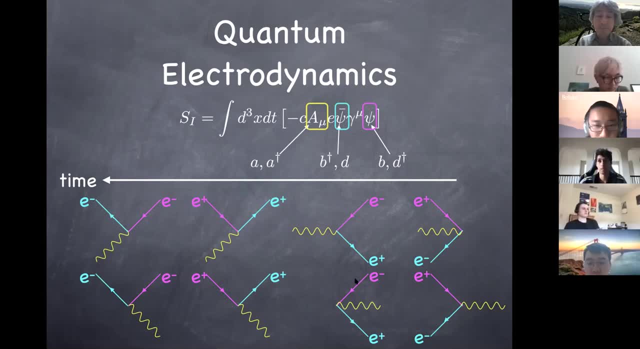 which line is like from the right-hand side to the left-hand side And which line is So. for example, in the left pictures you have the electron coming from the right, And in the right-hand side pictures you have electrons going away from the point. 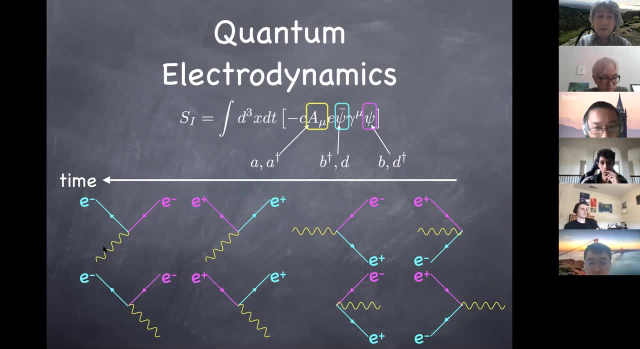 This one. Yeah, so I mean. so your blue operator in the left eye is the electron coming from the right-hand side to the left-hand side, And in the second column they appear in the right-hand side. So what's the time sequence here? 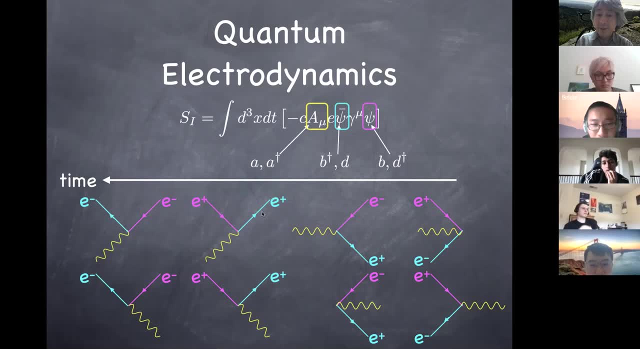 What determines the time sequence. So the time sequence is always from right to left And this positron was in an initial state which was annihilated by the antiparticle d And this magenta operator, psi, has this creation. operator of the antiparticle d, dagger. 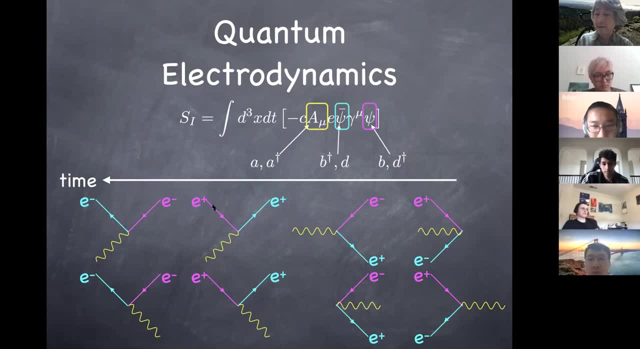 That's this magenta line. Okay, And by drawing the annihilation on the right-hand side, you are saying the annihilation happens first. Yeah, yeah, So in terms of time sequence, yes, So I'm using this psi bar operator. 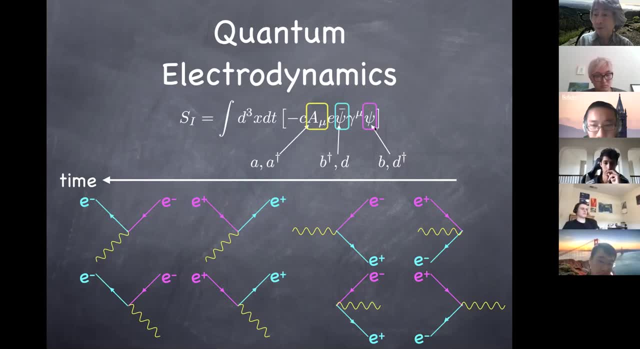 All of them are multiplied at the same space-time point. So all of these operators at the same time, right, But I use this operator first to annihilate the positron. I use the magenta operator to then create a positron, at the same time to create. 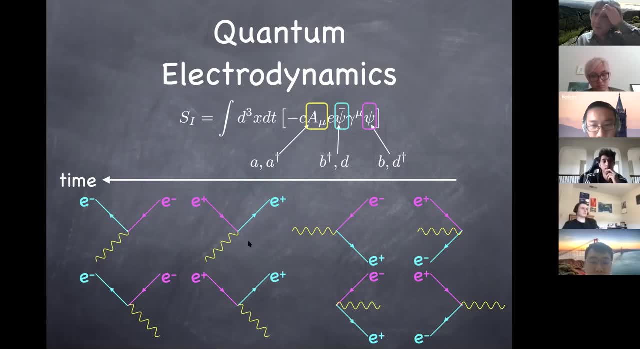 a photon. That's what this diagram is meant to convey. Okay, Okay, Does that make sense? Okay, and then you draw all the possible sequences. All the possible sequences. Yeah, so, because I have two operators in A, two operators in psi bar. 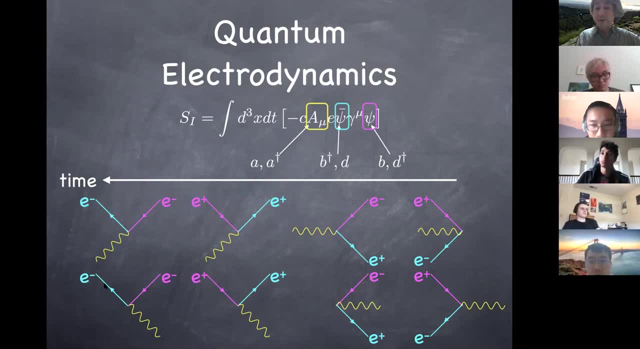 two operators in psi, I have, two times two times two, eight possibilities altogether. I see, Is that okay? Okay, thanks, Well, you can ask more questions. I had a very quick question in regards to the interaction action. So how exactly? 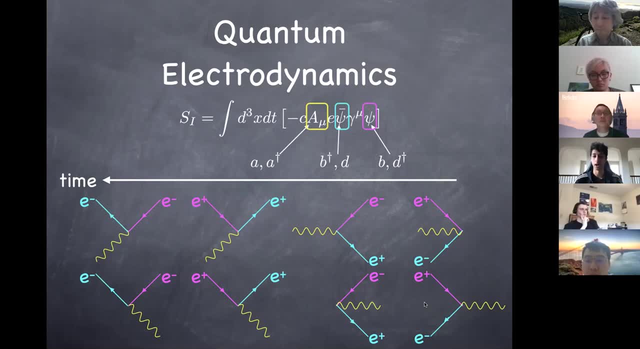 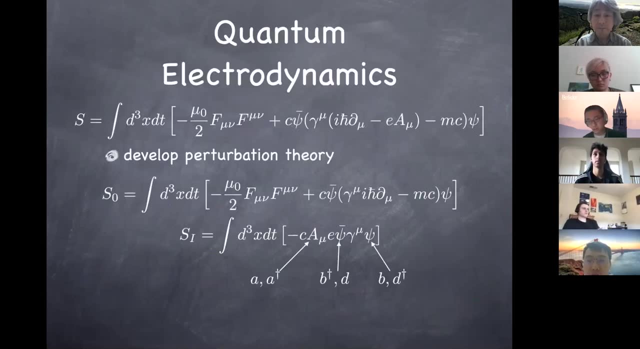 do we get that equal to the negative time derivative or time integral of the perturbation in the interaction picture? That came from here, right? So this is now the full Lagrangian of QED. First term is the free theory of photon. 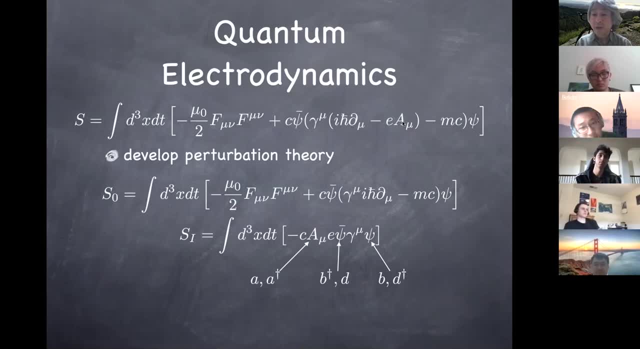 Most terms here are the free theory of electron, except this one here. So I isolated this term out of the full Lagrangian So that the first line is unperturbed theory with free photon and free electron And the rest is now new term. that's a perturbation. 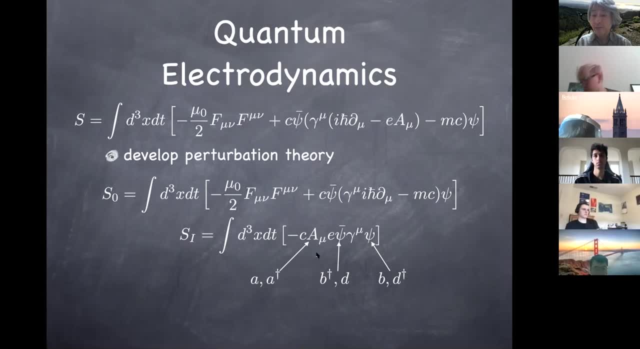 system which describes the interaction between electron positron and photon. So what we are trying to understand on the next slide we just talked about is what exactly this operator does. So that's where it came from. Oh yeah, I guess my question was how. 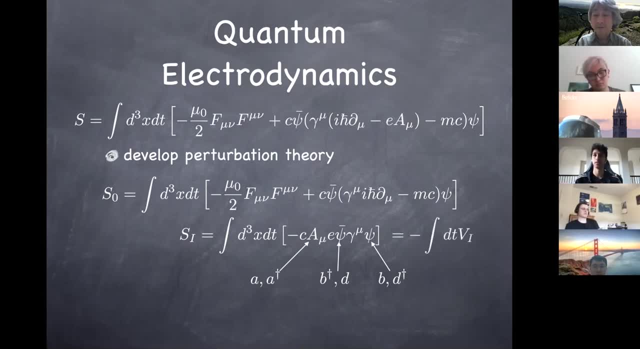 if you like, click the next point in the animation. how is that? equal to the integral on the? Oh yeah, so this is the time integral of the Lagrangian right Action is the time integral of the Lagrangian. 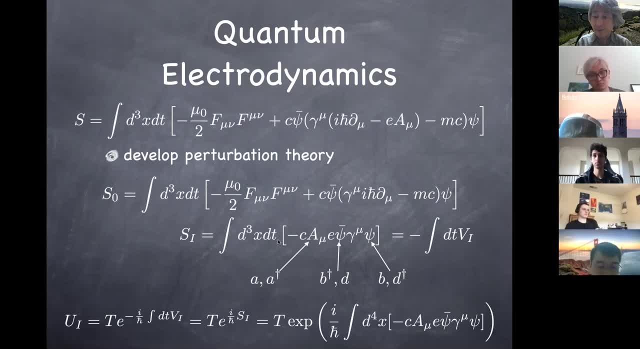 So to identify Lagrangian I remove this dt And interaction Hamiltonian is negative. interaction in Lagrangian In the particle mechanics potential comes in with the opposite sign inside the Lagrangian. So this p or yeah, where did the? 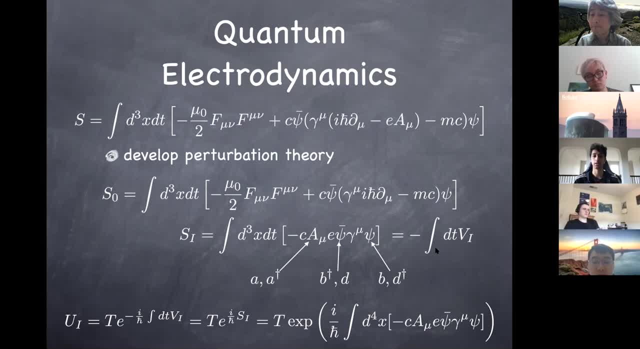 you know the, the expression from converting from the Lagrangian to the Hamiltonian. We have the, I think, what the position times the time derivative of the position minus the Hamiltonian. Is that not here anymore, or did we just drop that term? 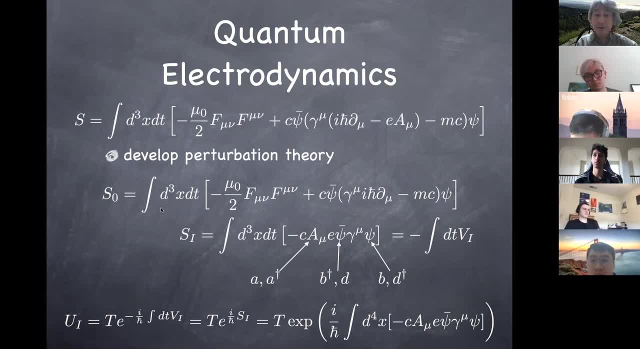 So that is meant to be contained in this free action so I didn't bother writing it. So if you start with this free action, then you can convert this into Hamiltonian and that's H naught, But this one here is not contained in it. 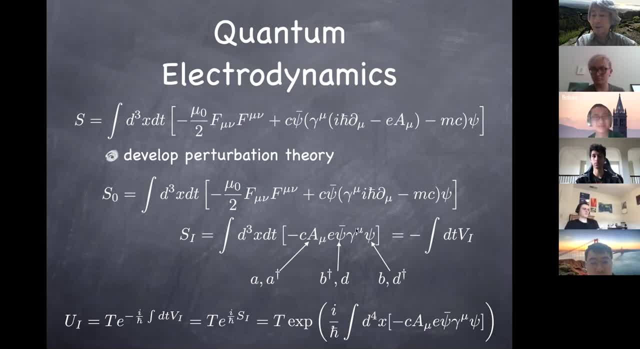 So this is meant to be the analog of the potential energy term in the quantum mechanics. So in Lagrangian that's negative potential energy. So that's why there's a minus sign over here. Okay, And then when you look at this time, evolution- 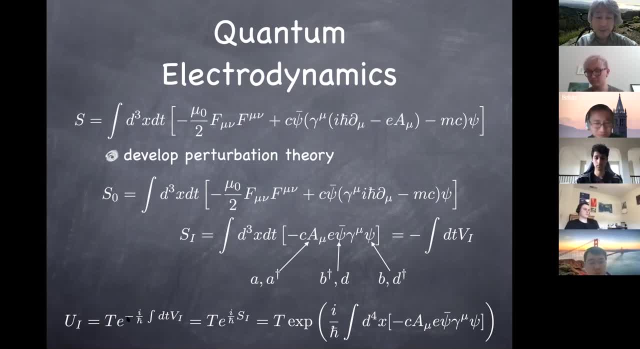 operator in interaction picture. what you have in the exponent is negative interaction Hamiltonian, which you integrate over time, So that actually turns into exactly the same thing as this interaction term in the action And that's why we're using this term here for the rest of the discussions. 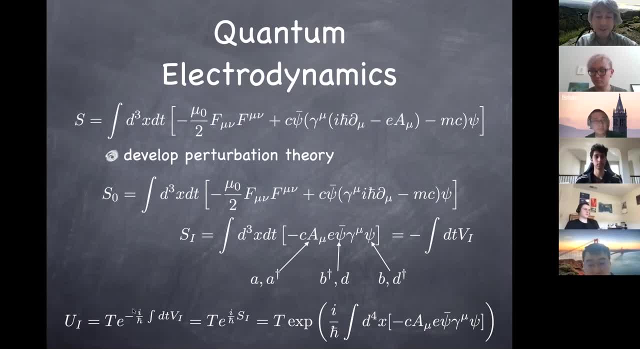 So maybe this was a confusing way of presenting because I switched the sign going to Hamiltonian and switched the sign again back to the action And that's why the action itself appeared here. But this actually turns out to be quite general in any theories we might actually think. 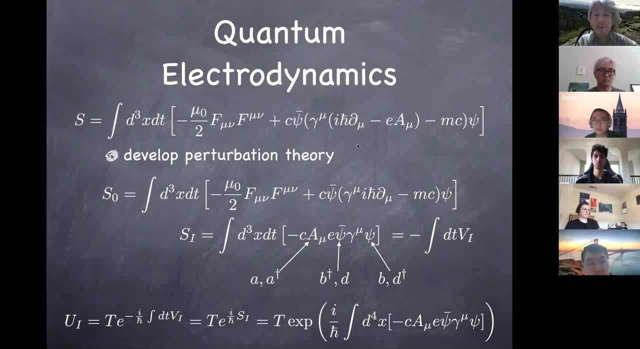 about. So it turns out that you just separate the original action which is given by the Lagrangian into the free piece and additional piece and you put this additional piece into the exponent and do the time order product and that defines the. 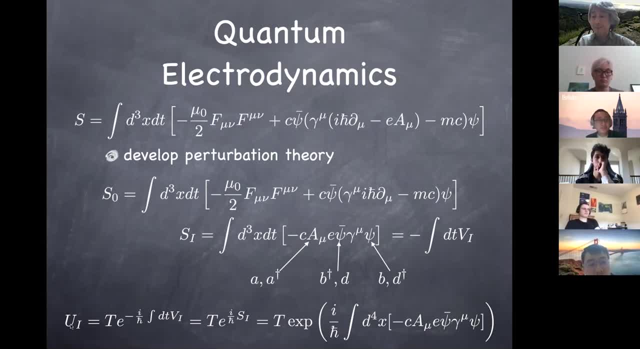 time evolution operator in the time-dependent perturbation theory. Sure, Okay, And the creation and annihilation operators are expressed also in the interaction picture, such that the potential v is now the interaction. That's right. Right, And because the time evolution of operator interaction. 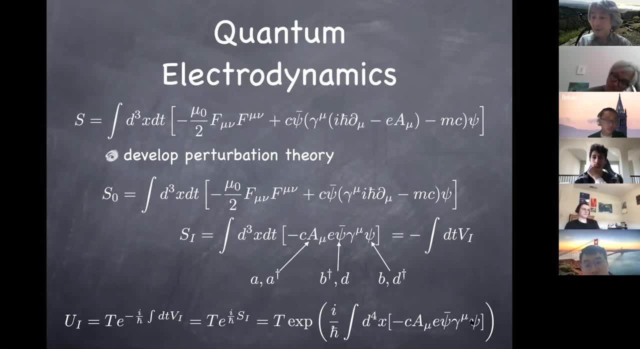 picture is according to the free theory. all of these things- psi, psi, bar and a- evolve according to the free theory And that's why we can use this mode- expansion of the free theory- to identify creation and annihilation operators in this interaction. Hamiltonian. 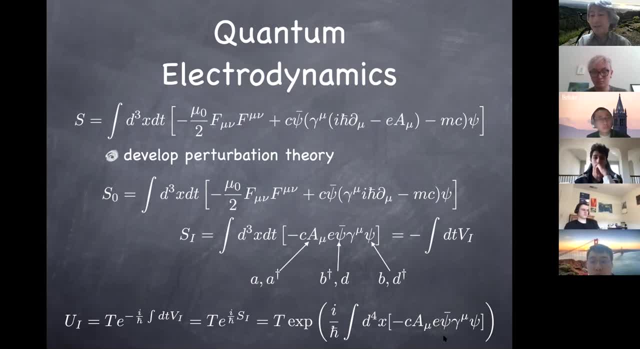 So this is, you know, ingenious And the people actually. the first person who clearly formulated this is Freeman Dyson, who only recently passed away at Institute for Advanced Study. He's the only physicist I know who became a well-known scientist without actually a PhD. 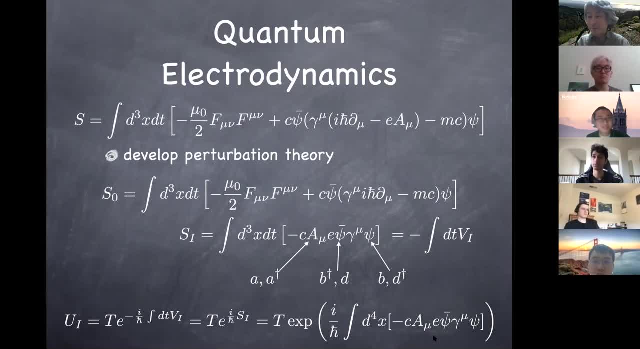 degree. He never bothered to get PhD, but he was a really towering figure in theoretical physics, And so he came up with this idea called Dyson formula, which is this formula: how to write down this time evolution, operating interaction picture which we rely on, And 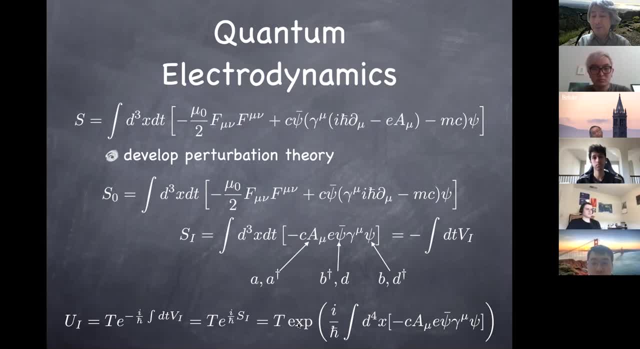 Feynman actually didn't derive Feynman rules and Feynman diagrams. It was actually Dyson. The Feynman somehow came up with this Feynman diagrams by intuition, without deriving it. So the people were initially skeptical, apparently, that that method 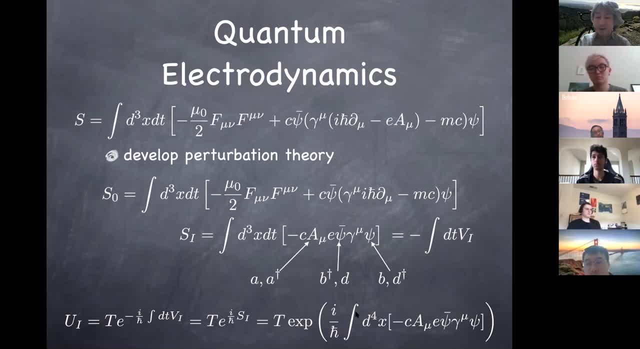 works at all, But in the end, the Freeman Dyson solidified it and derived it in this fashion, using this time order product in time-dependent perturbation theory, And that's the method we rely on these days. Okay, Did I answer questions, Sahil? 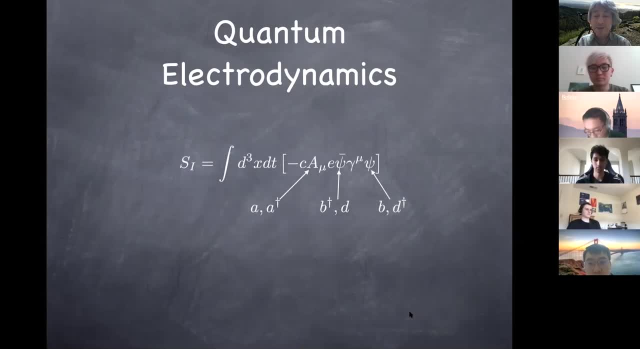 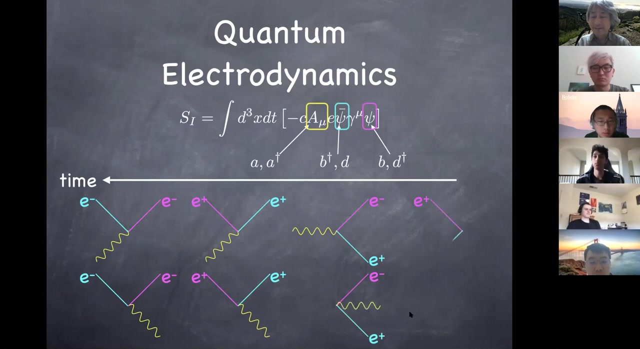 Yeah, Okay, good. Any other questions about these eight possible things that can happen from this interaction term in the time evolution operator? I hope you are recounting every process we talked about so far, So this extra time is probably not useless, but you can. 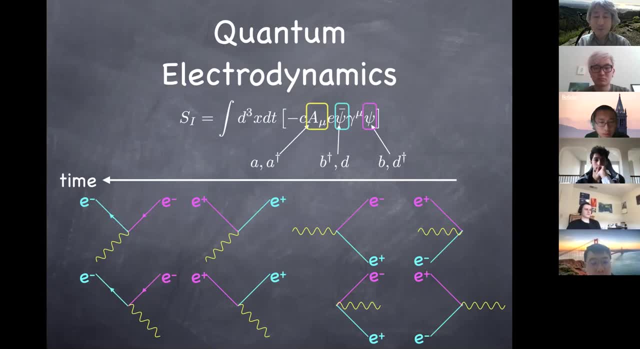 recount all the arguments we went through. So when you see backward arrow like this, it is supposed to convey its antiparticle. Here you have particle and antiparticle annihilating. Here you have a pair: creation of a particle and antiparticle. 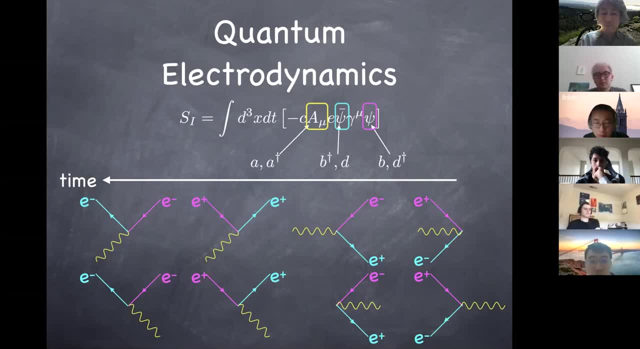 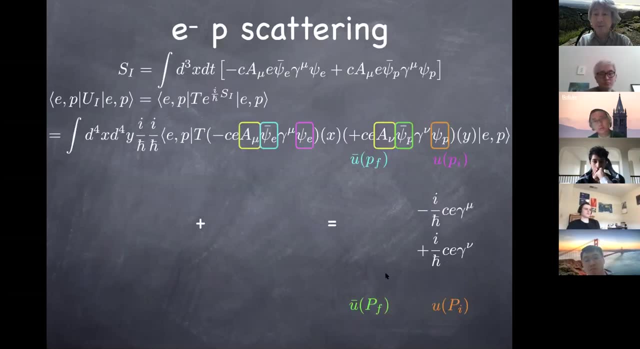 and there we go. Okay, So these are the eight possible things that can happen from this perturbation. So now we try to use this for something concrete, and that's your homework problem. So here is the interaction, Hamiltonian, Now I also. 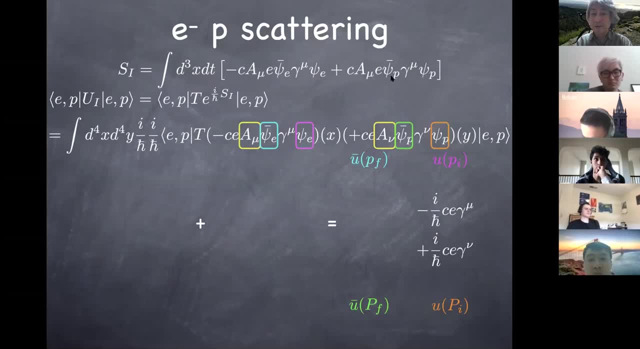 include the Dirac field for the proton. So I'm trying to understand how electron and proton can scatter against each other, And that's the analog of the waterfall scattering. So you are sending in the beam of electron, proton is sitting at rest. 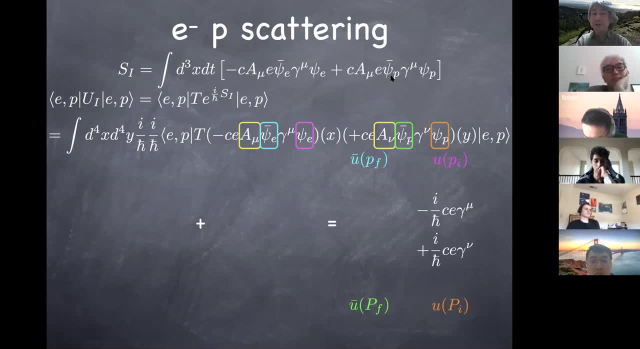 and electron gets scattered by the crude potential coming from the proton. Now we are looking at the quantum description of this process. So as a result, in an interaction term, I have this coupling of the photon to electron, Dirac field and also the coupling of the photon to proton. 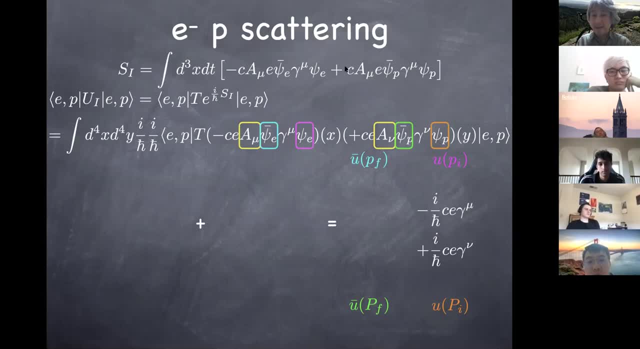 Dirac field. Both of them must be one half. They have opposite charges, so I flip the sign over here. So for electron I have minus e, For proton I have plus e, And this whole thing now goes into the exponent. 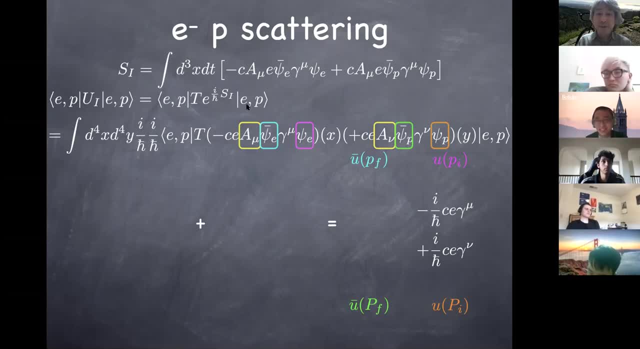 of the time evolution operator. An initial state has one electron and one proton each with some finite momentum. Final state also consists of one electron and one proton each with now different momentum after they scatter. But the idea of time dependent perturbation theory. 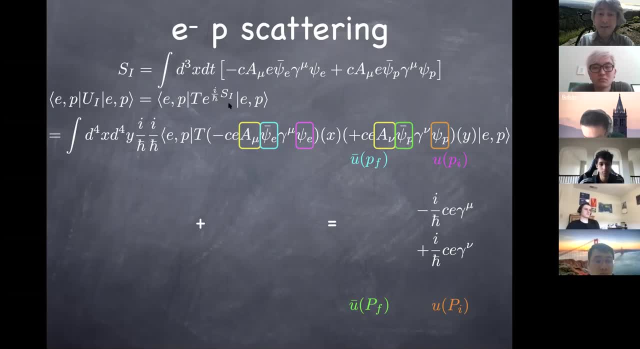 is all I need to do is to expand this exponential in power series in the exponent and identify a piece that would contribute to the finite matrix element, starting with the lowest order in the power series in e. So that's the idea of perturbation theory. 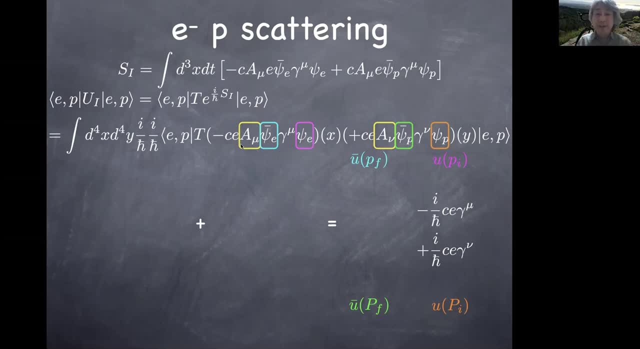 right. So then, what are you supposed to do is extract one power of the second term that is, the interaction with the proton, one power of the first term that describes the interaction with the electron, so that initial state electron can be annihilated. created to lead. 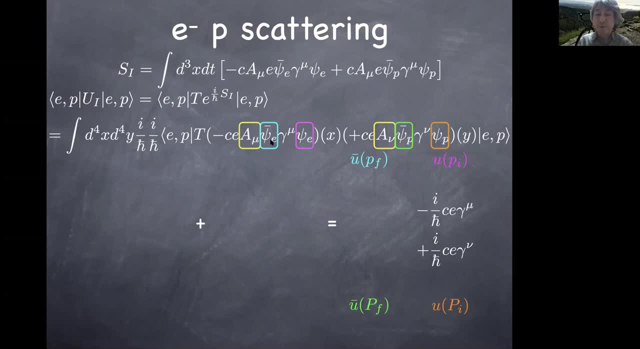 to the final state electron. That's why I need two of those, But also proton needs to be annihilated and created to go to the final state proton. At the same time, photon is created by the first operator and then annihilated by the second operator. 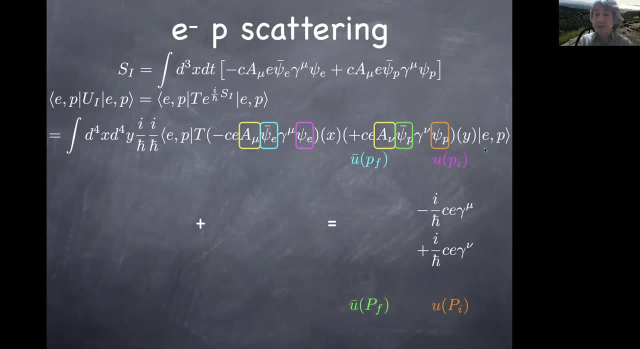 So that's the term you're looking at now in this matrix element. So this can be depicted by this following diagram. So this orange side p annihilates the proton in the initial state That's a particle. So I draw the arrow forward in time. 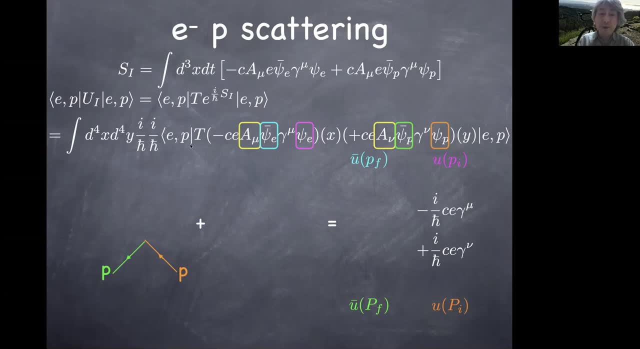 Psi bar p creates a proton that goes into the final state. So that's another line forward in time, because that's a particle proton And that's done by this green operator, psi bar p. And now comes the issue of the time-order product. 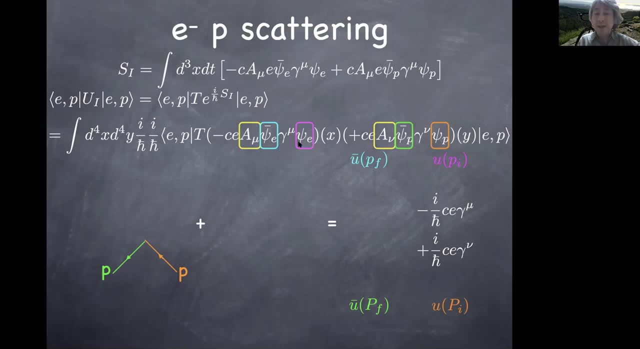 Now I'm drawing the process where this operator with the electron happens later than the operator with the proton. So what that means is that this operator involving proton field happens first and the operator with the electron field happens later, So this vertex appears at the later time. 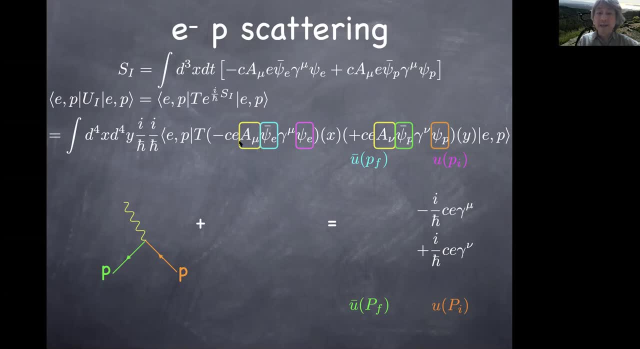 which means proton gets annihilated by the second a, mu at the later time. So that's this wiggly line for the photon And at this point the initial state electron gets annihilated and that leads to the creation of a different electron that leads to the final state. 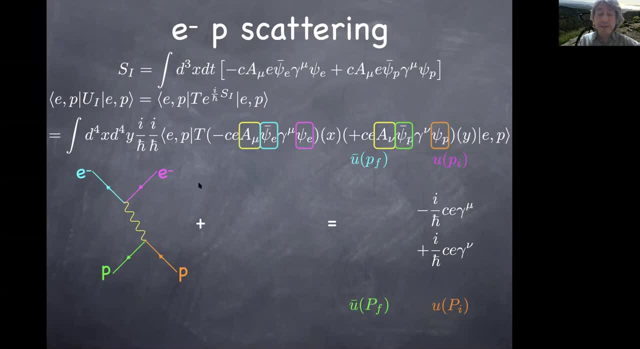 So one time ordering of these two operators lead to this diagram: Proton emits a photon first and electron absorbs that photon and as a result, electron gets scattered, So proton. when it emits a photon, again action-reaction, proton gets the backward kick, so proton itself. 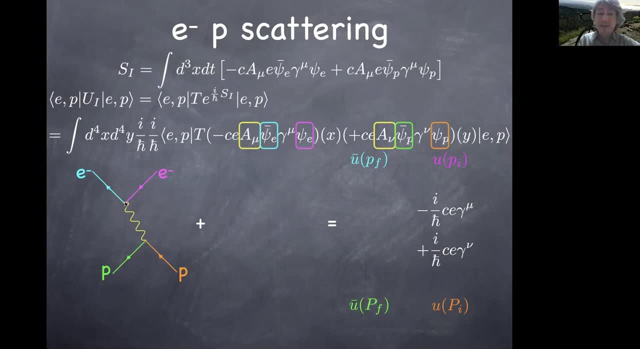 is scattered, Proton carries momentum with it that gets absorbed by this electron and then the electron gets kicked by the proton. So this is the new concept in the quantum theory of electromagnetism: scattering by a Coulomb potential is due to an exchange of a photon. 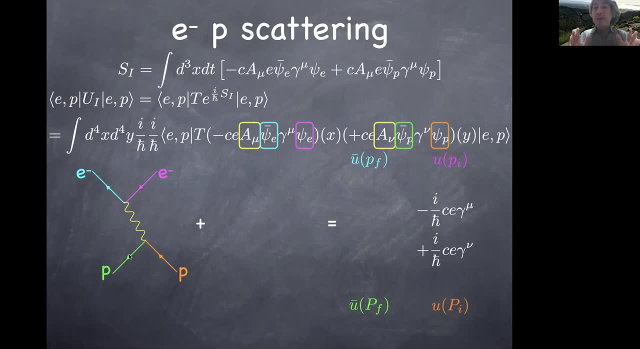 So the new concept here is that, when we think of the force going back to Newtonian mechanics, that the Coulomb force would scatter electron against proton, and that is why the function of the photon is so understood as an effect of exchanging a virtual photon. The meaning of the word. 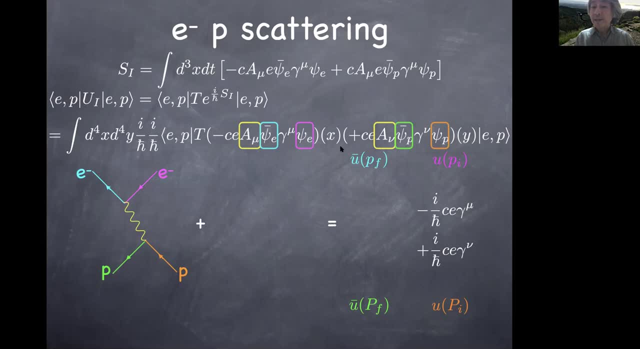 virtual is that this photon, if you insert the complete set of energy eigenstates in between these two operators, is the intermediate state that doesn't conserve energy. So that's the meaning: what used to be electronic oneness state goes to a virtual 2p state by absorbing a photon. 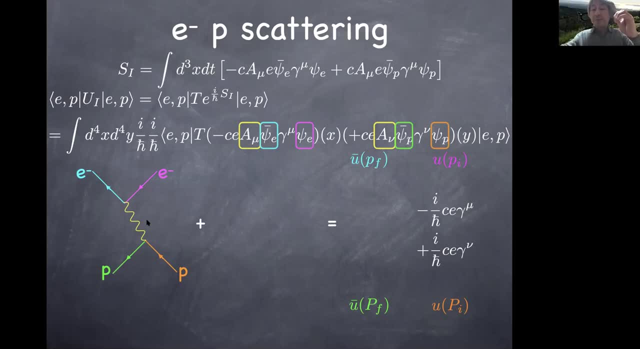 and goes back to one state by emitting a photon, and photon doesn't have enough energy to excite the oneness state to 2p state. so that's the virtual process, but nonetheless, intermediate state does go through 2p state and that's how we talked about weight is gathering and understood. 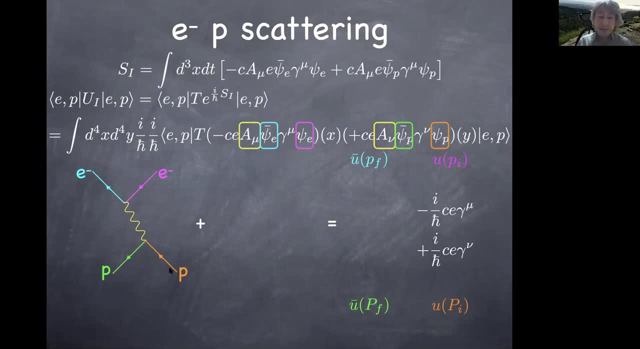 why the sky is blue. so the same idea here. the proton: initial state proton doesn't have energy to emit a full blown photon. that doesn't conserve energy. but as long as that's an intermediate state and gets absorbed by the electron, then the total energy momentum conservation is now satisfied. 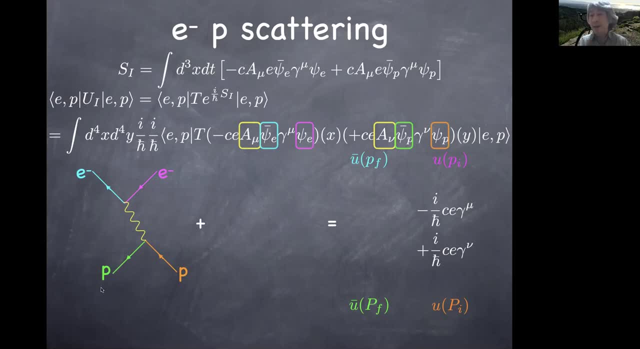 from initial state to final state and then it's okay, and that's why we call this photon a virtual photon. so the idea of the force in going back to newtonian mechanics is now replaced by the idea of sending particles back in force. you are exchanging a virtual photon, and that's what we used to think as the coolant force. 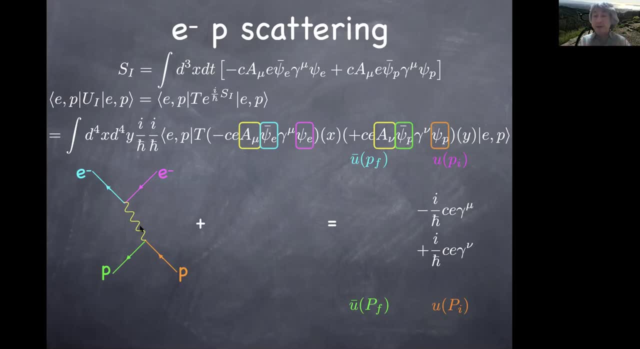 and obviously that's the natural thing to think about in the quantum field theory and that's why we call it the quantum field theory, because the other thing is no particle. the quantum field theory describes particle and wave on the equal footing. everything is particle at the same time, everything is a wave. that's the idea of 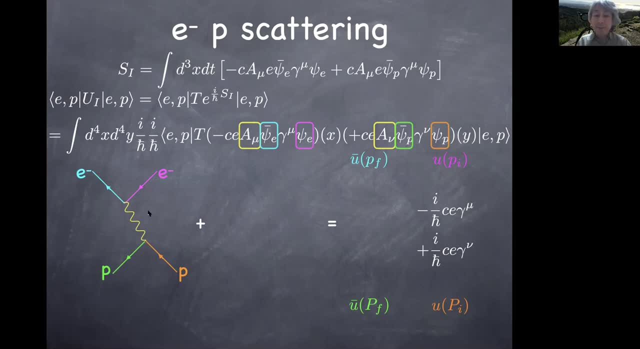 quantum field theory, and once everything can be regarded as a particle, then of course particle can go faster than speed of light. the coolant potential looks like an instantaneous force, but you already have learned in classical electromagnetism that electromagnetism cannot propagate faster than speed of light either. the way everything hinges together is based on this. 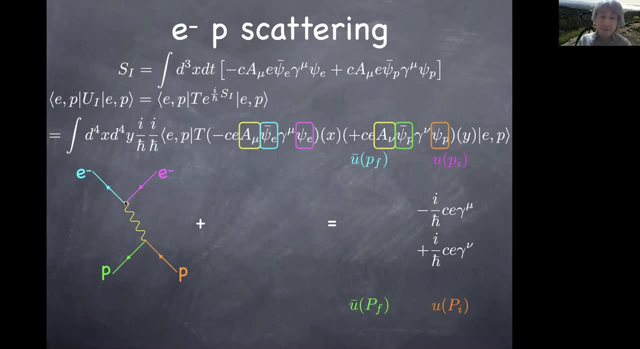 idea that you are sending a particle within the speed of light and that particle will produce a kick, and that's how the particles get scattered against each other by the coolant force we used to think of, but in reality that is caused by the exchange of the virtual photon. so that's a new concept. 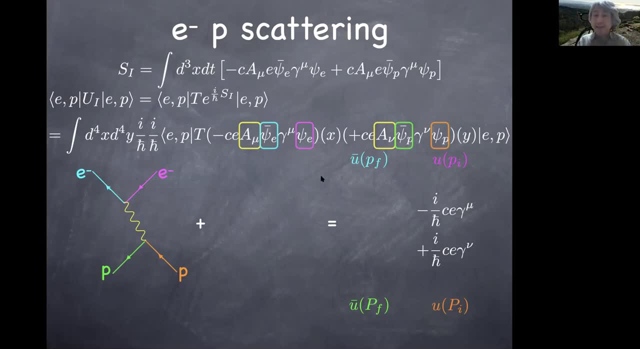 but what you see here is clearly that that is what is going on by using this perturbation theory, with this interaction, Hamiltonian, and so that's that new idea i'm asking you to absorb, and you eventually get used to this idea too. it takes time again to get synced into your mind, but nonetheless. 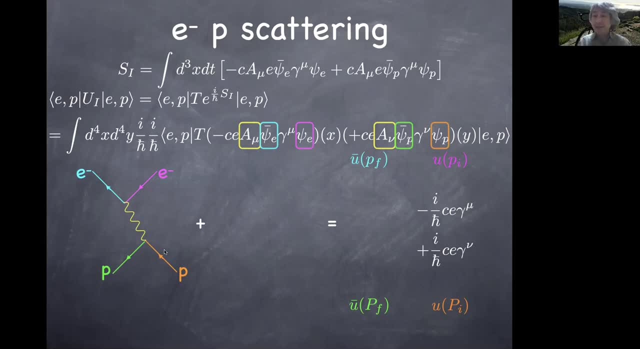 that's what we're going to do Now. let me just say that i think you know what i mean by that. you may be seeing the same thing, but actually you have to actually look at this problem that you have to try to solve in the future. we're going to look at the problem in this way and that's the way that you. 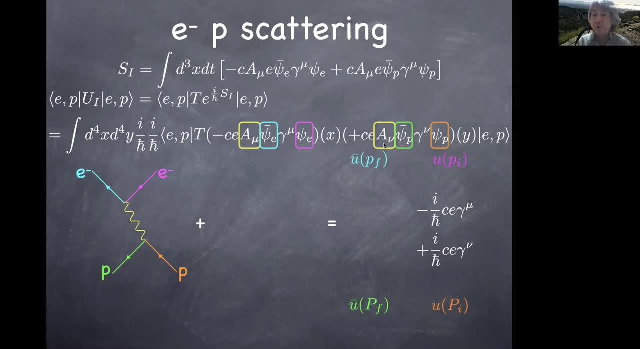 can solve the problem in your own way- and that's what you're seeing in this process and that's what you're trying to reproduce in your homework problem- by just writing psi p in terms of creation addition operator, psi p bar a nu, also by creation narration operator, and then you do the spatial 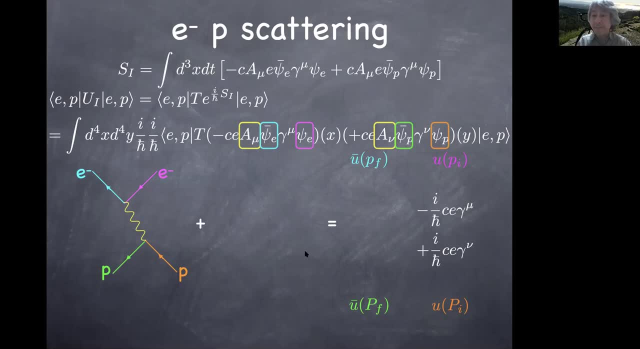 integral that leads to delta function in momentum space, then you can complete all of these. uh, the was come up in a moment, but anyway, that's what we're trying to do. But this time ordering can have the opposite. ordering Maybe this term with the electron. 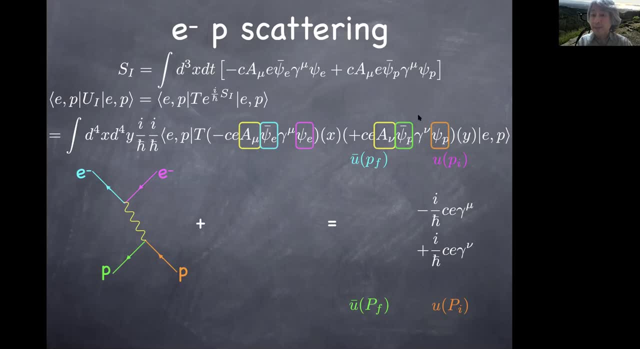 field can happen earlier than the piece with the proton field, Then what you're looking at is this process, namely that electron is annihilated, created and create a photon. This is what happens first, and then proton would absorb this photon with this annihilation. 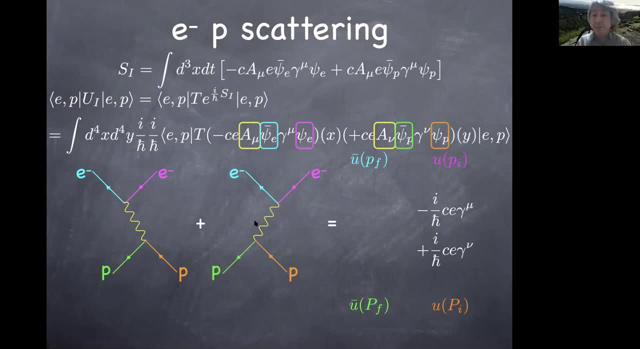 operator of the photon. So this is the opposite time ordering, So you have to sum both. But the only difference between these two processes, as you can see, is that the proton is annihilated and the photon is created. So you have to sum both. 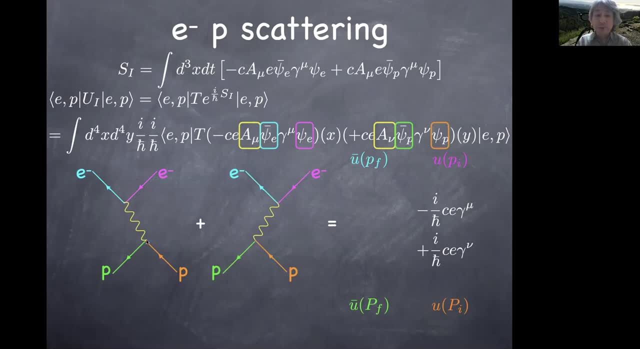 So you have to sum both. But the only difference between these two processes, as you can see, is the difference between whether the virtual photon was created by proton and absorbed by the electron, or created by the electron and absorbed by the proton. That's the only difference between the two. 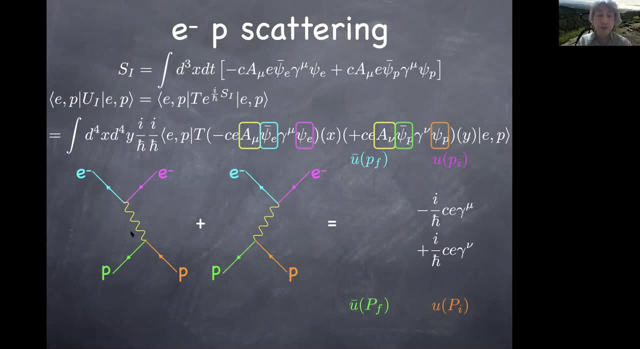 So in some sense we don't need to bother writing two different processes, as long as you use a wavy line, which is called a propagator, and that turns out to have this following form- we will justify this later on- which sums already two different time ordering. 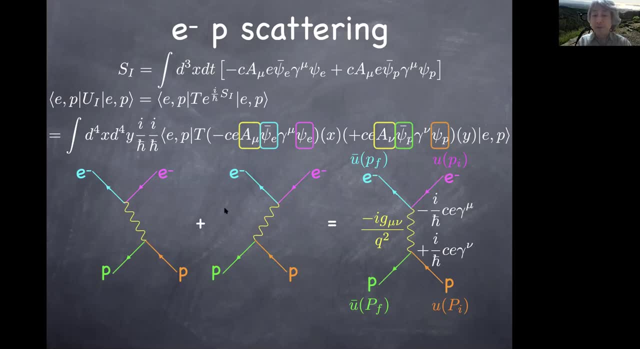 of which one emits the photon and which one destroys the photon, which can happen in two time orderings, But every time you see a virtual photon, which always comes with these two different time orderings anyway, so you don't need to remember each one of them as long as you. 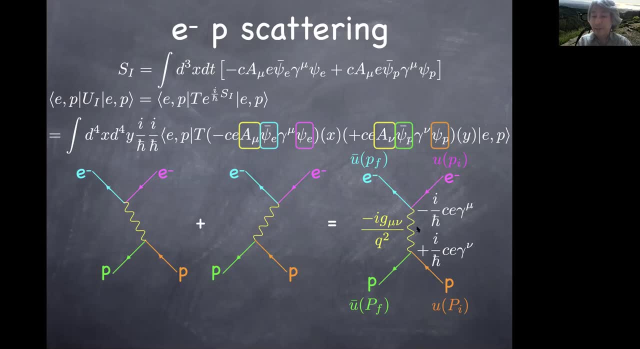 remember what the sum of that turns out to be, And that's the idea, quote-unquote, of the photon. So this wavy line now, which is drawn totally at a single instance, is meant to be the sum of two different time orderings- and I computed this for you already- which has this form of 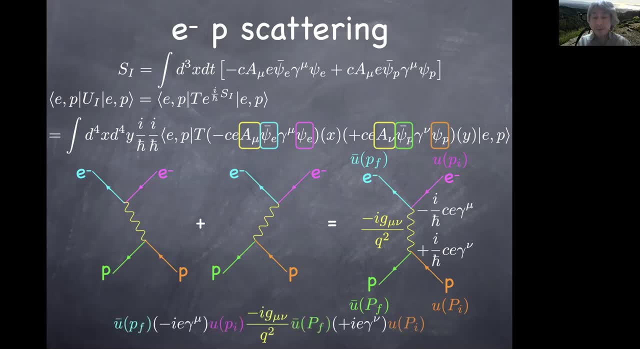 minus i g-mini over q-squared. So end result turns out to be this Feynman amplitude and that's what you're deriving in your homework problem. So the idea is very simple. If you look at this psi p field, if you look at the piece that annihilates a proton, that piece comes together with a positive. 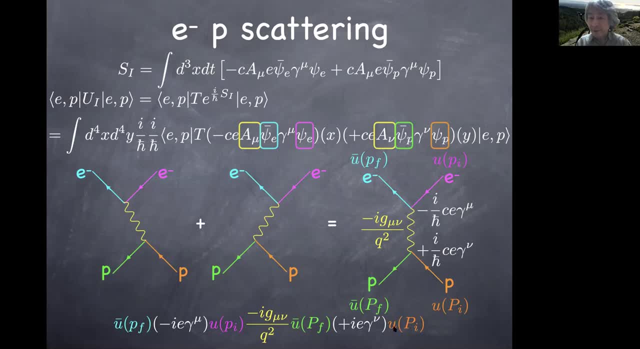 energy solution for the proton, which is the positive energy solution for a given momentum of an initial state proton, which I denoted by capital PI. Then on top of it I have this c, e, gamma, nu times i over h bar in front. That's this factor, and I actually omitted c and 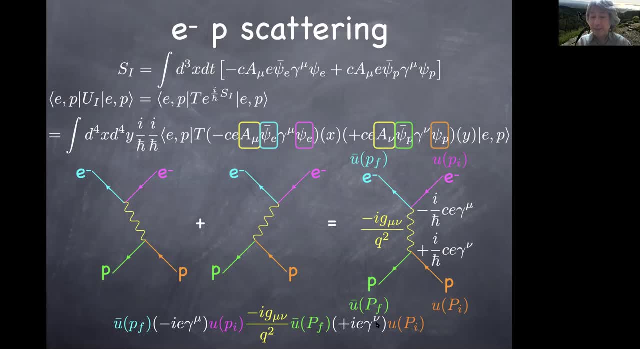 h bar for simplicity of notation. I will explain that in a moment. So that's this vertex. So if you write it fully, I have c, e, gamma nu times i over h bar. That's what I wrote over here By omitting c and h bar, that's i, e, gamma nu over here And that turns into the final state proton. 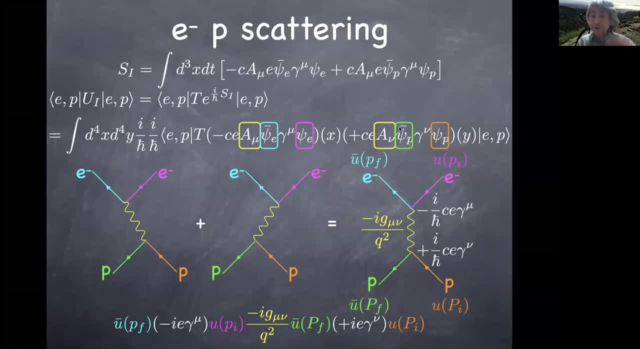 using this psi bar operator. So creation operator of the particle again comes with a positive energy solution with a bar, namely permission, conjugate times, gamma, naught, I write u bar of the final state, proton momentum, p, f. That's this side of the things. 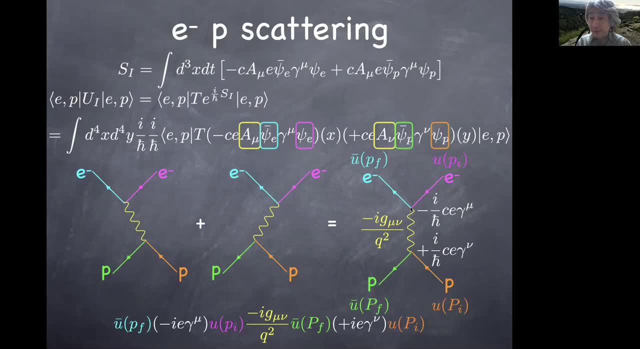 And now it doesn't matter whether proton emits the photon or electron emits the photon. Sum over the two is given by this photon propagator in yellow And on the electron side, initial state. electron gets annihilated by this magenta psi e Annihilation, operator of the particle comes. 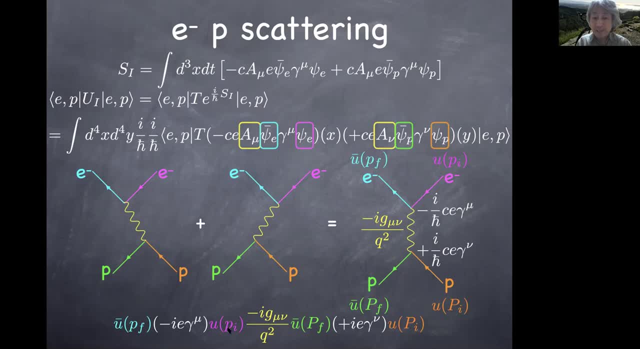 together with the positive energy solution u for a given momentum, pi. Again I have this gamma mu minus c, e, i over h bar That's written here without c and h bar, And this psi and psi bar e creates the final state electron, which comes with again positive energy solution. 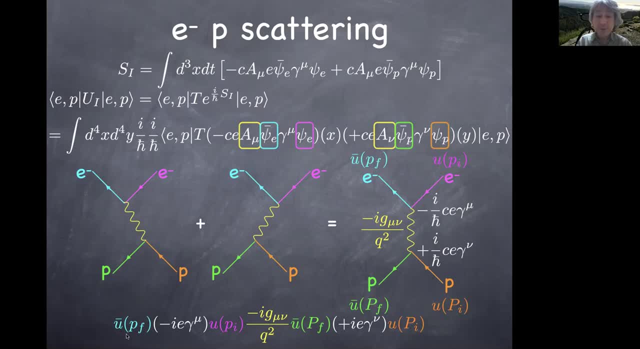 u bar, That's u bar p f. So end result is just this. So this is the beginning where you see the idea of the Feynman rules, When you are thinking about the process of electron proton scattering. all you have to do is to draw a diagram. Once you do a diagram, you associate. 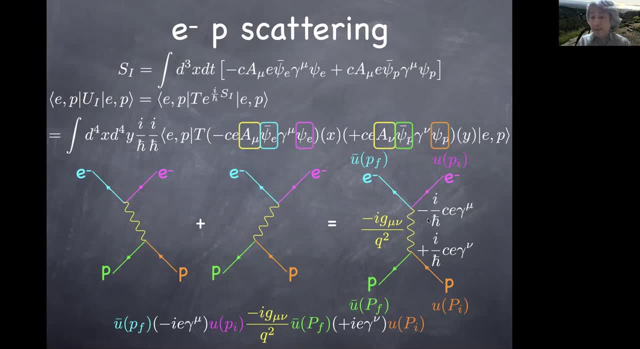 each vertex with this Feynman rule, namely minus i, e, gamma, mu. The first vertex is: it is upright. The second vertex is the Etc. Thanks for watching. It's nice to meet you. Sorry about that. So that flex is over, All right, Have a nice day yo. 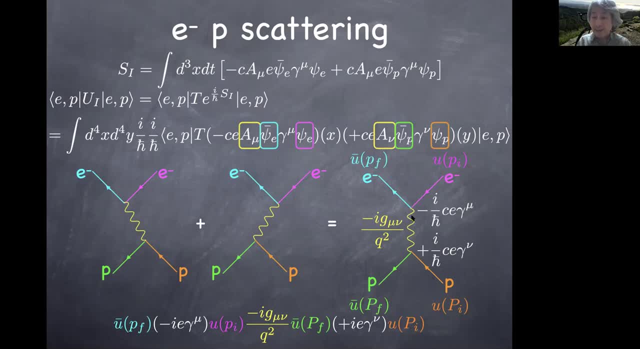 R. There's a vertex in between And between these vertices you stick in this propagator of the photon. That's this minus i g mu nu over q squared. This nu index is contracted with the nu index of gamma nu. This mu index is contracted with the mu index of gamma mu. 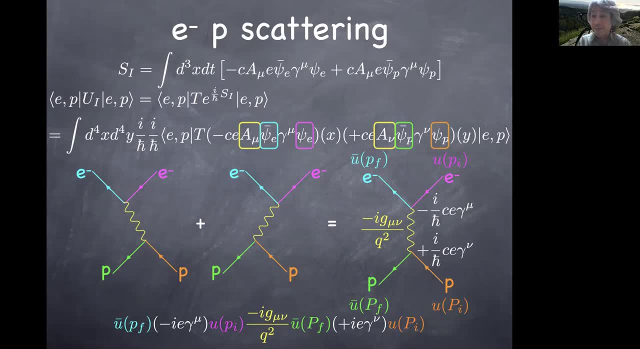 Then you see everything looks Lorentz invariant. That's the way you find the amplitude for this process And that's what you are supposed to reproduce in the current homework problem. The only thing I did not write on this slide is that when you fully do the spatial integral, 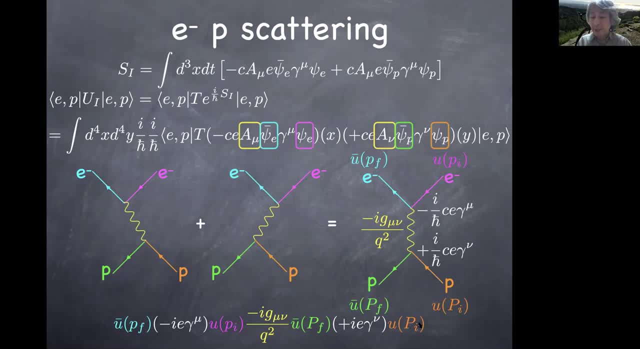 and momentum integral for all the operators. you will find also delta function for the full momentum conservation between initial state and final state. So you get this amplitude times four-dimensional delta function And that's the answer, And that's the end result of this matrix element. So the process may look complicated. 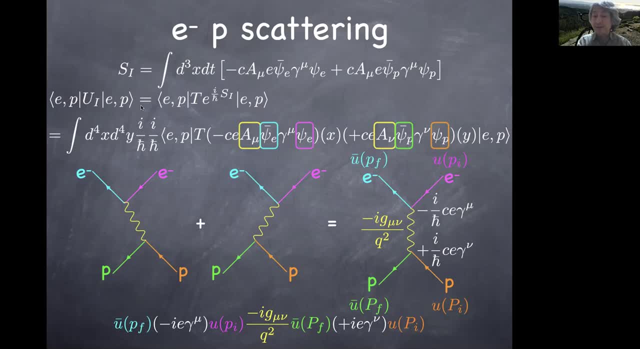 but end result is incredibly simple to understand. Once you have initial state and final state in your mind, the first thing you do is to write a diagram like this, And once you draw a diagram, you know exactly how to associate positive energy solutions and vertices, and 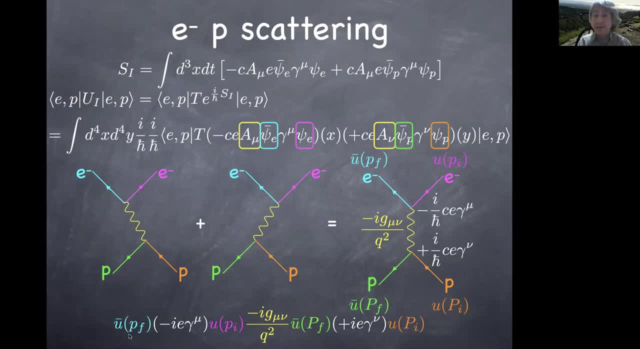 propagator. So you first write down the amplitude and then you use this simple formula to determine the amplitude, and then you use the formula for the amplitude and then you use the formula to determine the amplitude. So that's the idea that you have here. 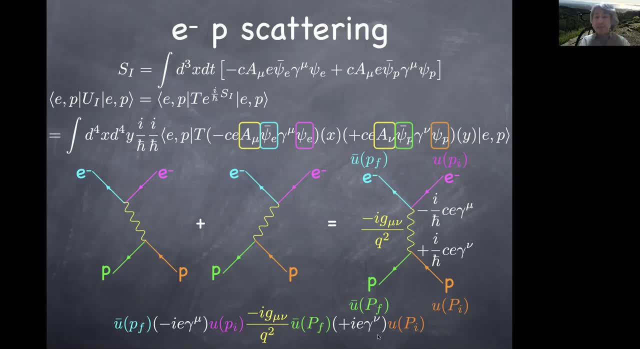 As I said, when you have the no-texture, you can make a keep cred or do the same thing like us, can understand where it came from, but end result is just as what Feynman told us: draw the diagram and you get the amplitude. So that's the idea of the Feynman diagrams. 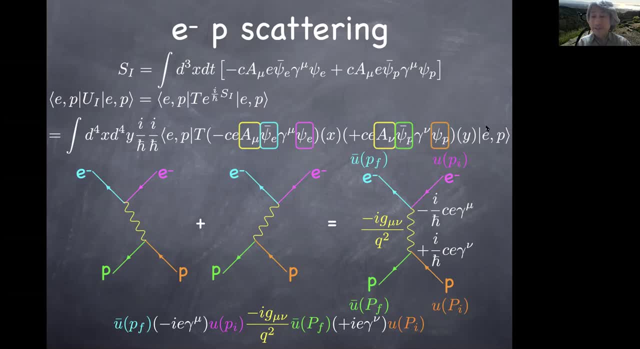 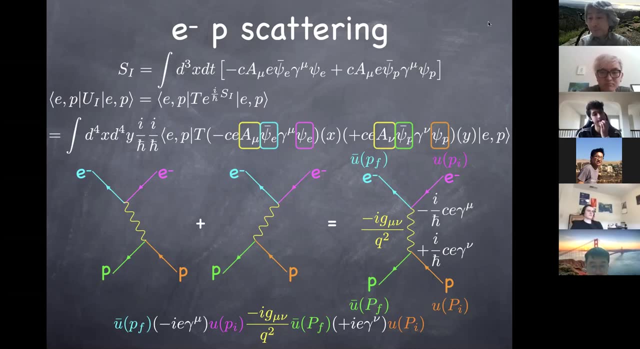 Okay, that was a long explanation. I'm sure you got questions here. I might have missed it, but could you go over again, like how exactly the we got the propagator? Yeah, so this is something I haven't fully explained, but the idea is that I have a mu here. 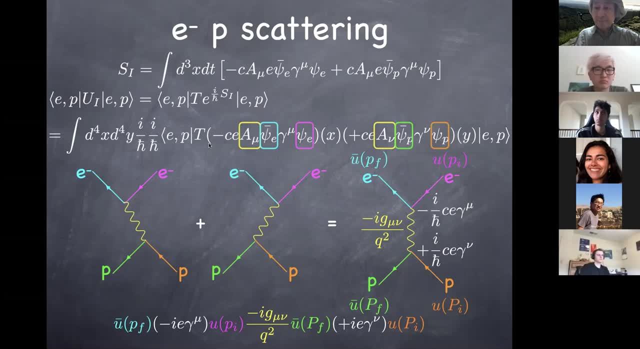 and a mu here, and the time product and initial and final states don't have any photons. So as far as the photon is concerned, that's a vacuum state. So operationally, what you need to compute is the time order product of a mu field and a mu field sandwiched between initial vacuum state and final vacuum state. 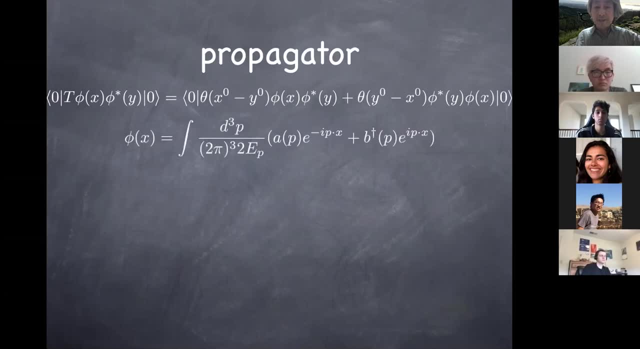 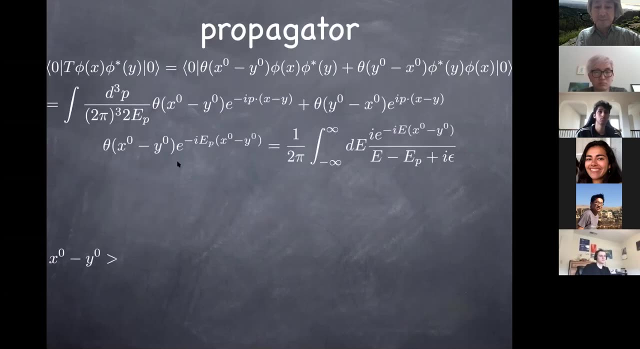 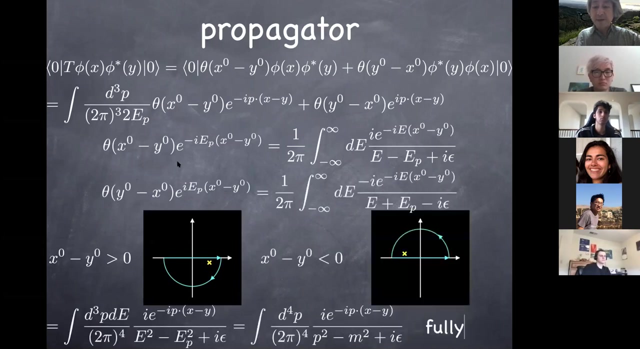 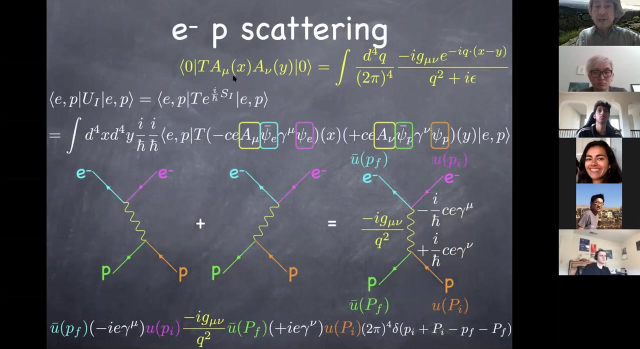 And that's something that will come up actually here- and sorry I'm going fast- and then come back to this. So this is the way I'm just defining this idea of the propagator. but at the end of the day, what you need is this: so time order: product of a mu field and a mu field from the vacuum. as far as 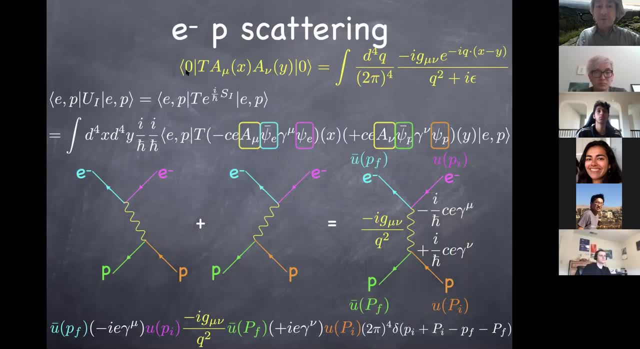 the photon is concerned to the vacuum. again, as far as the photon is concerned, can be computed and it's given by this expression at the end of the day. So this one in the integrand, except for this wave factor, is the propagator I used here for this wavy. 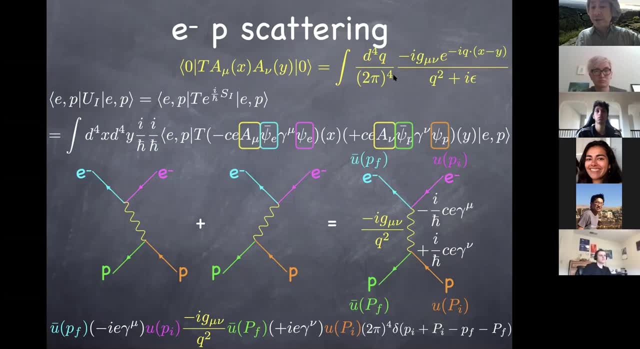 yellow line, And I would just this expression as we go on. So I sort of borrowed this idea from what I would like to explain next. But what you computed is actually this thing over here, because this is the thing which was missing in computing this amplitude: We took care of the proton, we took care of the electron. 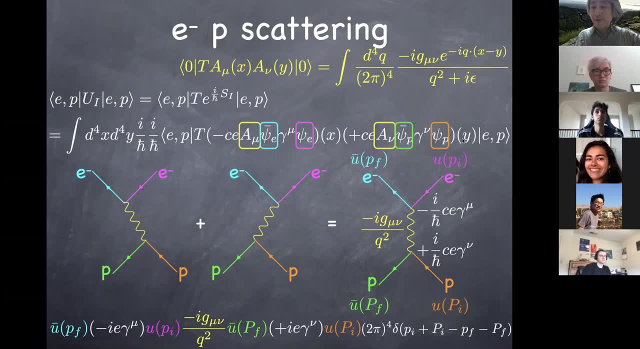 but as far as this photon is concerned, you start with a vacuum for the photon. that's this and a nu a nu a mu, a mu time-order product and a vacuum for the photon. So, as long as you know how to compute this in terms of that, there it came, this propagator factor. So that's coming. 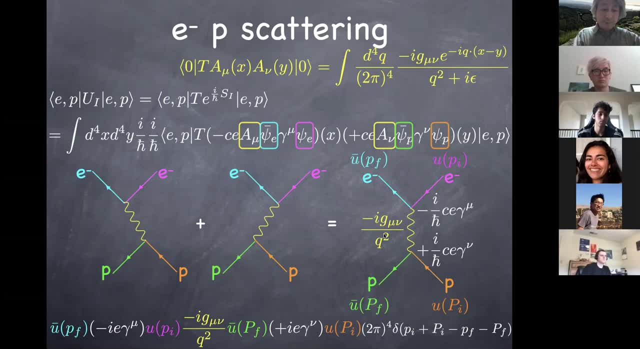 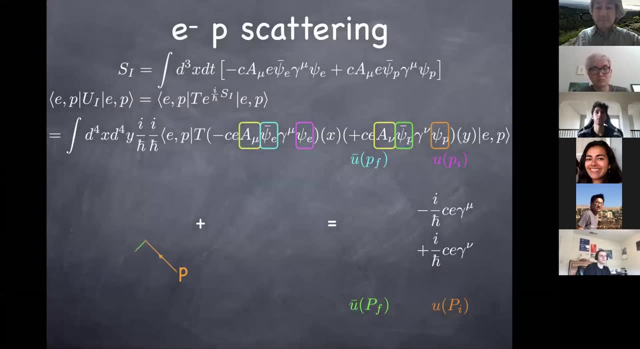 Does it make sense? Okay, yeah, All right now going back any further questions. Why do we not do something similar with the proton? We did it with the other operators, So we did it with the vector field or, yeah, with the 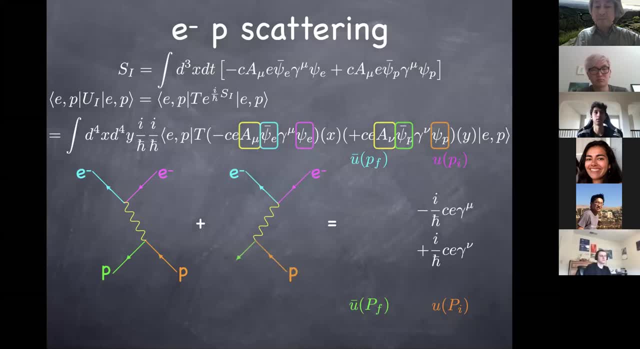 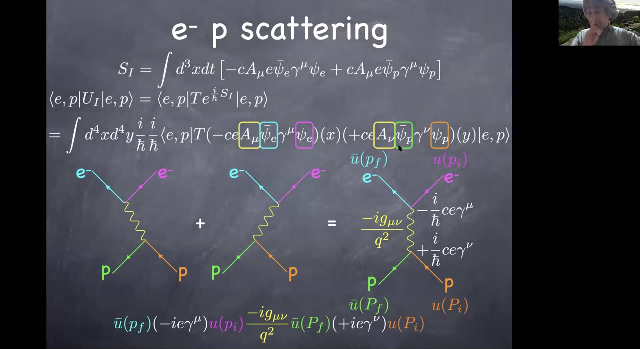 four-vector vector field. But why do we not do the similar calculation that you just flashed before? That's because we already had proton in initial state, So we can also compute the propagator for the fermion field too, which we will use later on. 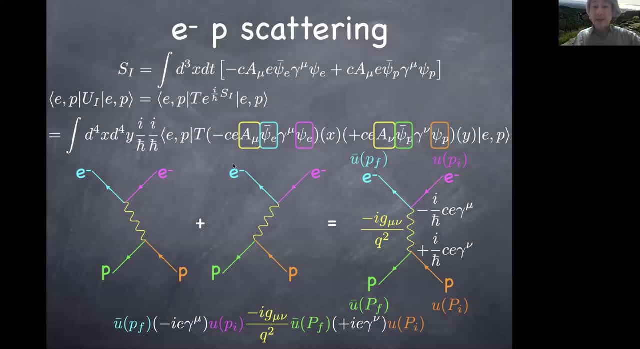 But in this case we're looking at the lowest order perturbation theory to understand electron proton scattering. If you start using propagator for the fermion field, like Psi going to Psi bar over here, then this proton doesn't get annihilated nor created. So initial. 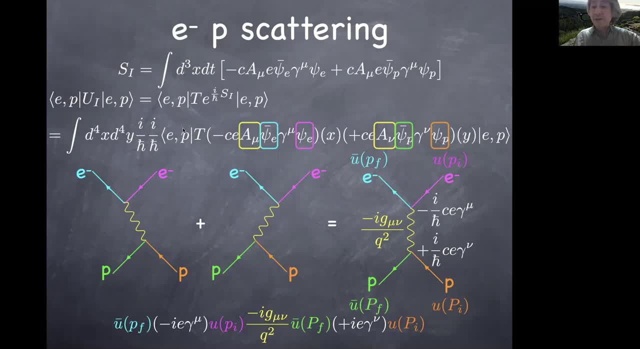 state proton would go immediately to the final state proton, which means the proton doesn't get scattered. We are interested in the scattering process, So we want to change, for example, momentum of the initial state proton in a mu, for example, and the potentialффweredêts on this basis. 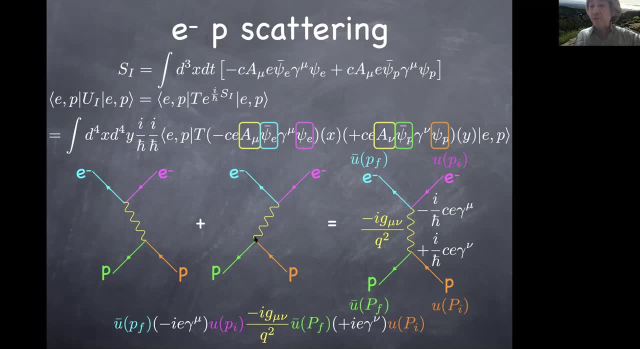 in a final state, proton by the interaction with a photon. So that's why I better use this protonization operator to annihilate this proton instead of letting propagate through this anti-proton over here. So that depends on the purpose And if you go to higher-order perturbation theory. 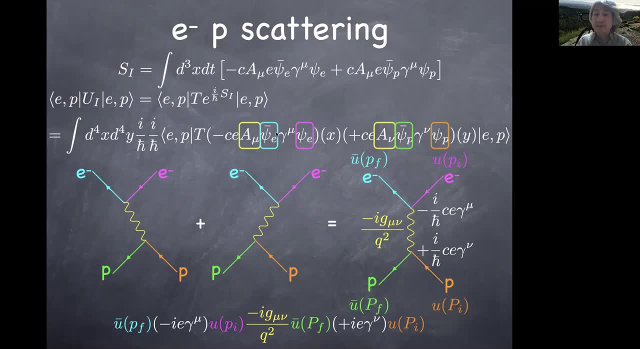 you will see a process where you also have the time-order product of the proton field and anti-proton field sandwiched between the vacuum states as a propagator, And we will end up using that too, But for this particular process, at the lowest-order perturbation theory at the least. 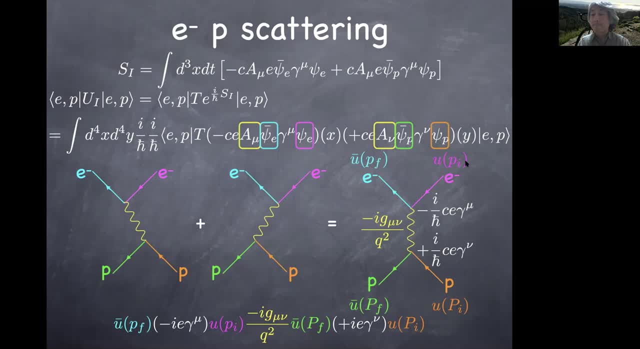 we didn't have a need for it. Does that answer your question? Seyo, Yeah, and all the coefficients or quantities we have at the bottom-most expression all commute right. So regardless of whatever the time-order product is, it's the same expression. 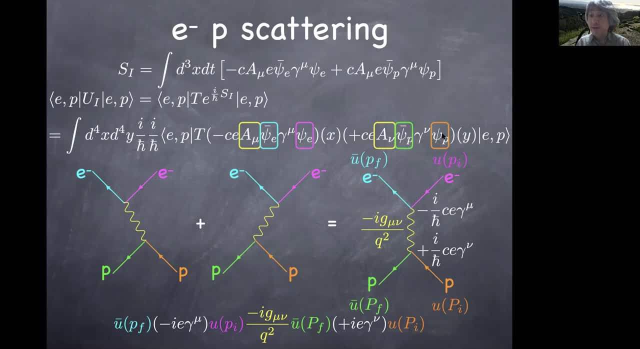 Right, because these operators have two fermion fields in it, So this is now already a bosonic permuting operators. So time-ordering doesn't change the sign and that's why there's a plus sign. Great, thank you for asking. 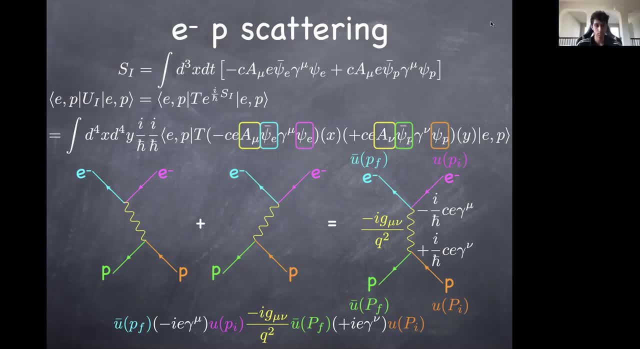 Any other questions here? I hope at least you get this idea that this complicated expression with the operators turn into very simple expression or depiction in terms of these diagrams, so that things start to make sense much better intuitively. Any further questions here? This is kind of an important point. 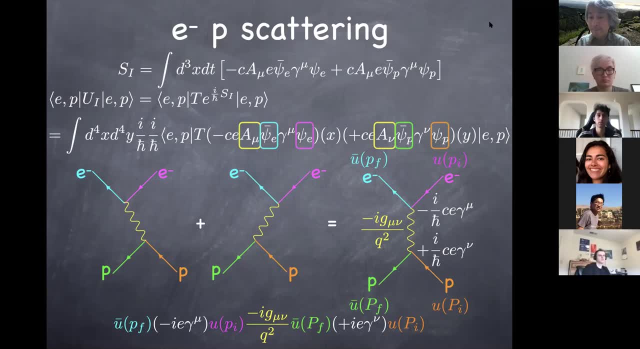 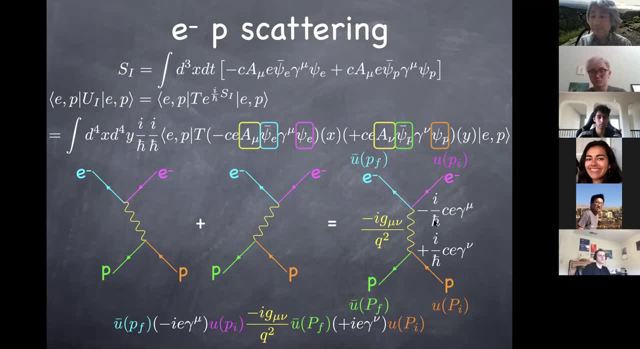 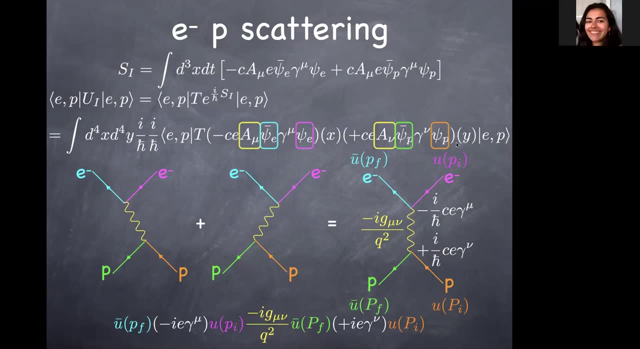 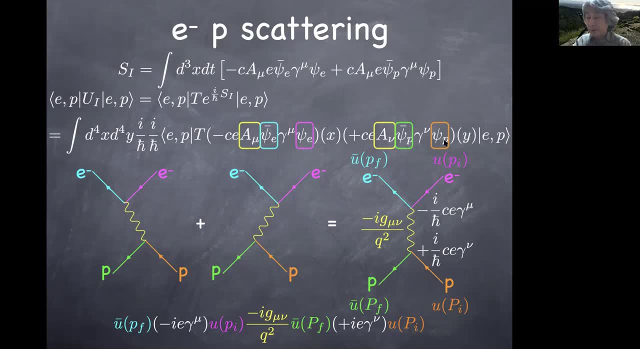 And it comes with an annihilation operator of particle times, a positive energy solution, and the creation operator of the anti particle times negative energy solution. That's the mode expansion we talked about before. So when you use annihilation operator to annihilate this initial state electron, 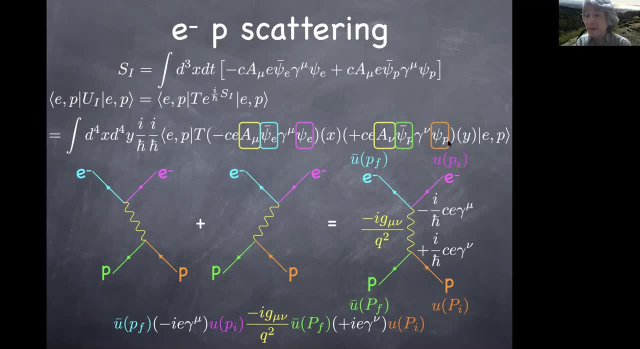 then this positive energy solution remains, remains as a part of psi, because you haven't used it, So I have to keep track of that. And that comes with this gamma nu matrix acting on it. And then I use this creation operator, proton, to create a final state proton. 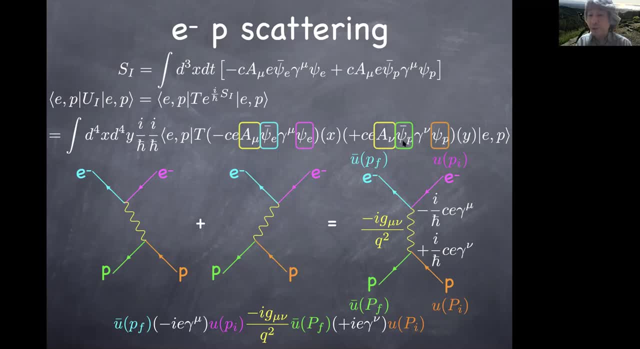 And that comes together with, again, positive energy solution, U with bar on it, And that's this U bar here. So that's how you use this operator to get this U bar, gamma, nu U, And because you know what U is, we have solved for the positive energy solution before. 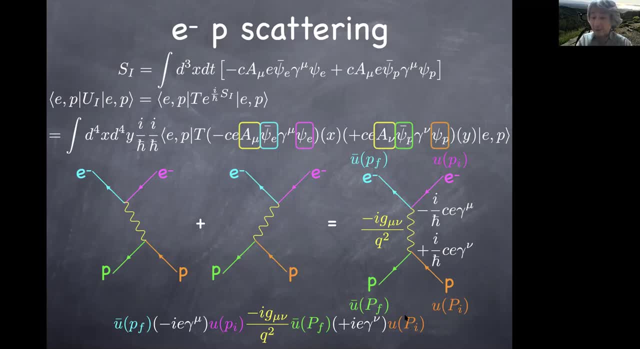 All you need to do is stick in that four-dimensional column vector for the momentum and helicity you like, Multiply gamma matrix And then four-dimensional row vector. now, This now is no longer a matrix, It's a number, But it comes with four components of U. 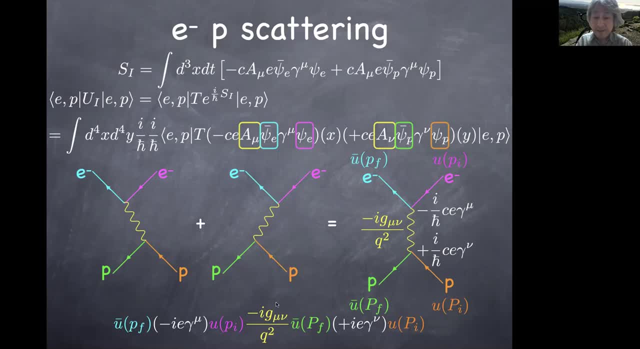 The same here numbers with four components: Then this U contract over the positive energy solution U, And then this U contract over the positive energy solution U. So in this case the whole thing now becomes a single complex number at the end of the day. 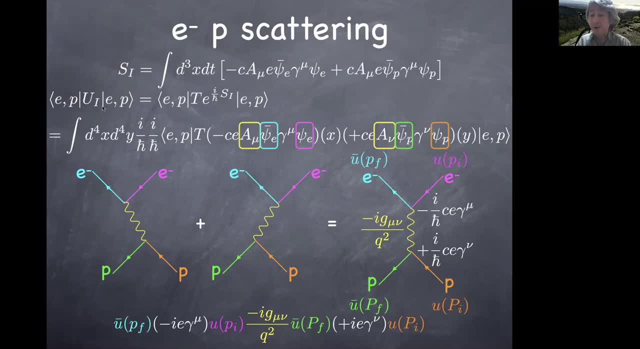 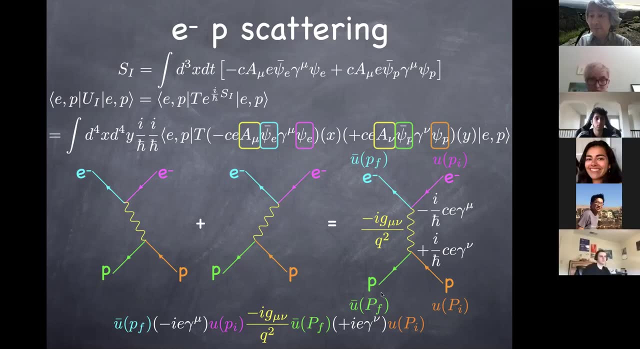 And hence that is the matrix element of the scattering process. Does that answer the question, Anna? Yeah, Thank you. Okay, great, Any further questions? So this is where all the ideas we talked about over the entire semester are now coming together into this diagram. 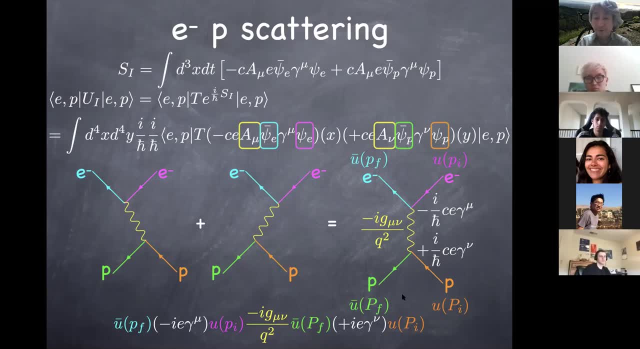 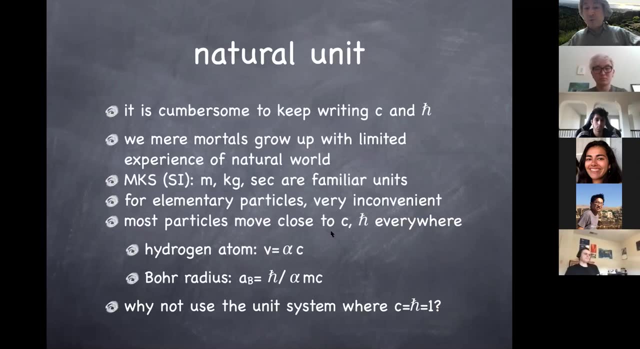 So let me go on And we can come back to it later next time. Bye, come back and talk about that more if you like, but just to get an idea on how things work. So one thing I did do here is to drop h, bar and c, and that is the idea called natural unit. because c and h bar appears everywhere in these expressions. It's just cumbersome to keep track of c and h bar and in some sense we are growing up. we grew up in a world with very limited experience of a natural world. that's why mks system with meters, kilogram and second are familiar. 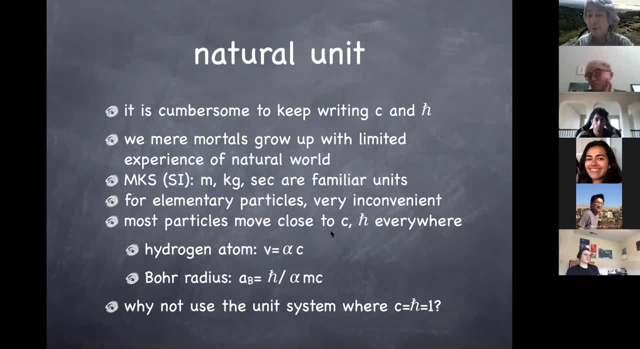 units for us, but if you are born as elementary particle that's a very inconvenient unit system. Media is huge. kilogram is way heavy. second is a very long time. So most elementary particles move close to the speed of light. h bar is everywhere. Hydrogen atom has the electron moving with the velocity. 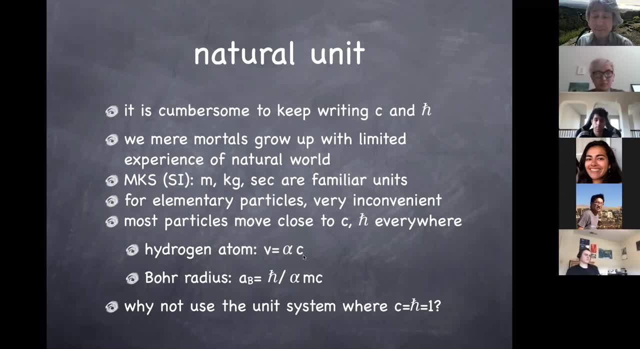 which is roughly alpha times c, that's one percent of speed of light. So everything's close to the speed of light. Bore radius is h bar over alpha and c and h bar is everywhere. So from the point of view of if you were elementary particle, it's much more convenient to use a unit system where c and h bar. 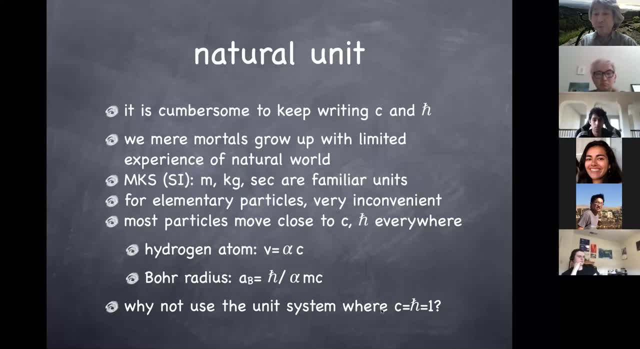 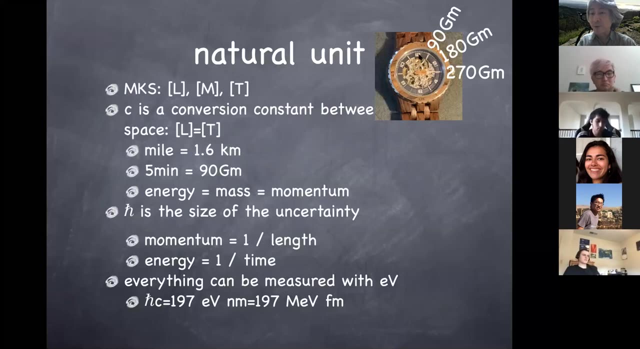 are taken care of in a natural fashion. and after all, c is just a convolution constant between time and space in the spirit of relativity. So you can measure time using length. So if you have a watch, we label the watch within five minutes, 10 minutes, 15 minutes, but from the point of view elementary. 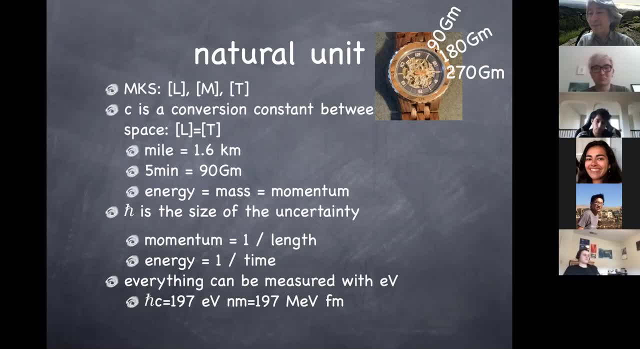 particle. it's much better to label this with 19 gigameters, 180 gigameters and so on. by using speed of light. You can measure time with meters, if you like, and you can measure distance with seconds And if you're doing high energy physics experiment. 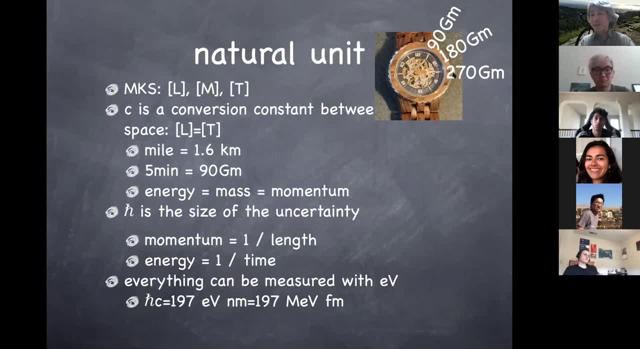 then nanosecond is a familiar unit because that's typically how long for a particle produced in accelerator would take to reach the detector. So you are basically measuring the distance with a second. So c is just a conversion constant. So just like when you say a miles, 1.6 kilometers. 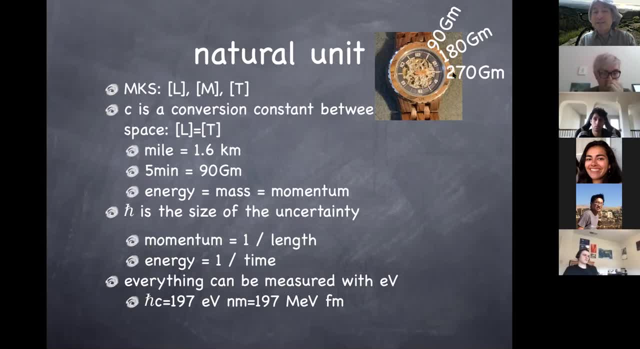 you know it's just a conversion constant 1.6.. So let's say c is 1 and you measure length and time using the same unit, then that's the idea of a natural unit. Then energy, mass and momentum all have the same unit. 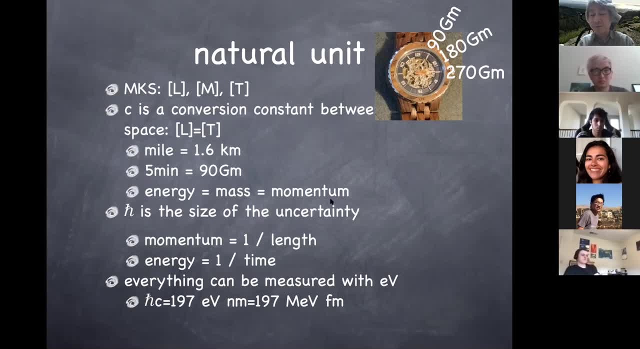 and you can measure all of them using, let's say, electron volt. h bar is the size of the uncertainty, so momentum can be measured now using the inverse length. Energy can be measured by inverse time. So mks system has three fundamental units here, but by using this idea that I have now made two of the units the same, using c, 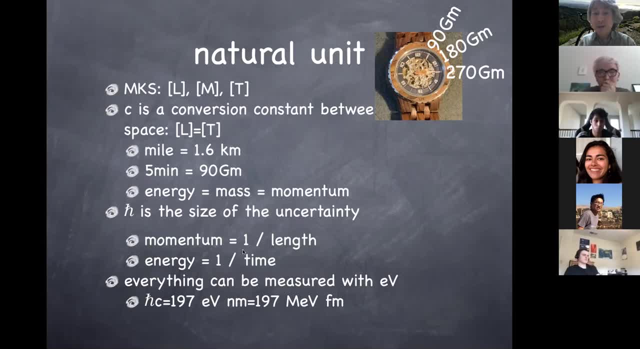 two more units, the same, using h bar. so I have only one fundamental unit left, which can be taken as electron volt or meters or second, whichever you like, But you can use one unit system to describe all of them. An easy conversion constant to remember. 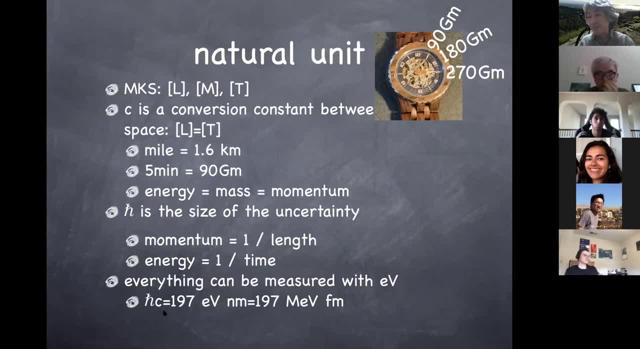 is this combination: h bar c, because c probably everybody remembers already. you know 300 000 kilometers per second, So the only new number you need to remember is h bar c In a convenient unit for atomic physics: 197 electron voltage, nanometer, because nanometer is. about the size of an atom, So you can use that to describe all of them. And the only new number you need to remember is h bar c In a convenient unit for atomic physics: 197 electron voltage, nanometer, because nanometer is about the size of an atom. 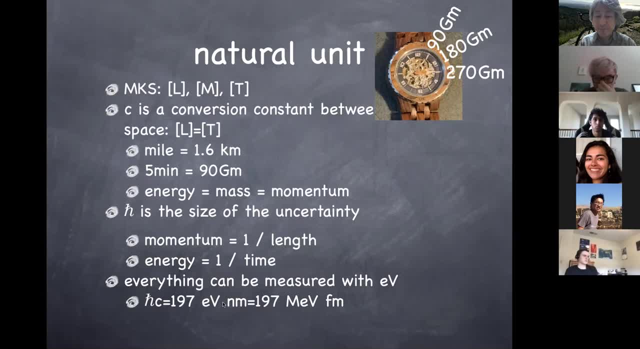 So you can use this combination h bar c In a convenient unit for atomic physics. 197 electron voltage- nanometer, because nanometer is about the size of an atom. Electron volt is size of atomic excitation energy or, if you're a nuclear physicist, 197 meV. 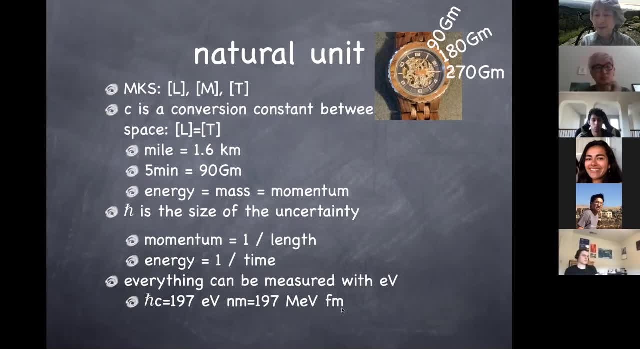 million electron volt times. femtometer 10 to minus 13 centimeter, that's about the size of the nucleus, And so this is h bar c combination, which is good to remember. then you can convert any unit to whatever you need to like. So that's the unit system we typically use when we deal with this. 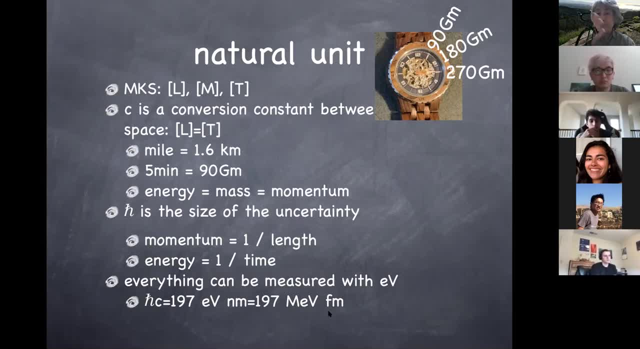 fundamental quantum system n minus 10 to the power of 16.. And again in the past, the integrals of h is one and c is one. So that's why I dropped h bar and c in expression on the previous slide, because h bar is one, c is one, But to the extent of computing numbers. 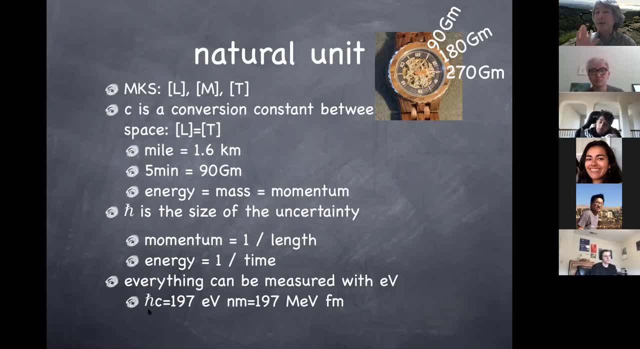 you can just keep track of what is the dimension of the quantity. Then you can recover the下一 bar and c without ambiguity, as long as you keep track of the dimension of the quantities properly. But at the intermediate stage of calculations you don't need to bother writing down h by c. 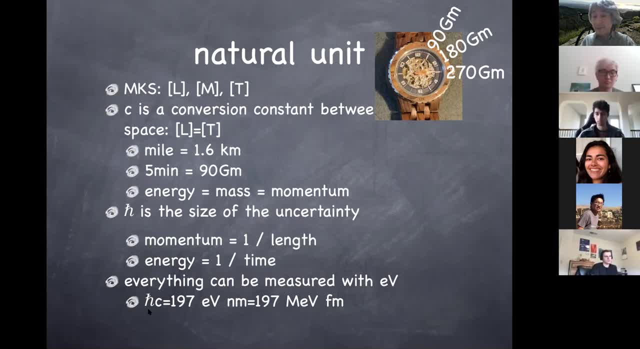 all the time. That saves a lot of time in writing and not a space on your notes or slides. So that's the unit system I use for the rest of the class today and Friday, and also in your homework problem as well. Any questions about this idea? 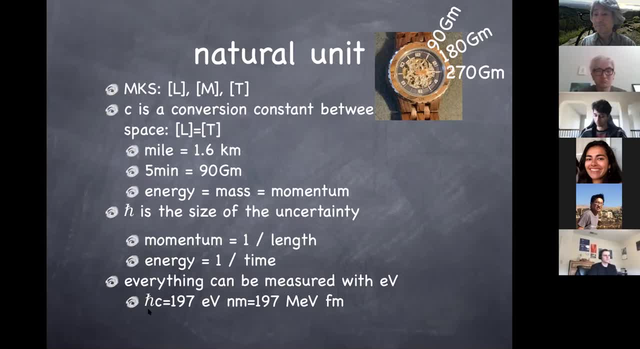 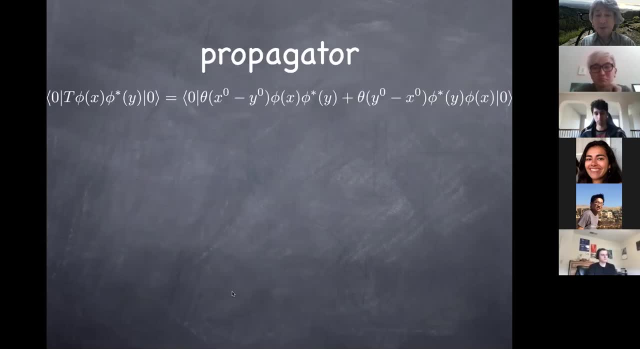 Okay. so people seem to be okay with that. So one thing I have not justified yet in the diagram I've shown earlier is with the question from Anna, and that's the idea of the propagator and that's the first part of the homework problem. So to simplify the problem I ask you to look at: 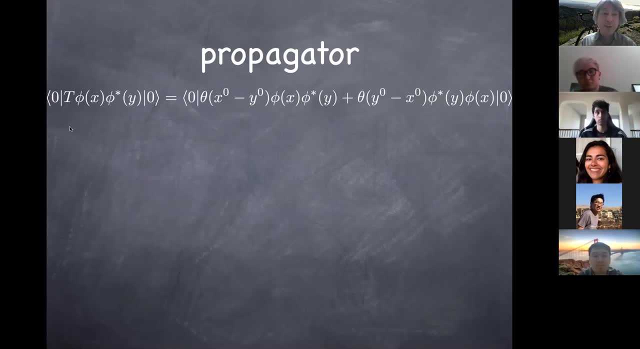 the complex Klang-Golden field, so that you don't need to futz around with a low-resolution problem. So I'm going to show you how to do that. So I'm going to start by using the simple time-order product. The time-order product is the time-order product of a field sandwiched between the vacuum state. 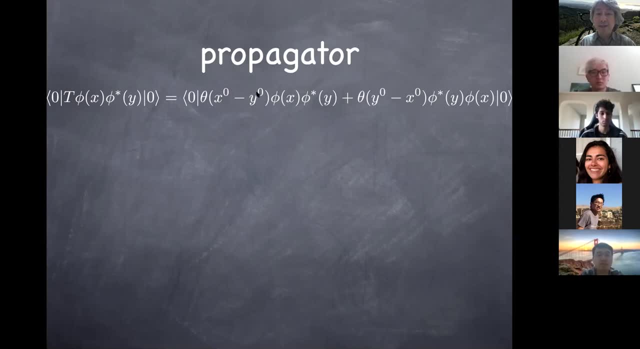 And time-order product is, of course, ordering of two operators, according to which happens later. So x naught is the time of space-time coordinate x. y naught is the time for the space-time coordinate y. you use disordering. If y naught is bigger than x naught, then y is later. x is earlier. 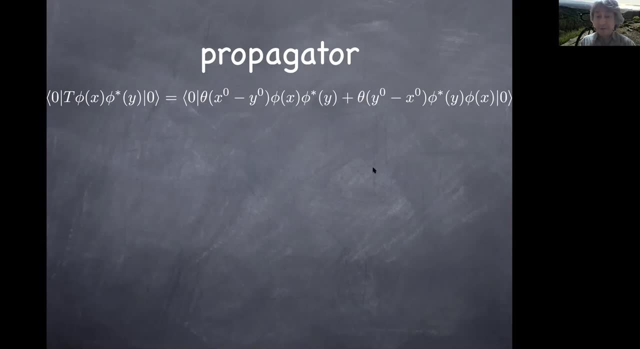 you use disordering and just a definition of the time order product, as you have seen before. And here you use this now bifamiliar mode expansion, where I set h bar and c to be one. I just stick that in there. Then this becomes this double integrated momentum space. 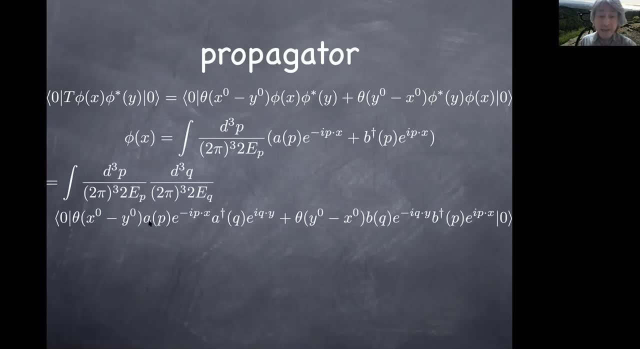 But now I have piece which is a times a dagger, b times b dagger. Other ordering of a dagger: a acting on a vacuum state vanishes. b dagger b acting on vacuum state vanishes. So these are the only pieces that would survive. Then I can change a a dagger with a commutator. 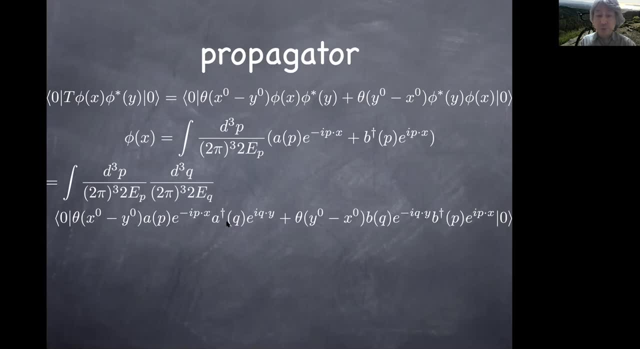 You know what commutator is: 2 pi cubed, 2e delta function. So then I can eliminate one of the momentum integrals using that delta function: 2 pi cubed, 2e times delta. Then you'll find this end result which looks kind of simple. So, depending on different time, 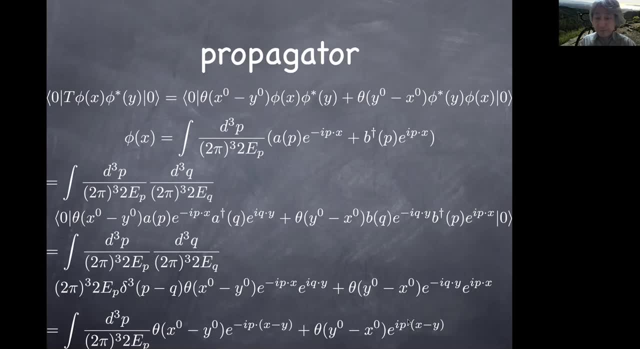 orderings. I have just a difference in the sign of these wave factors, e to the minus ip, x minus y. So that's how you compute the propagator. It still doesn't quite look a fully Lorentz invariant and that's. 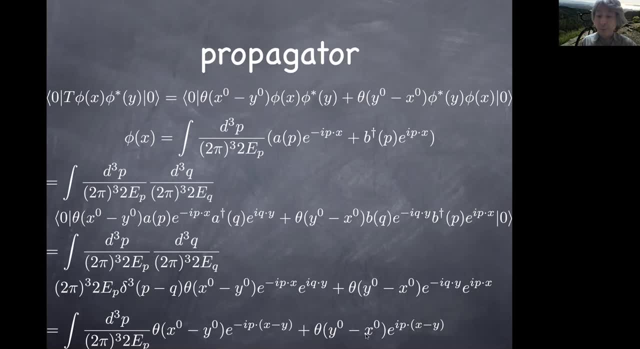 I need to take care of by properly taking care of this time ordering business. But anyway, I hope every idea here is familiar to you by now. Any questions about this? Okay, it looks okay to me then. So the the rest is we write this step function in time. 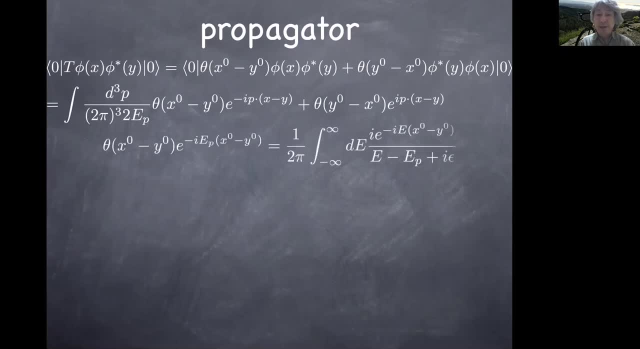 using the energy integral, And that's something we will learn about later during this session, and that's something you have done before when we were talking about the resonance. So when you do this energy integral with a pole slightly shifted away from the real axis, 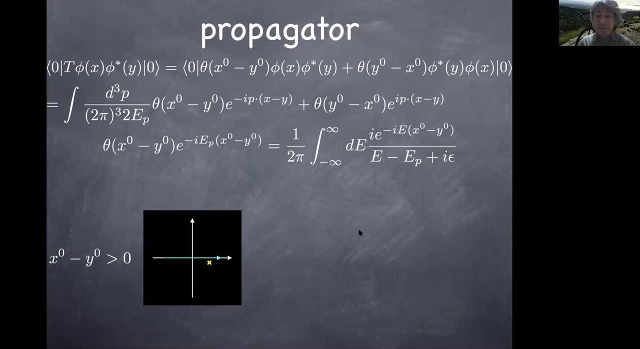 you can close the contour depending on whether time is positive or not. So when you have this integral along the real axis in E complex plane, using this I epsilon prescription, the pole on E plane is EP minus IE, which is slightly below the real axis, And when X naught minus Y naught is positive, 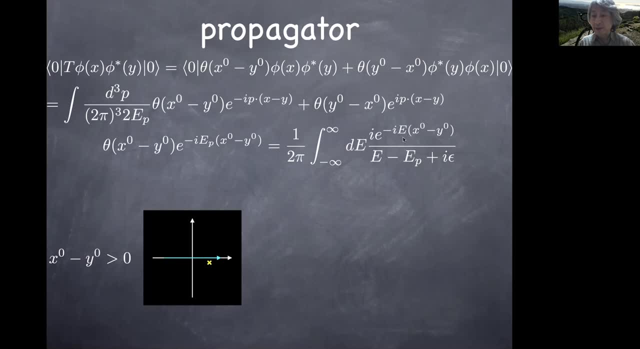 because of this minus IE factor and exponent, extending contour in the lower half plane gives you exponentially vanishing contribution. So when you take the contour to the infinite line radius, then it contributes zero to the integral. so adding this additional lower half plane does not change the result of the integral. and now you have a close contour and that picks up this pole. 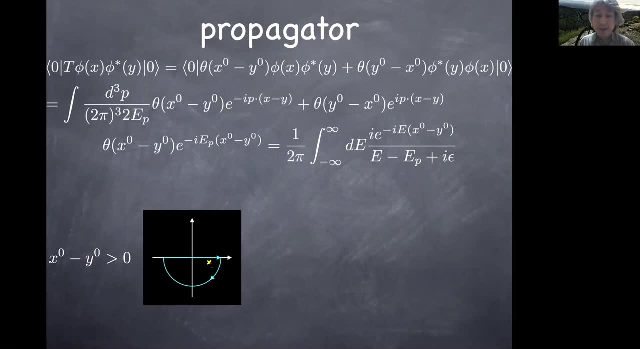 and when you pick up a pole then you have two pi minus i, so that takes care of this two pi times i, and then e is now replaced by the position of the pole, which is ep. so that's how you recover this: e to the minus iep, which is part of this, e to the minus ip, dot x in. 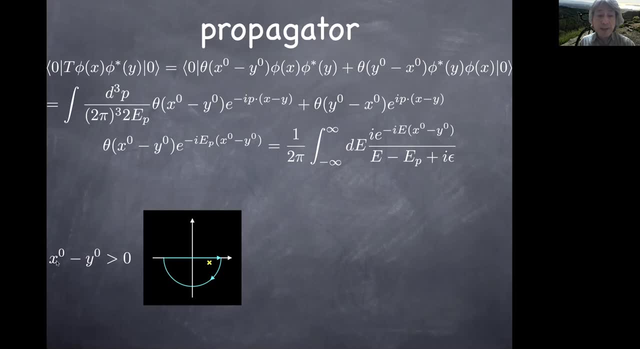 lawrence invariant inner product. but when x naught minus y naught is negative, this is exponentially large so i can't add that. so in this case i have to come back on upper half plane so that i don't change the result of the integral. but the contour in alpha half plane does not enclose the pole. 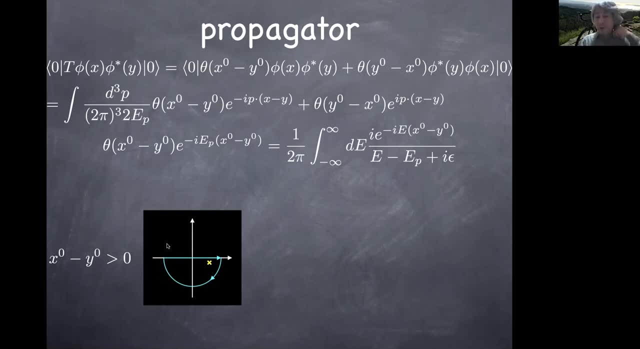 then i can shrink the contour to zero using cauchy's theorem, and end result is zero. that's why i have this step function. when x naught minus y naught is negative, then result of the integral is zero because there is no pole to encircle. so that's how i can rewrite this piece here, using: 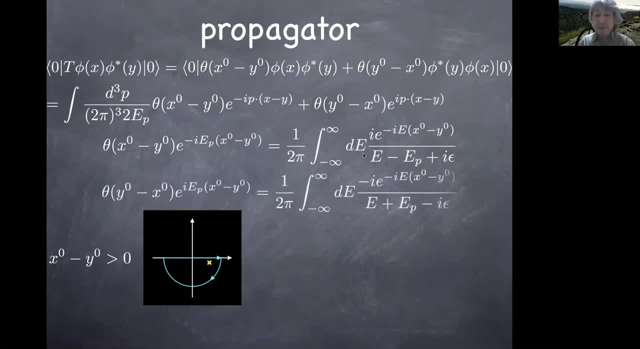 this energy integral. you do the same thing for the second piece by using a different pole, which is relevant when x naught minus y naught is negative. so again we do, because it's minus i in the exponent. when this is negative, i can add exponentially small contribution in upper half plane. 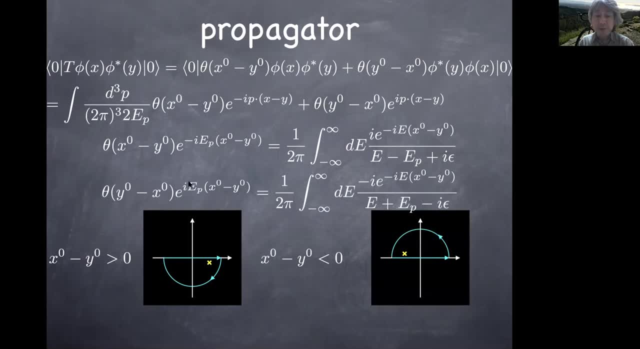 to encircle this pole and to recover this original expression in this e to the ip dot x minus i. but when x naught minus y naught is positive, i'm supposed to go down on a lower half plane that doesn't encircle this pole and i get vanishing result. hence the step function. 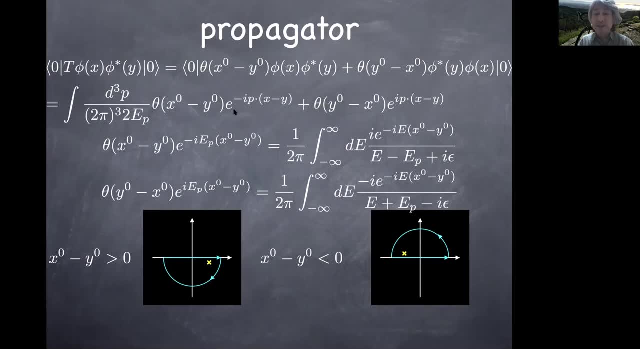 so this is the way i can rewrite two different pieces of the time ordering with a single integral in e. if you add these two pieces, and if you add these two pieces, you can see that one over e minus ep and one of e plus ep ends up being one over e minus ep squared and two e upstairs two. 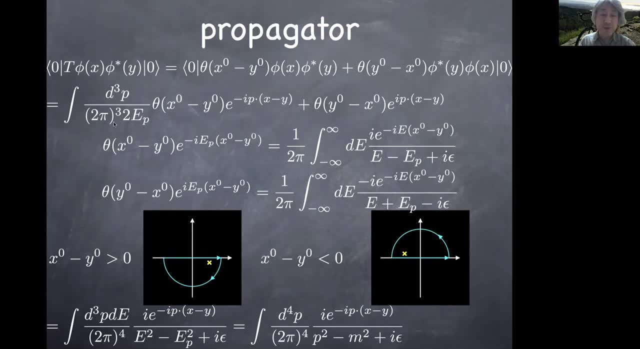 eastancel's, this 2e in the original mode expansion. so i end up with this four dimensional integral over p, three dimension over p and one dimensional over e. so this now looks very Lorentz invariant. and also this denominator e square minus e, p squared, remembering ep is negative. so i take this: 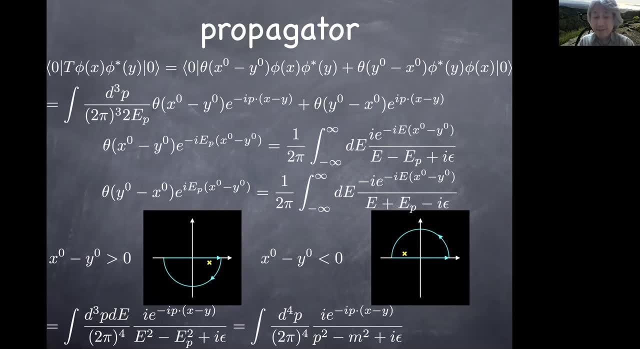 E. p is square root of p squared plus m squared. This is e squared minus p squared minus m squared. E minus p squared is the Lorentz invariant inner product p squared. So now everything looks fully Lorentz invariant. So that's the propagator. So if you take this integration volume away, 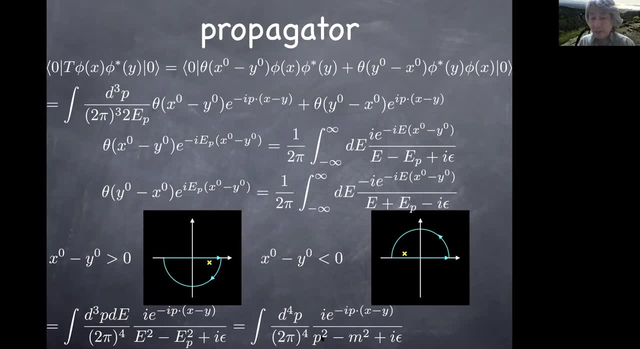 if you take this wave factor away, it's i over p, minus p squared, minus m squared together with this prescription, how to avoid the pole. So this is the propagator: i over p, minus p squared, minus m squared in the case of complex Klein-Gordon field. And this is what you're. 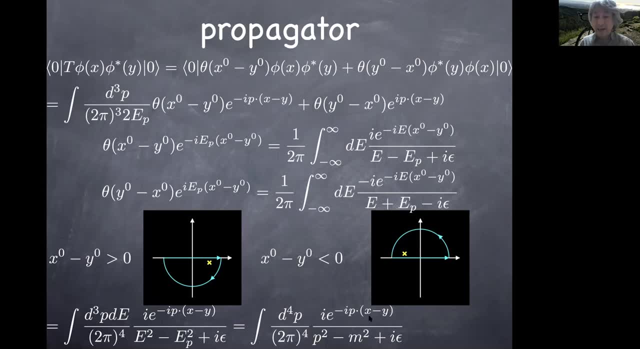 supposed to derive in the first half of the homework problem, And now I'm sort of giving it away here, but I hope you can follow this three on your own to convince yourself that this is indeed the time-order product of the field operators. Any questions about this? 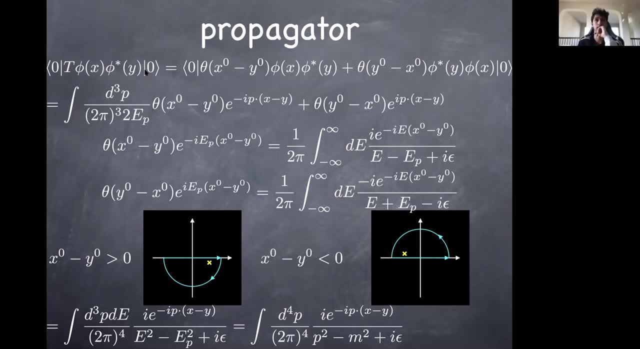 How do we arrive at the first expression on the last line from taking the sum of those two, This one here at the bottom, Yeah, So I'm just summing this piece right-hand side of the first time ordering and this piece right-hand side of the second time ordering. Both share the. 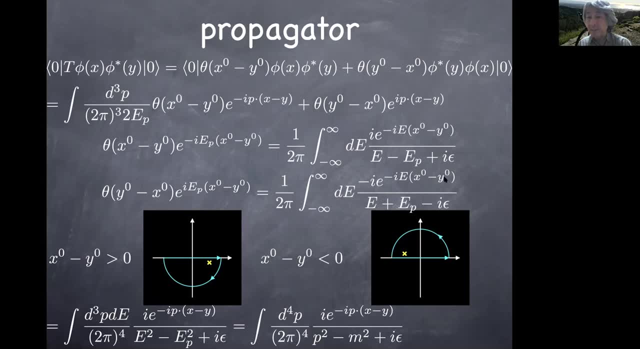 same frequency, dependence: e to the minus i e x naught minus y naught. Only difference here is: i over e minus e p And minus i over e plus e p, And you combine two fractions so the denominator becomes the product of two. 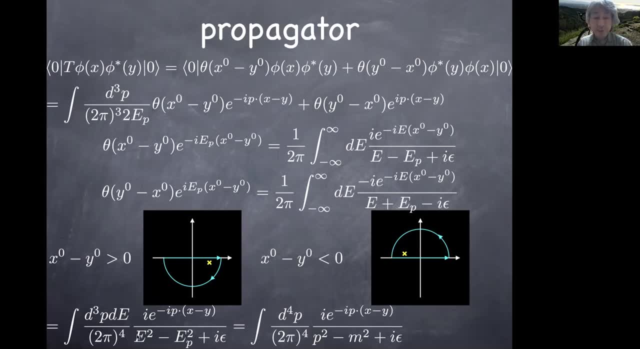 e minus e p times e plus e p. is e squared minus e p squared. Numerator is sum over the two. together with the minus sign, That turns into 2 e p. And going back to this original volume that has one over two e p in it, numerator cancels this one. 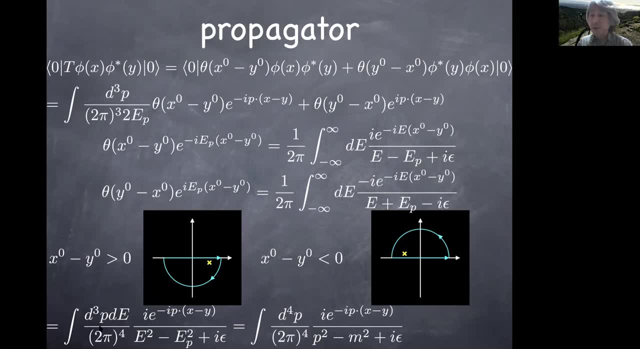 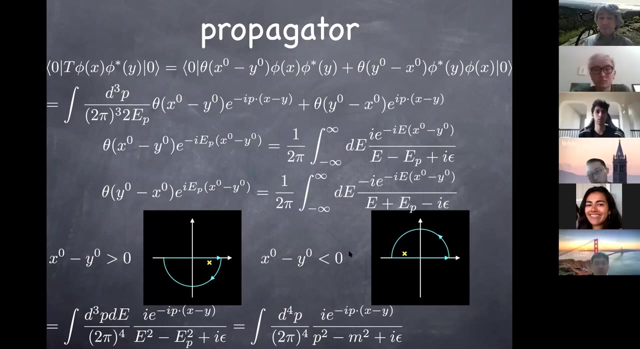 one over two EP, so that I end up with this integration body at the bottom. Do you see it? Yeah, yeah, Okay, good, Thank you for asking any other questions And, yeah, I guess. just one quick thing: Where did you get the P squared minus M squared? 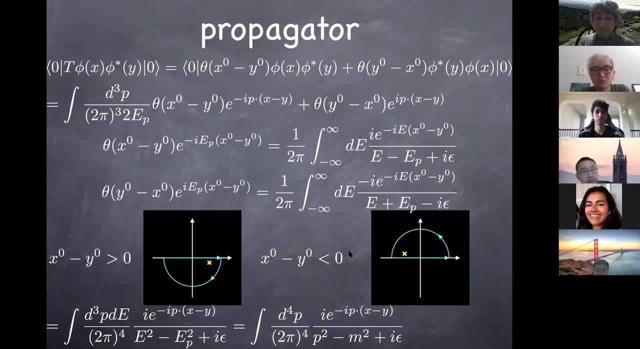 Isn't this from the dispersion relation for E? That's right. So EP is square root of P squared plus M squared. I'm setting C to one now. So EP squared is minus P squared, minus M squared where P is a spatial component of P, right. 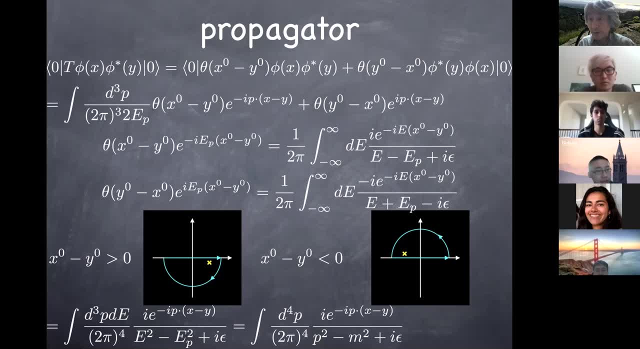 Then I have E squared, minus spatial component of P squared, which is written as the Lorentz invariant P squared, P mu, P, mu. Then I'm still left with minus M squared. So that's the meaning of this denominator Right. 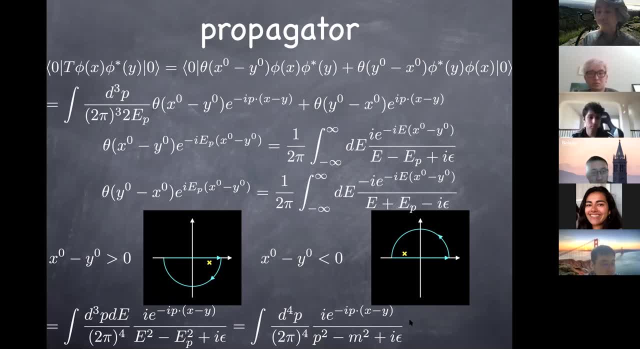 Any further questions here? Just to check: is theta the step function? Okay, thanks, Yeah, so theta is one when the argument is positive, theta is zero when the argument is negative. That's a common notation of the step function. If you haven't seen it, that's a definition. 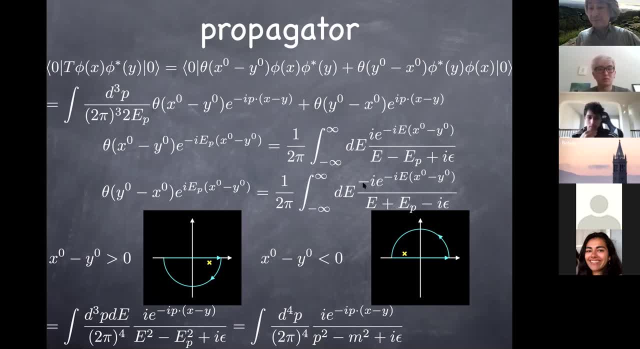 Okay, thanks for asking that too. Any other questions? So what we have done with the propagator photon is the same idea, but now you need to do that with the, with the Lorentz index, But the point here is the propagator. 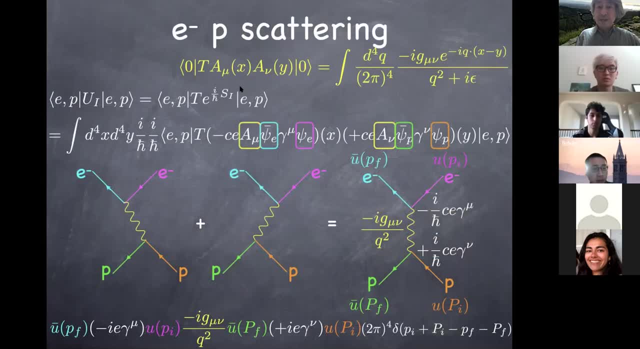 now looks fully four dimensional. So that's the idea. So in the case of the photon field, I don't go through the same kind of calculation which I did with the Klein-Gordon field, But the only difference is you end up with additional numerator, which is G mu nu. 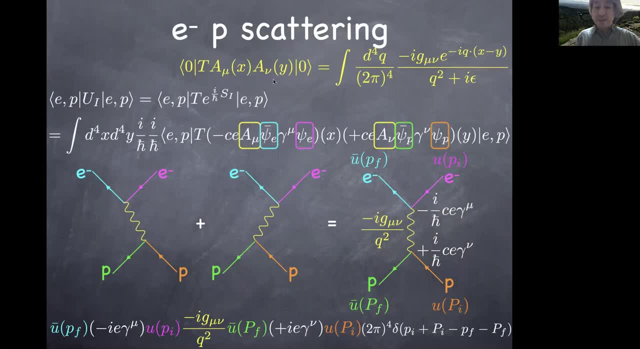 That's the only Lorentz covariant thing I can write to be consistent with these indices. And that justifies this yellow line as minus I g mu nu. And that justifies this yellow line as minus I g mu nu. And that justifies this yellow line as minus I g mu nu. 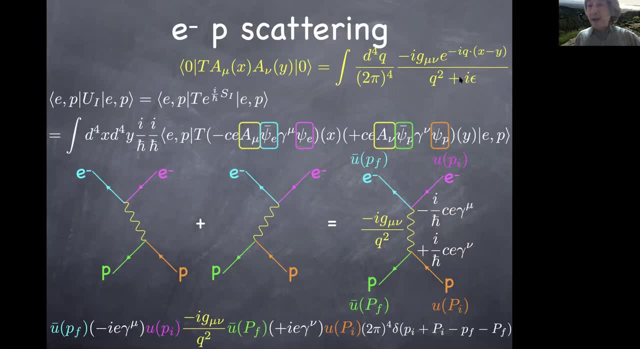 over q squared and a photon doesn't have a mass. that's why there's no minus m squared. Now I have told you how every factor in this expression came from. So from psi fields and psi bar fields, I have these positive energy solutions, u and u bar. I have this vertex e. 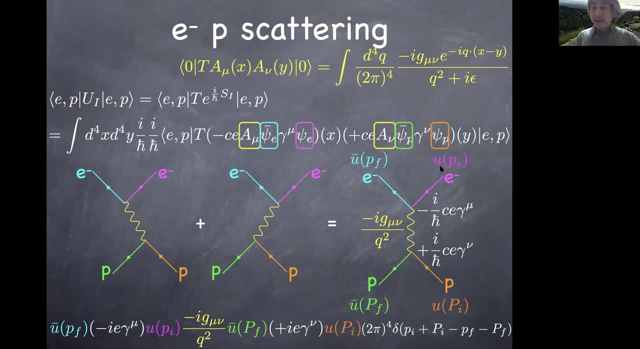 gamma nu in between, And from the electron field I have positive energy solution u and u bar. Again, this vertex e, gamma nu is in between, And then they're connected by this yellow line, which already sums over two possible time orderings on the left into a single. 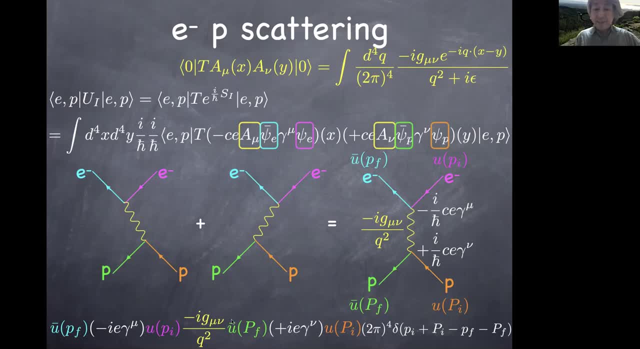 wavy line And that's this minus ig, mu over q squared. So once you draw this diagram, you can associate each line with factors, each vertices with factors, which you just multiply along the direction of the arrow, And you don't need to go through. 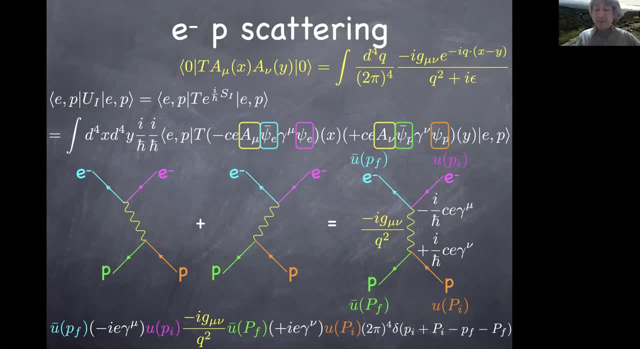 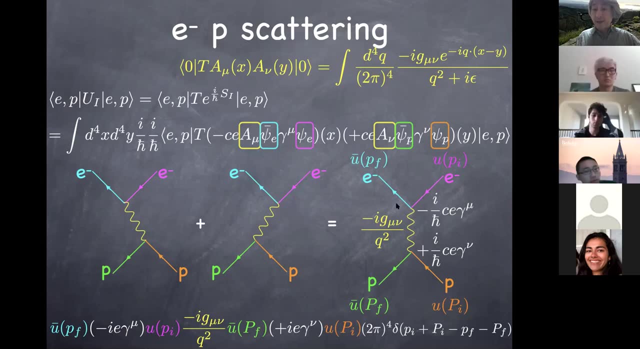 this process ever again, which you can immediately write down: this amplitude together with a delta function, which I didn't write earlier. So that's the idea of the Feynman diagram. Any questions about this? Okay, so give me just a few more seconds minutes. 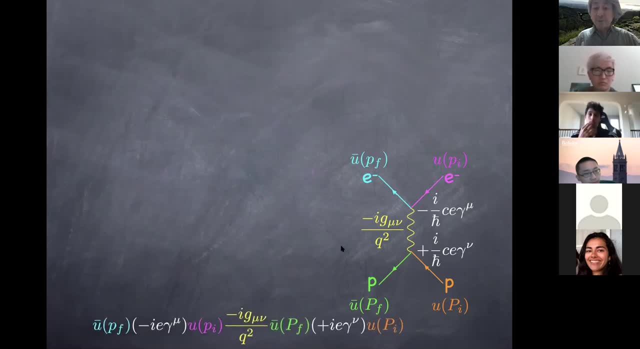 to give you this entire picture of the Feynman rules. So when you have initial state particle, you associate that with positive energy solution. Final state particle is associated by u bar, as we have done with electron and proton in electron proton scattering process. 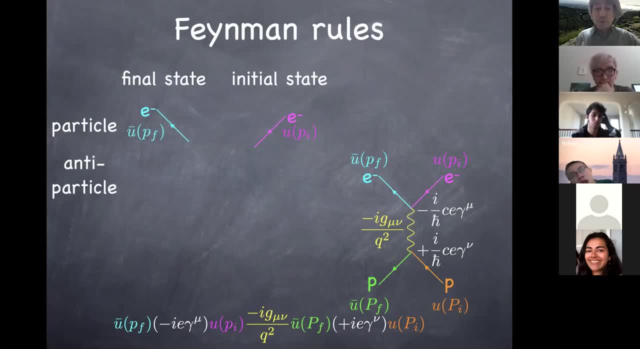 If you have anti-particle, though, the arrows go backwards, So initial state would have arrow going backwards and that's why you associated with bar of negative energy solution And final state antiparticle will be just negative energy solution without bar. 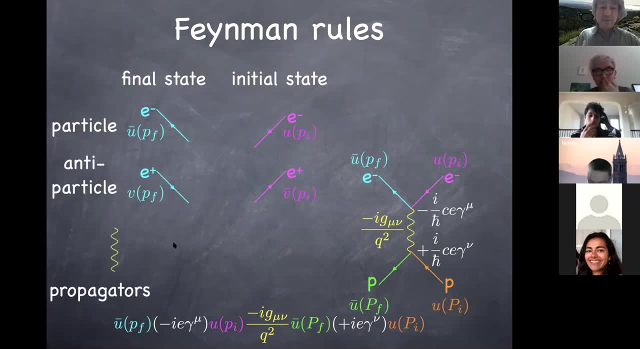 And in the case of the propagator, you have this wavy line I associated with this factor over here And the vertex we have already derived is minus I, E, gamma, mu when you set C and H bar. to be one. So the only thing that are missing so far, 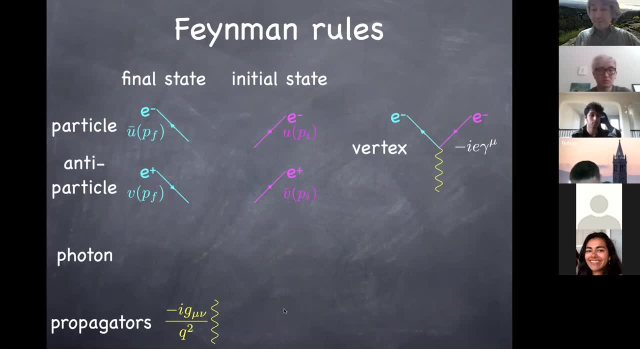 is the photon initial and final state, And when you have photon initial state you associate with a polarization vector. We also worked this out before when we quantized the Maxwell field And final state. photon is also associated with the polarization vector, but with complex conjugate. 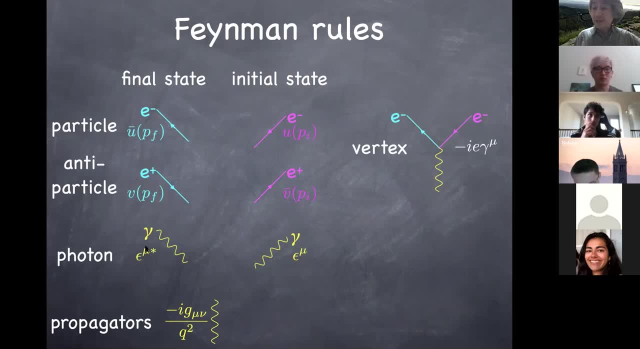 similar to bar in the case of fermion. if you use helicity eigenvector in states, which is the complex polarization vector, You also need to know the propagator for the fermion And that actually has this form, which is also very simple. 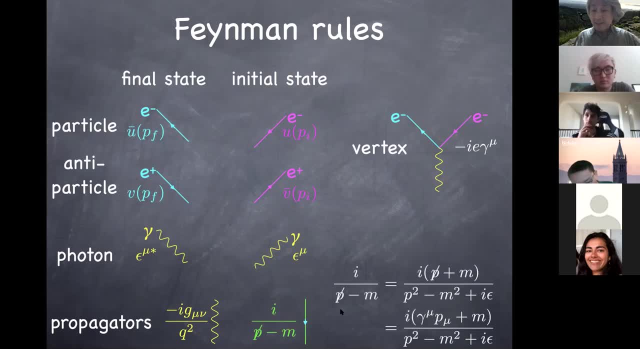 And you have this new notation, P slash, and P slash is meant to be gamma mu, P mu, which is a matrix. Having matrix downstairs sounds weird but it's defined to be by multiplying P slash plus M in both numerator and denominator. And if you multiply P slash plus M to P slash minus M, 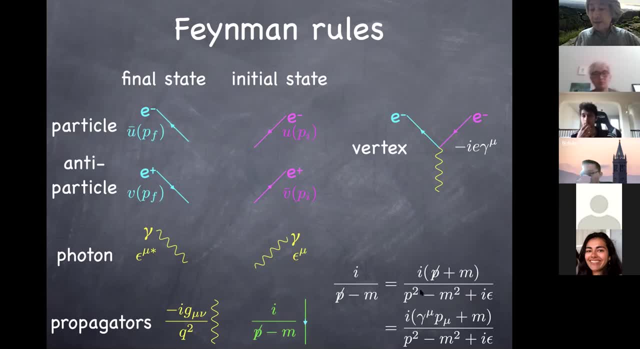 you get P slash squared minus M squared. P slash squares using the anti commutation formula for gamma mu turns into just a number of P, mu, P squared. So you don't have any matrix downstairs anymore. the only matrix is now in the numerator. 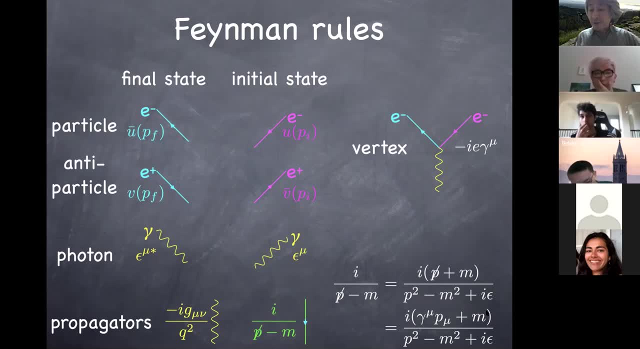 So that's just a shorthand notation of this combination out here And that's the propagator you use for the fermion. Then you know everything's under control. so that's good thing you need to know in order to work out the Feynman amplitudes The minute you draw a diagram. 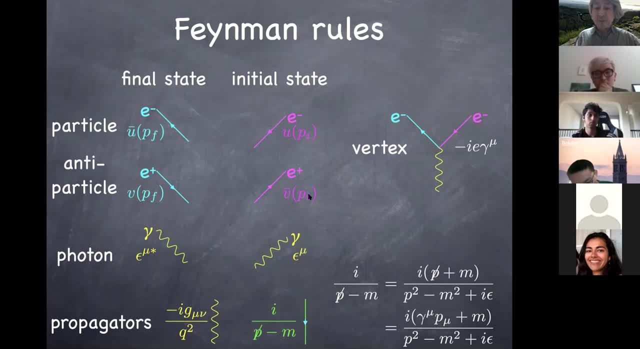 you can associate every initial state and final states with these in some sense wave functions, every internal lines with these propagators to write down the Feynman amplitude. And so here's one example of that, If you're talking about the process of electron positron, 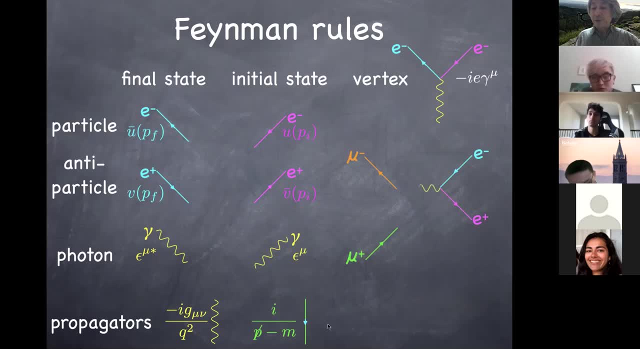 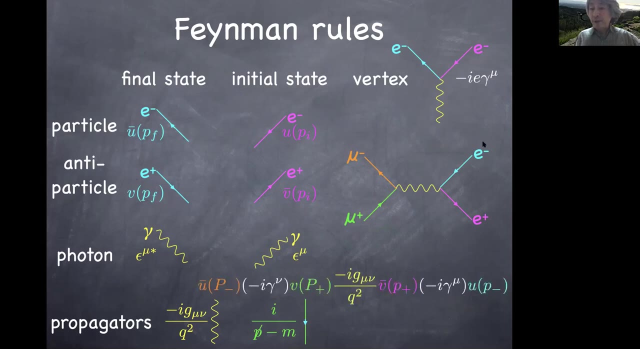 going to muon muon. you glue them together to a vertex. I associate this propagator for the virtual proton. Here's yet another vertex And the minute you have this Feynman diagram, I can immediately write the Feynman amplitude associating this electron initial state with the positive energy. 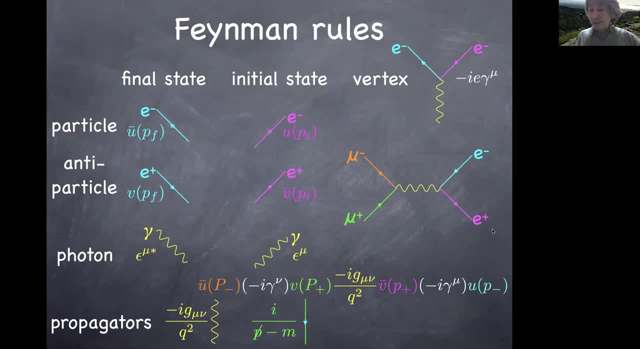 solution positron in the initial state as the negative energy solution with bar. according to this rule, You have propagator for the proton and final state antiparticle. is this negative energy solution? here is the vertex And final state particle is positive energy solution: bar. 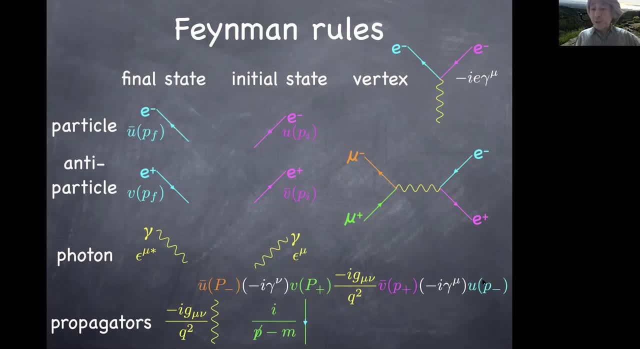 So this Wasser Sag instantly corresponds to this specific expression where you can plug in the solutions to get a number out. That's the way you use this Feynman rules. Whenever you think of a process, the first thing is to use this vertex to glue them together into a diagram with a consistent flow of the arrows The minute. 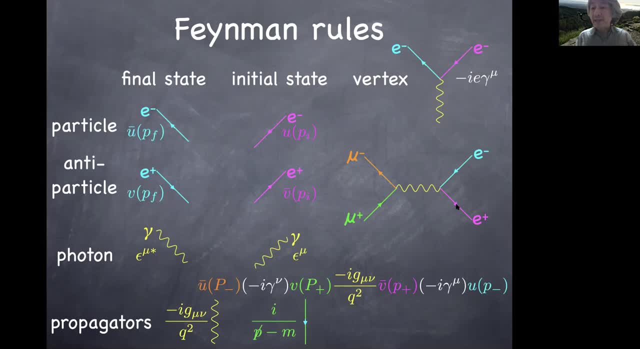 you have a diagram, you know how to associate each lines by these factors, to immediately write down the amplitude for the process, together with the four-dimensional delta function. So that's when everything becomes very visual, intuitive, but very practical, because the diagram means something very specific in terms of writing down the amplitude. 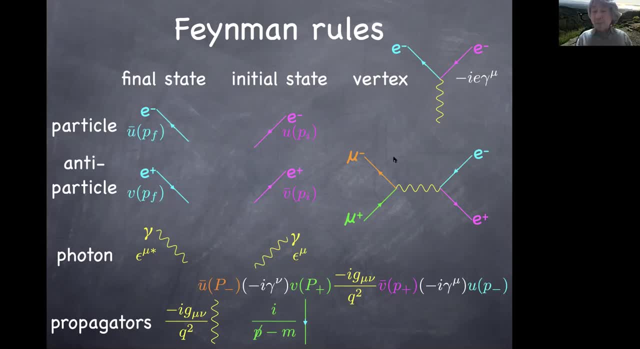 And we go through this once again on Friday. and once you have this amplitude, of course you can compute the cross section and we go through some simple examples and working them out and that basically completes the course on quantum field theory this semester. Okay, any questions here? So at the end I went fast just to get flash the idea and go through. 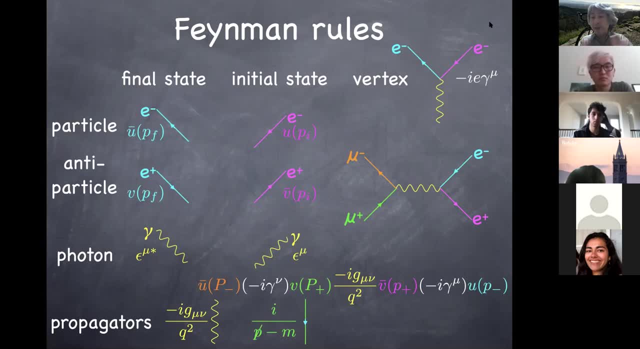 this once again on Friday. I hope you see where things are heading and end result is very intuitive, visual and practical. That's the idea of the Feynman diagrams. Any questions? I just had a question about the propagators. So are they essential actors that you can't hear you? 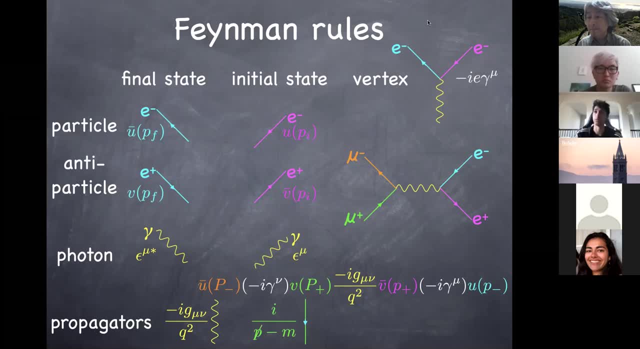 somehow. Oh, can you hear me now? or I still can't hear you for some reason. Maybe that's my problem, I'm not hearing it. I can hear something just now, but not right now. Well, I'm hearing it. Are you speaking, Tom? 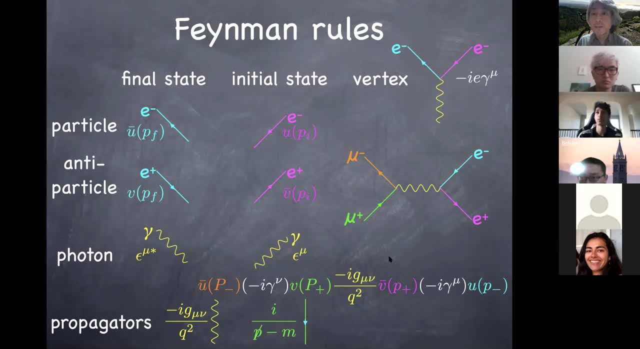 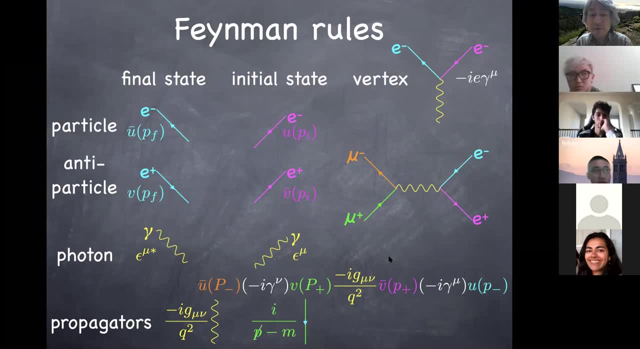 Let me then switch the computer microphone. Hello, can you hear me? Can anybody speak? Oh, hello, Yeah, I can hear you now. Sorry, that's my problem, it seems. Yeah, I just had a quick question on the propagators. So are they essentially just the factors you get from the intermediate state, the vacuum states? 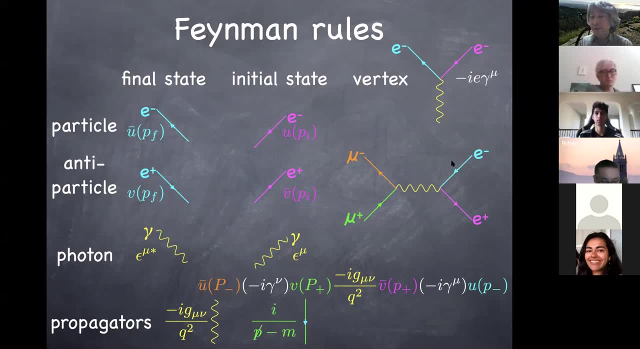 That's right. So I don't have any photon initial state. It is created at this point. It is created at this vertex. It's annihilated at this vertex. That's why it corresponds to this expression of the propagator starting with a vacuum. 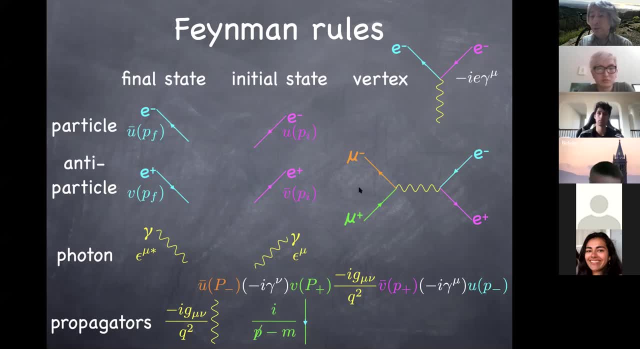 I have a new field, a new field with time ordering going back to vacuum, And that's the propagator. Oh, I see, But we don't have propagators like for the products. you know the resulting particles on one side and the particles that were the original particles, because we're annihilating those and creating them. 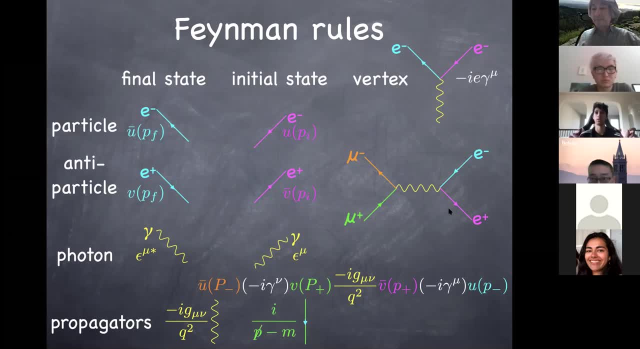 So they have their associated factors. So the propagator is just when you go from vacuum state to vacuum state and you get some non-trivial factor from that process, Right. So you use propagator when a line starts with a vertex and line ends with a vertex, which is the internal line in a diagram. 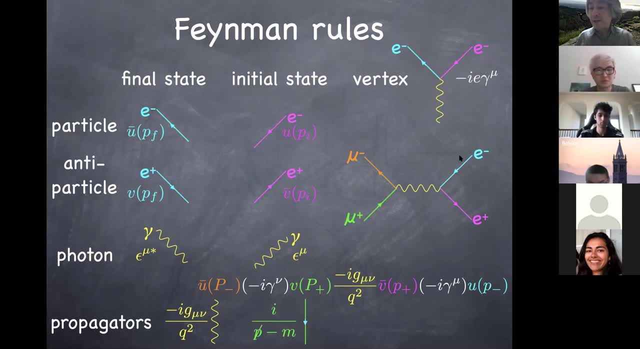 Here electron and muon are external lines because they correspond to the particles that exist in the initial ket and particles that exist in the final bra. So external lines are not propagators. They come with this: positive energy solutions or polarization vectors. Internal lines are given by propagators. 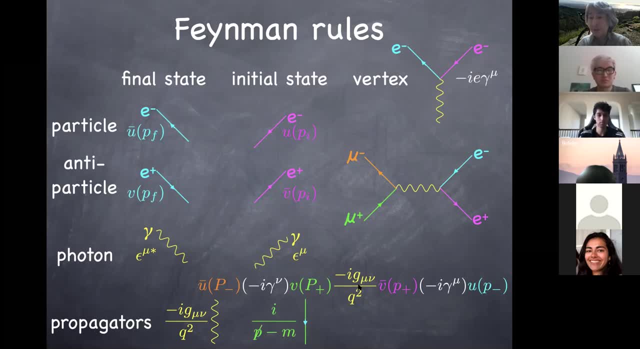 And that's the idea. Thank you for asking. That's a very good clarifying question. And, Tom, you had a question too, Now that I can hear people. No, I was saying I can hear you, So that was my problem. 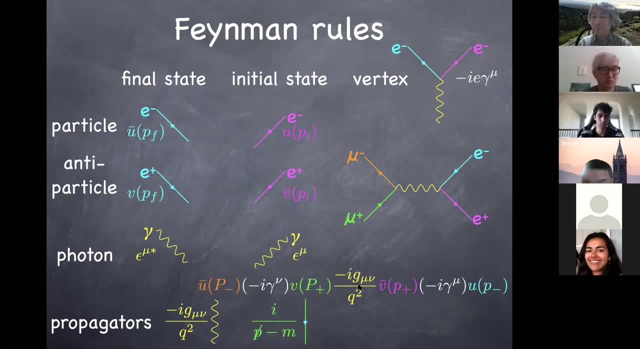 Any other questions here? No, Okay, So we'll come back and talk about this again on Friday, And once you start seeing many examples, I believe that idea would start to sink in, So you can understand what diagrams mean And you learn how to associate amplitude for whatever diagram you see. 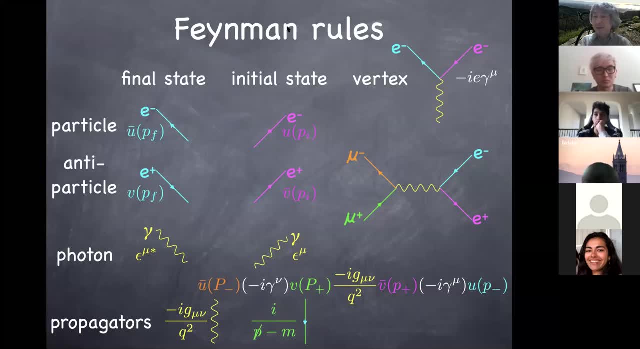 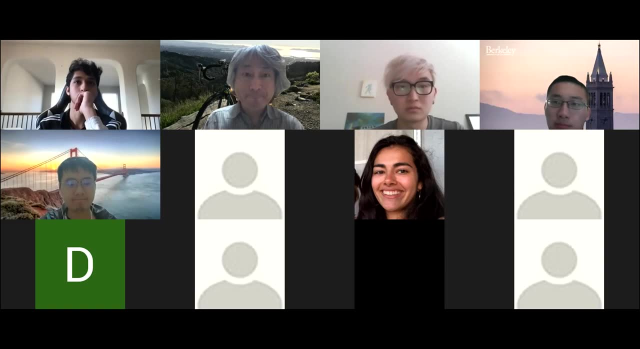 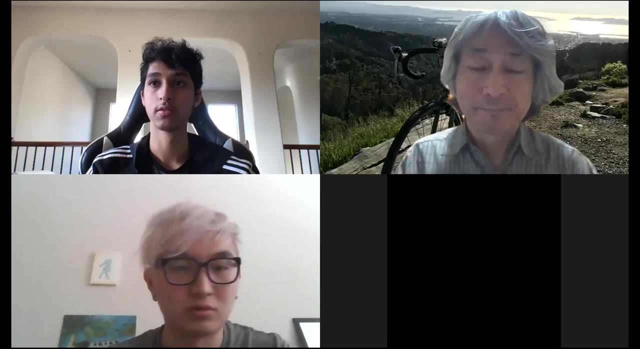 So that's what we do on Friday, Okay, So I see you again on Friday, And then we are getting close to the end of the course. Okay, So stay safe, Thank you. Thank you, Bye.